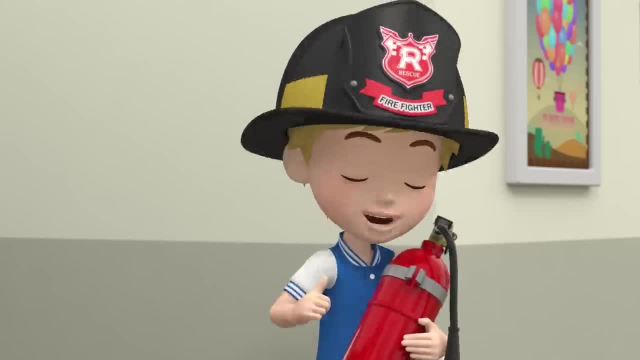 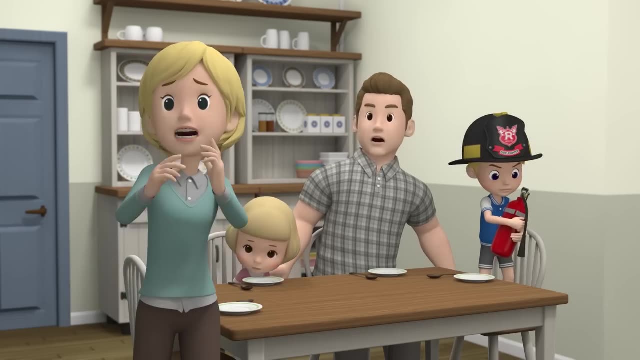 No, you won't, Mom. The safety of our house is in the hands of the fireman. He's right, Let him be the fire expert. Hmm, Huh, Oh, my Fire Fire, Oh, no Huh. 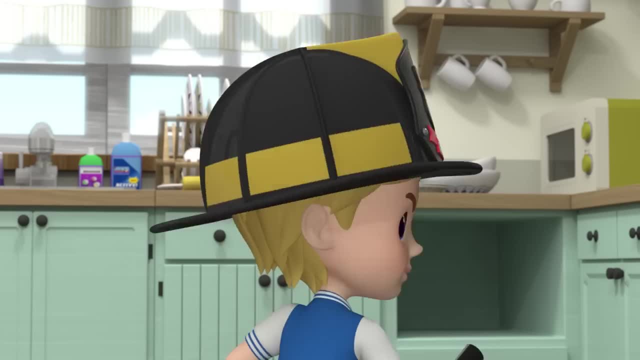 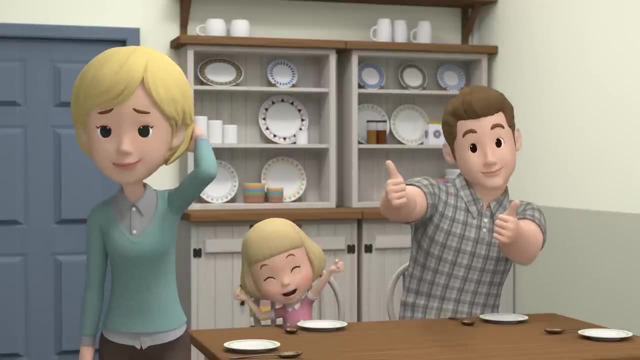 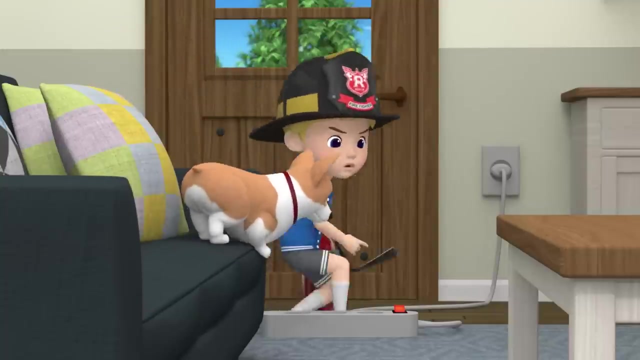 Ha, Oh, Everyone's safe. Am I a real firefighter or what? Wow, Hey Peter, that was really awesome. My brother's the best. Ha-ha-ha-ha, Hmm, Hmm, Whoa, Easy, buddy, Keep back, It's dangerous. 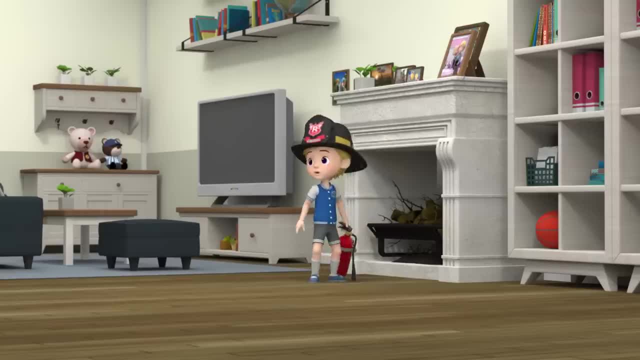 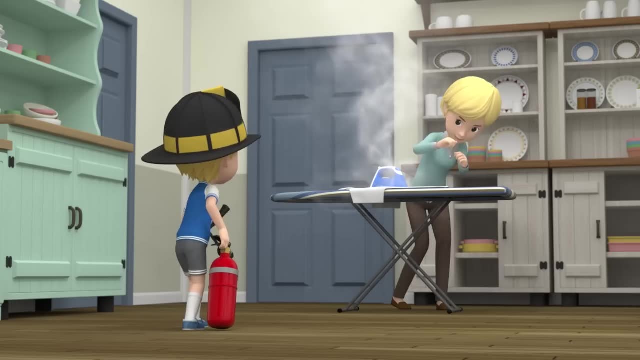 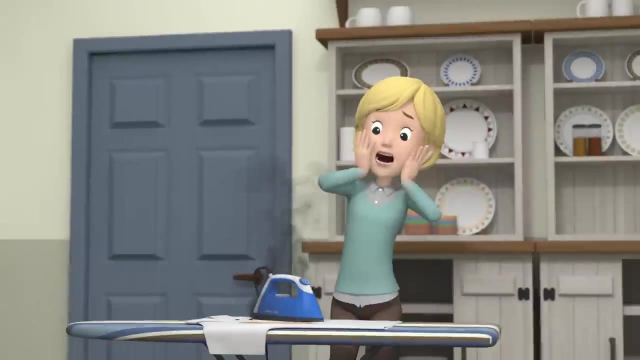 Hmm, Looks safe. Huh, Hmm, Is that? Oh Ha, Huh, Ah, Huh, Peter. Oh man, I thought it was a fire. Goodness, I was scared. Huh Ah, My clothes are burning. 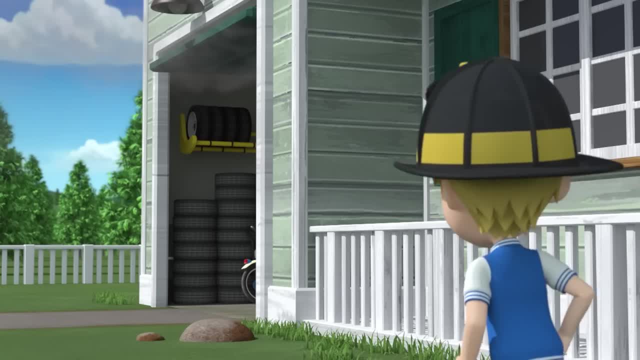 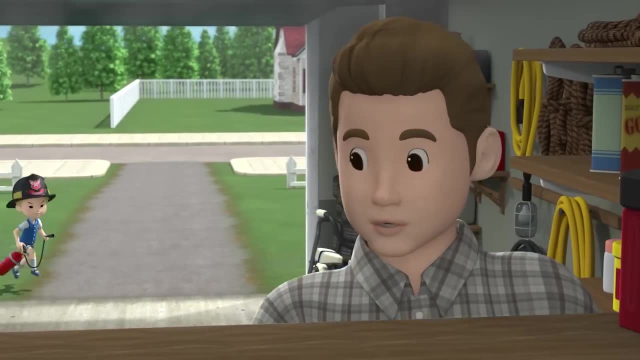 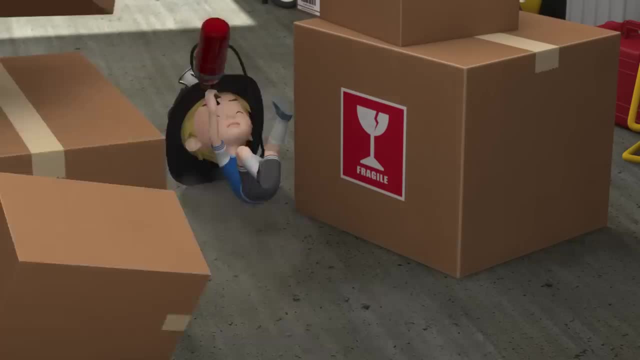 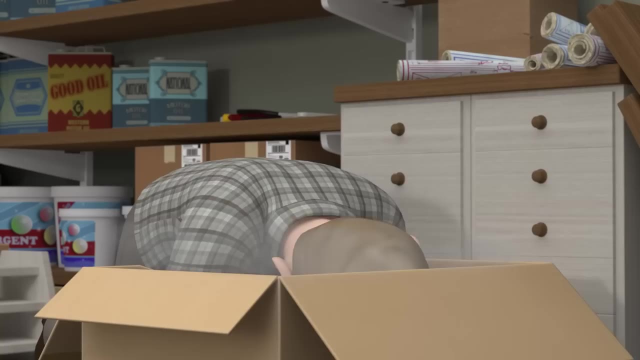 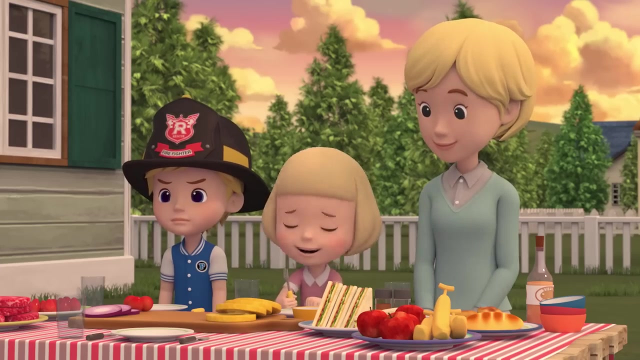 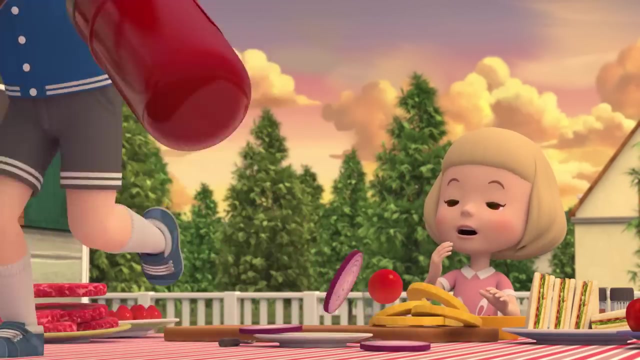 Huh, Huh, Huh, Huh, Huh, Peter, there's no fire. Smells really really good, Honey. is it ready? yet We're almost there. Huh, A fire, A fire. That was close. 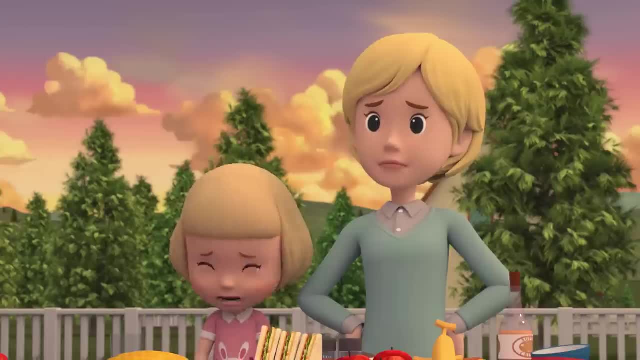 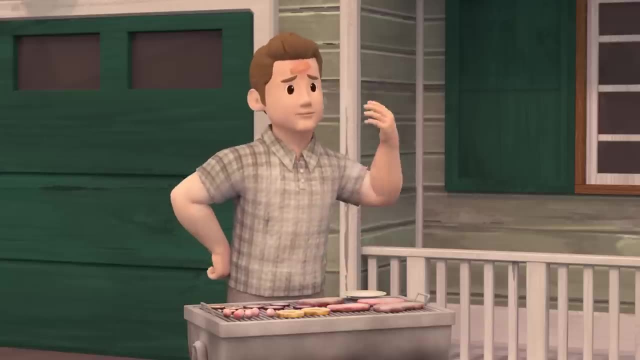 Peter, what was that? I extinguished a fire. Peter, messed up the whole barbecue. Peter, this wasn't a dangerous fire, A little grease just dropped on the charcoal. Yeah, it happens all the time when you're cooking on a grill. 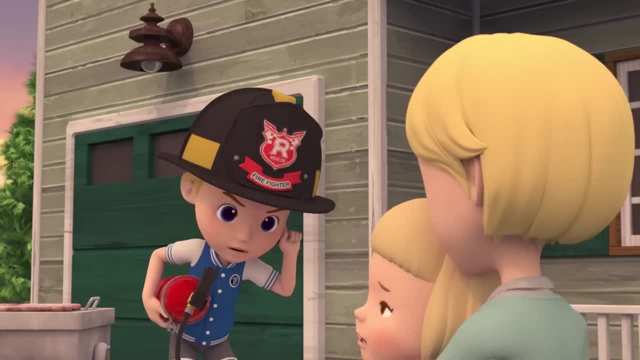 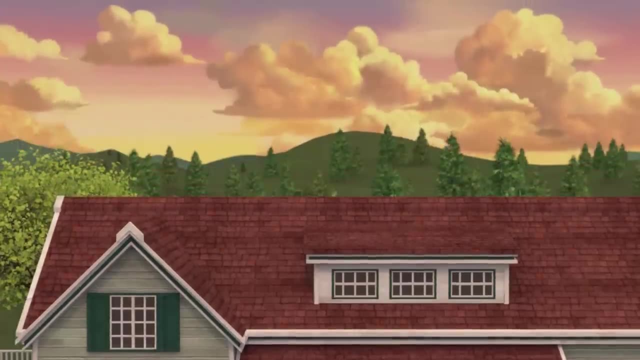 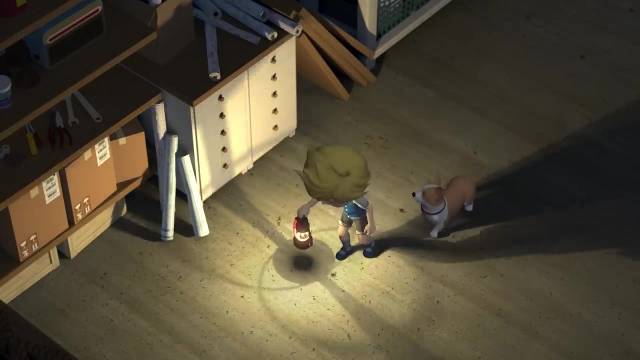 Mom, that is just the kind of unsafe thinking that leads to really dangerous fires. And that is the final straw. I'm taking this, Peter, But Dad no, Huh. Hmm, It's gotta be here somewhere. Oh, Found it. 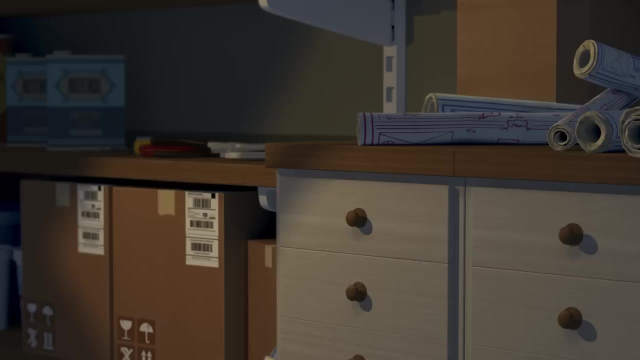 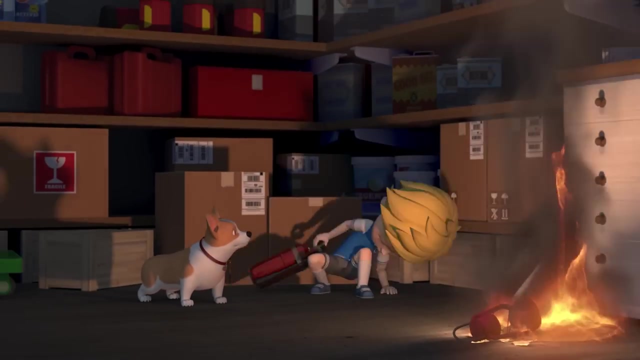 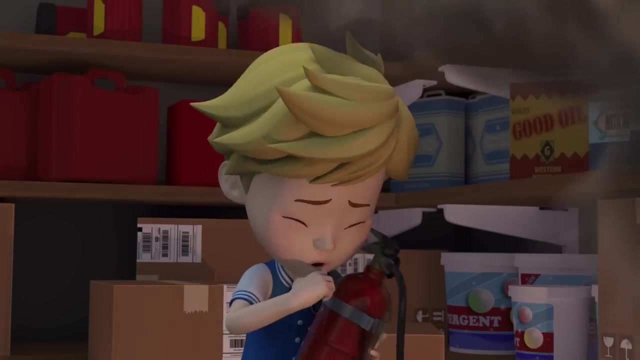 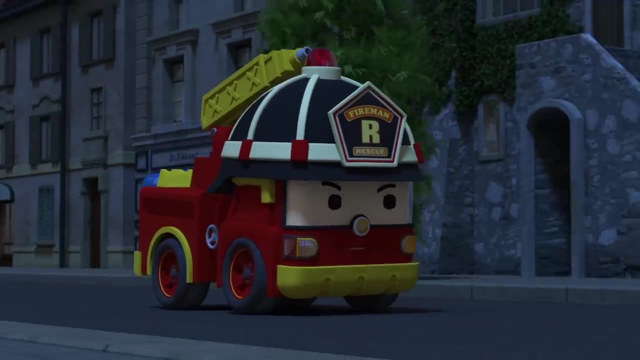 Ha, ha, Ouch. What is it, buddy, Huh, Huh, Ah, Fire Ugh. Why isn't anything happening, Buddy? what is it? Ah? Dad, Peter, Huh, What's up Jin? 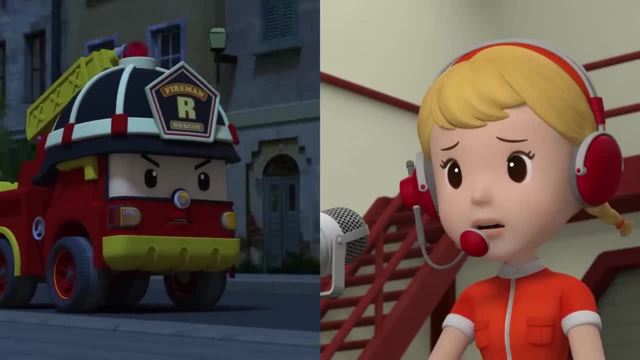 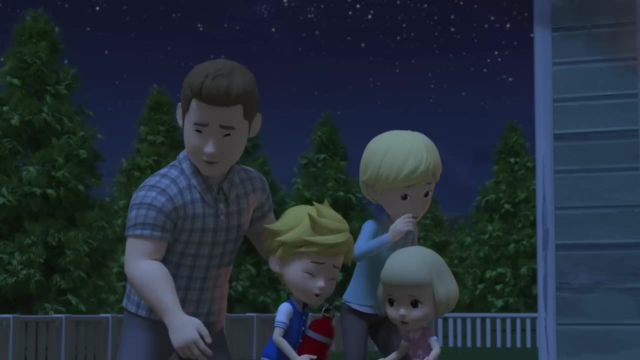 Roy, get to Peter's house quick as you can. There's a fire in his garage. On it, Hm, Hm, Ha, ha, ha, ha ha. Roy, Roy, Ha, Hmph, Hmph, Hmph. Has anyone hurt? 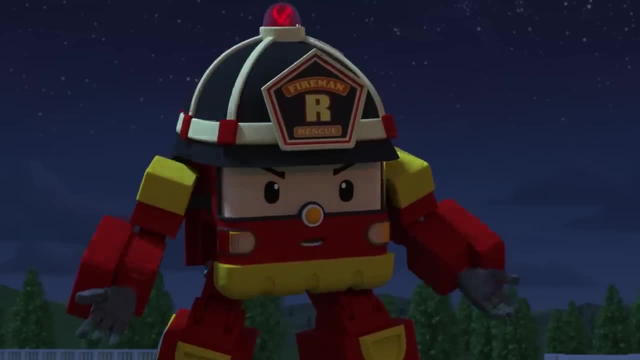 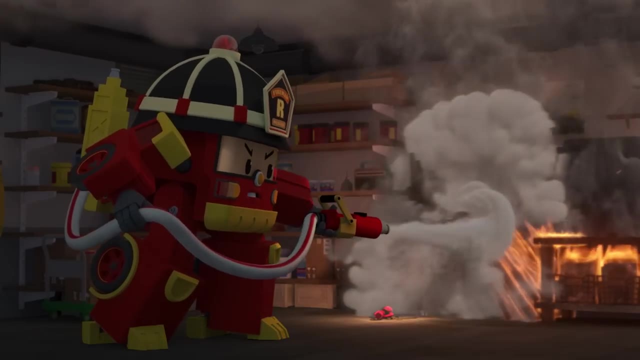 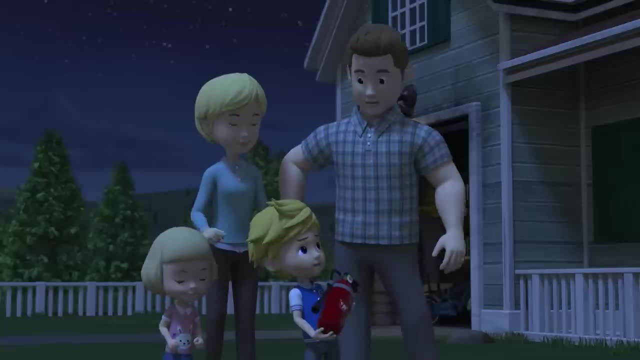 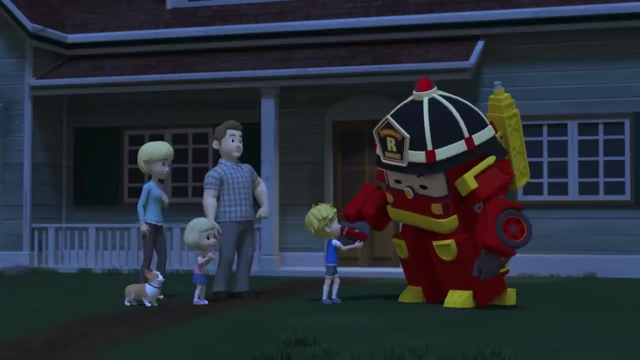 Thank you, Roy. That fire could have burned our house down. Sorry everyone, But the extinguisher wouldn't work at all, Peter, can I see that extinguisher? Of course, Roy Hmph. Tell me, Peter, Have you been using this? 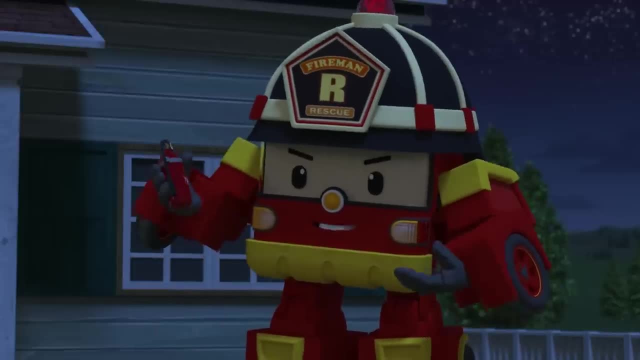 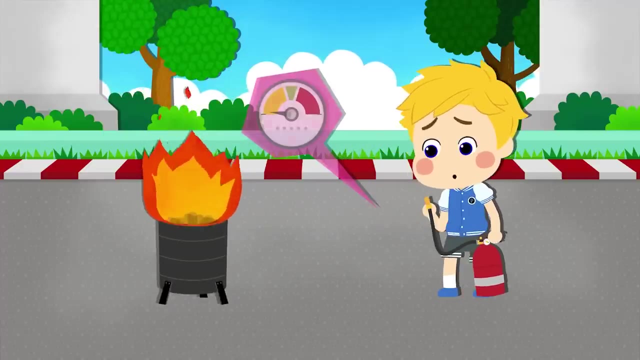 Mm-hm. I kept thinking there was a fire, Peter. fire extinguishers can't be used multiple times. Mm-hm, it loses its gas and the pressure drops. Then nothing will come out. You have to check your extinguishers regularly. 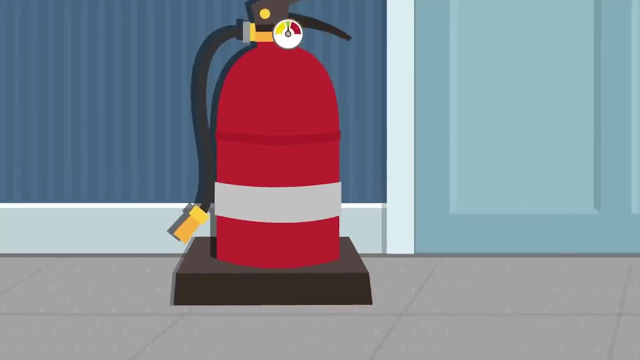 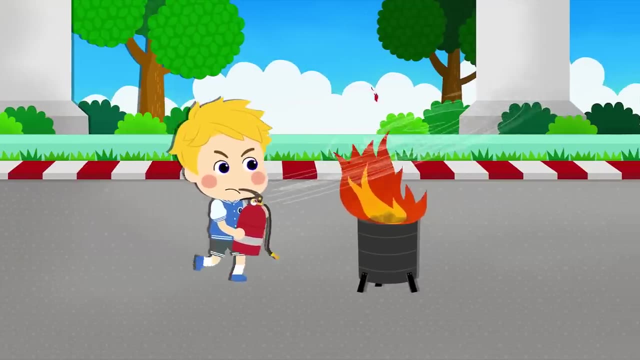 to see if they have enough pressure. It's best to put extinguishers near the exit so they're easy to find. To use the fire extinguisher, pull out the safety pin, stand against the wind and point the hose toward the fire. 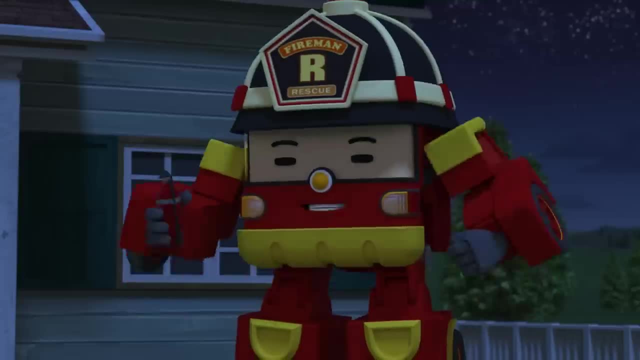 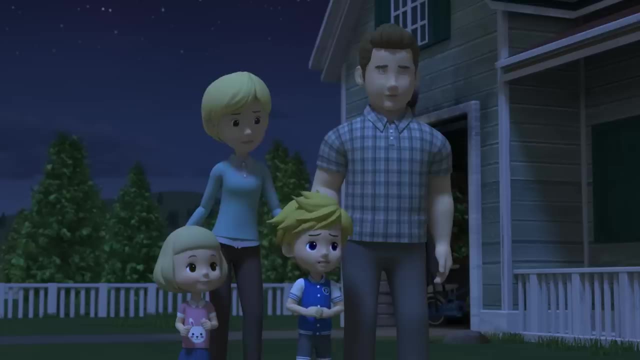 Then squeeze the handle and put the fire out. Peter, it was brave to try and use the extinguisher on that fire, but evacuate is what you really should do. You're right, Roy. Cheer up, Peter. You were only trying to keep the family safe. 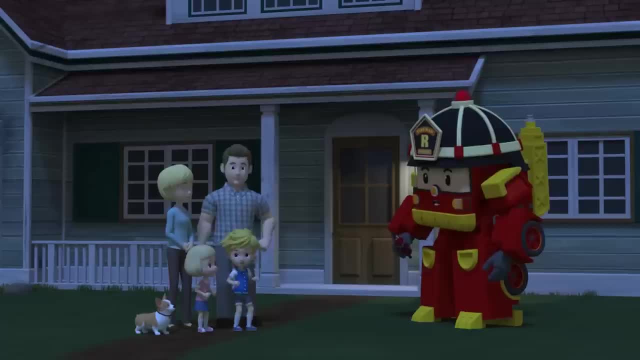 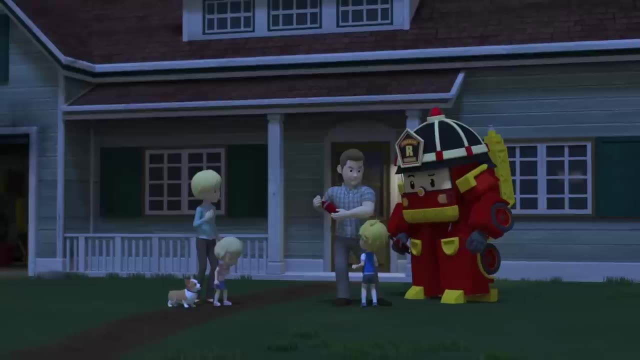 Yeah, that's true. Right Now, trade me your old extinguisher for this fresh one. Sweet New extinguisher. Oh, and it's gonna stay new, Peter, I promise I won't mess it up this time. Just let me hold it. 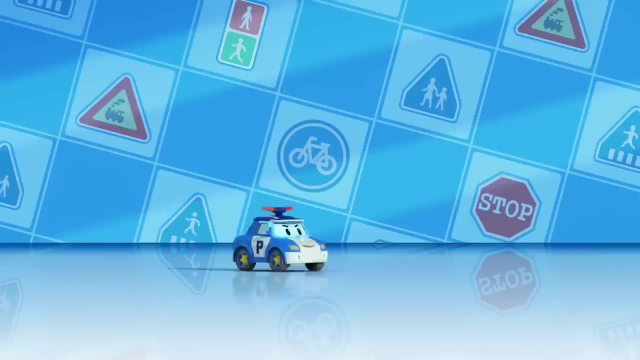 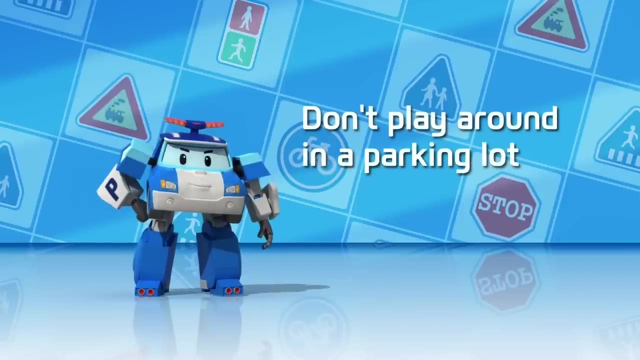 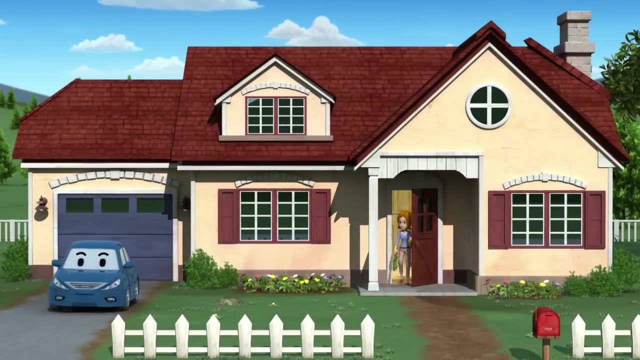 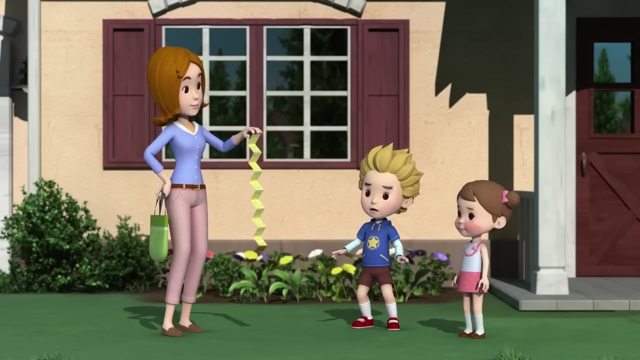 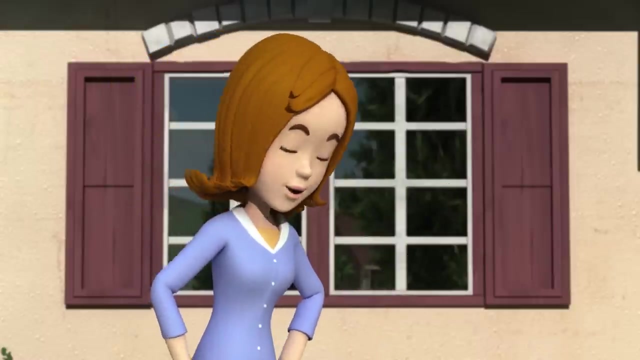 You got a chance. Yeah, Ta-da, Whoa, hey, what is that? This is a list of everything we need to buy today. Really, All that, All that. Broom Smart's having a sale right now. We'd better hurry before they're sold out of everything we need. 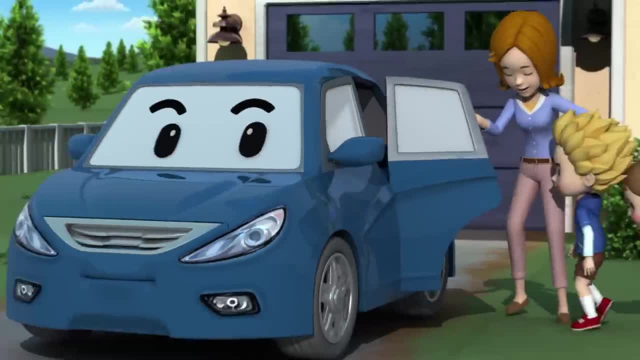 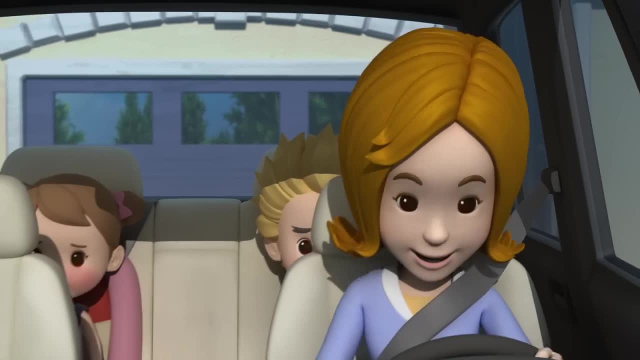 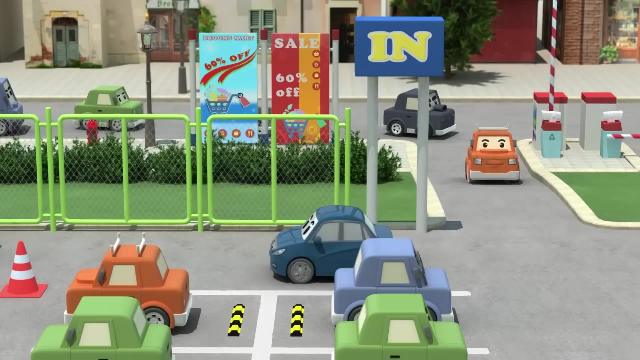 Can I get a video game? I want a new teddy bear. You guys, I'm afraid those things aren't on the list. OK, Buckle up you two, Here we go, OK, Yeah, Oh, all of these cars. 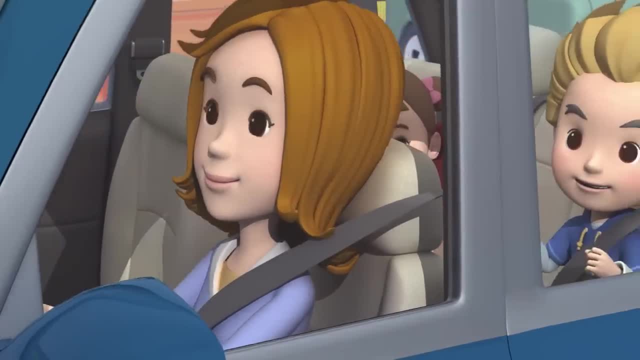 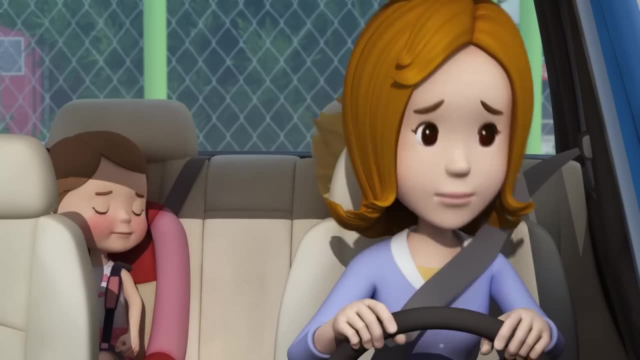 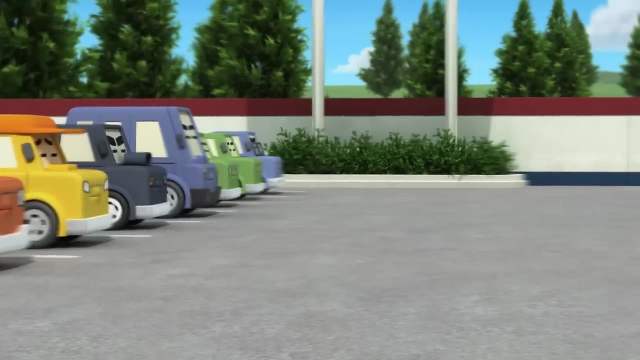 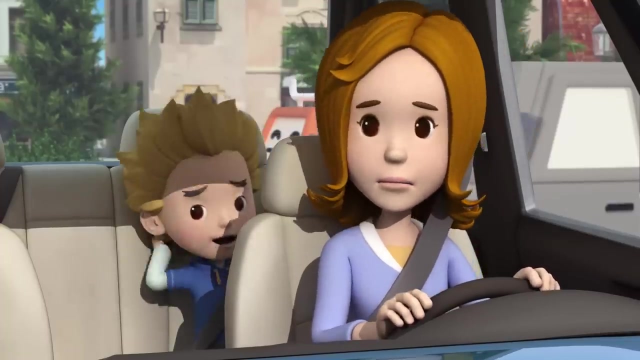 Over there. Mom look: Huh, Yes, Goodness, Are you all right? Yeah, Oh, my, We're too late. Mom, look, There's one. Where is it? Ah, Oh, there's already a car there. 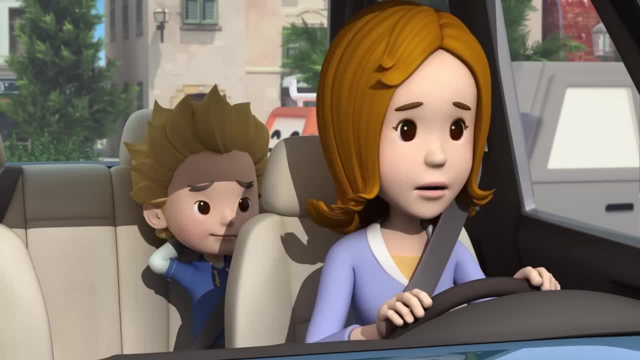 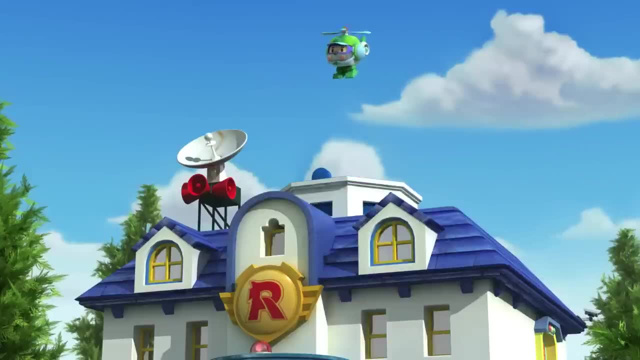 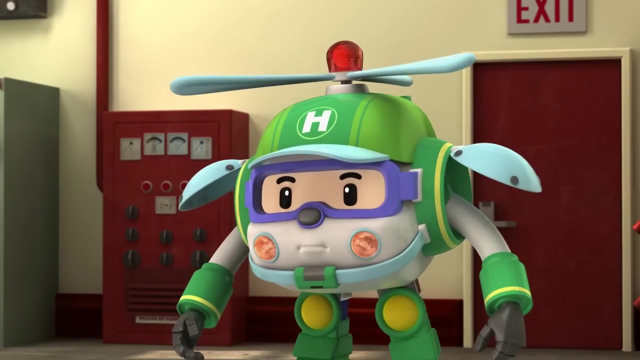 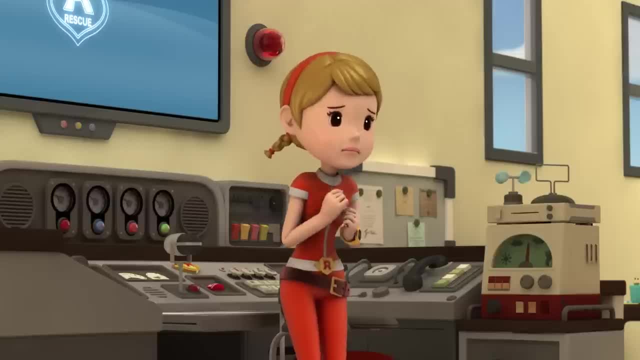 Actually, Broom Smart is having a sale and all of them are sold out. Actually, Broom Smart is having a sale and all of them are sold out. I was going to get a new bathing suit, but what if they're all sold out? 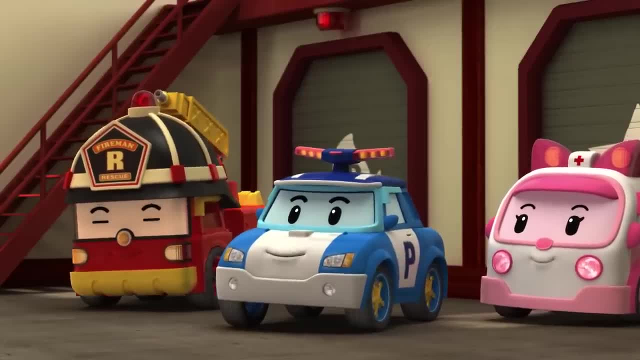 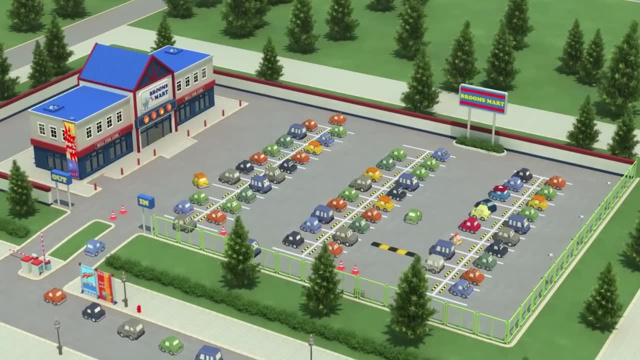 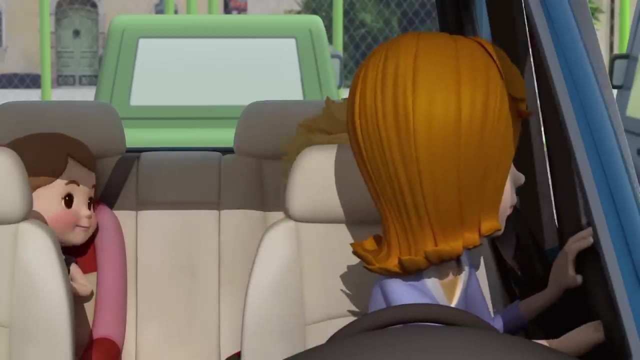 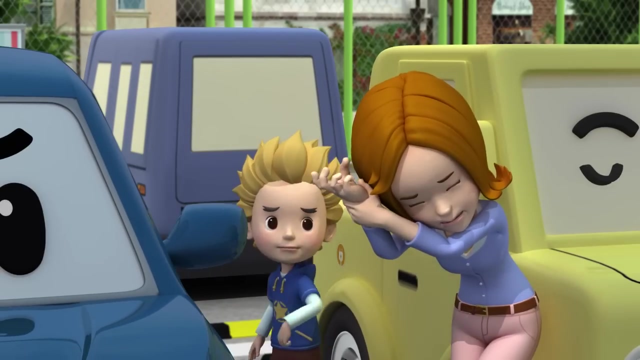 Jin, don't you think we should worry about the traffic problem first? Heli, let's move out, Okay, Okay, Now just wait for me to get the door. Huh, Watch out, Ow, You should be more careful, Mom. 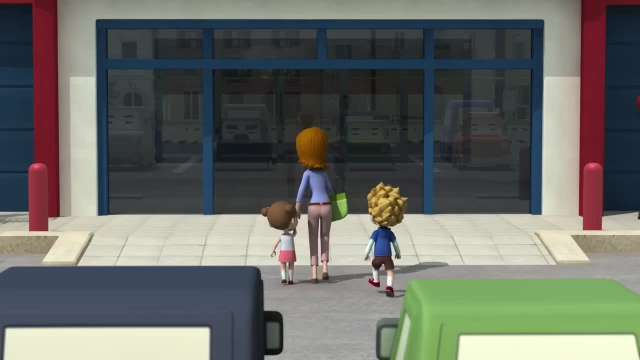 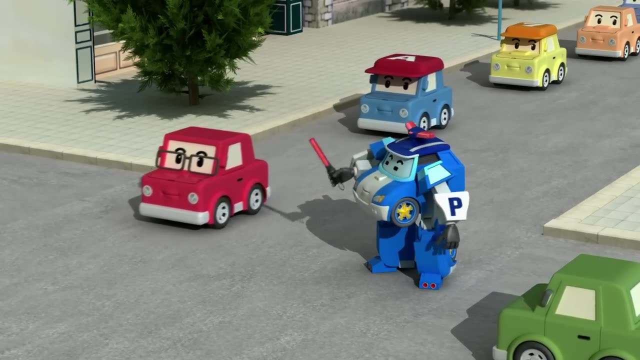 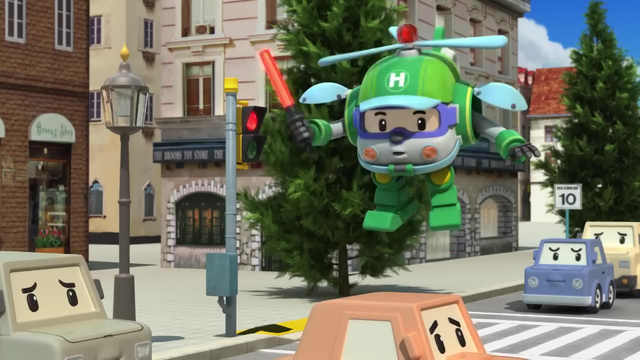 I told you to wait, Are you okay, Mommy? Yes, I'm okay. Stop, Okay, please go now. Whew, I think it's under control now, Heli, how does it look over there? Well, I've still got a lot of cars headed to the store. 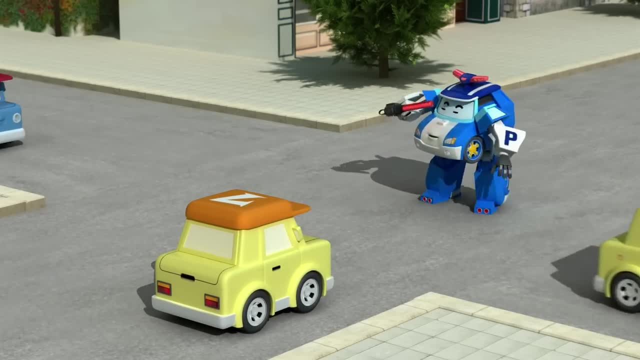 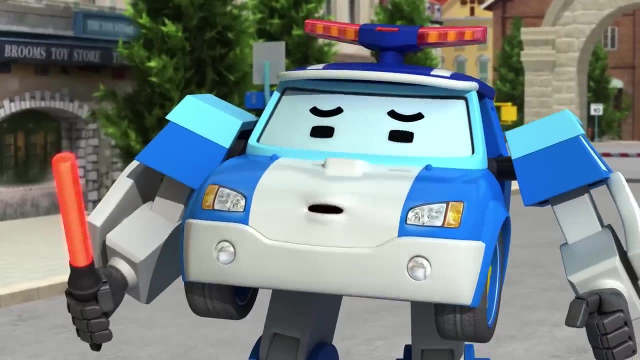 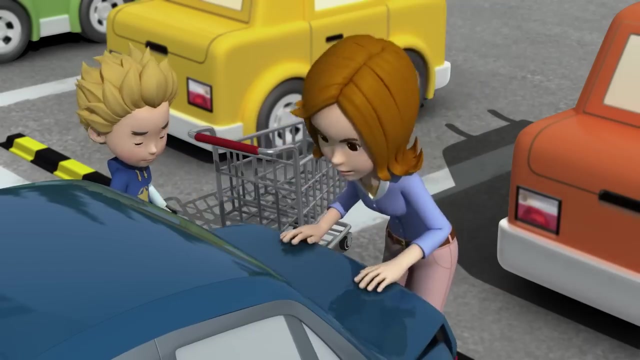 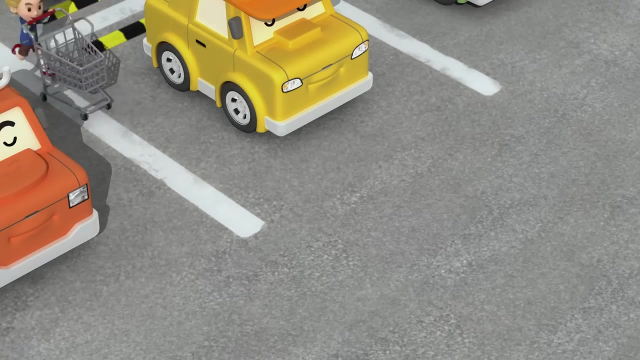 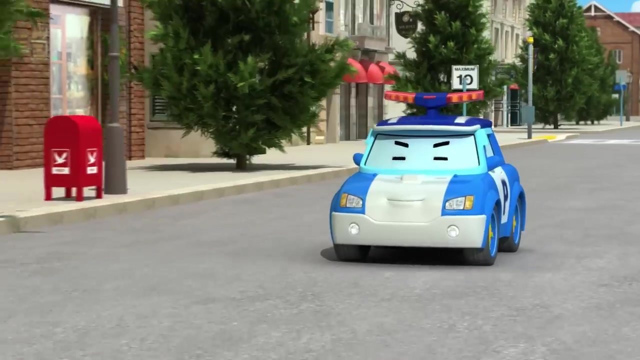 Really. Okay, I'm coming to help. Okay, So late, I'm so late. What's going on? That car is not driving safely. Hey Mom, I'll go put this back. Woo-hoo, Huh, There's that car. 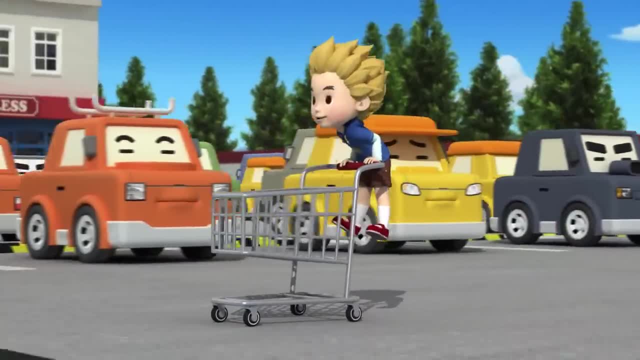 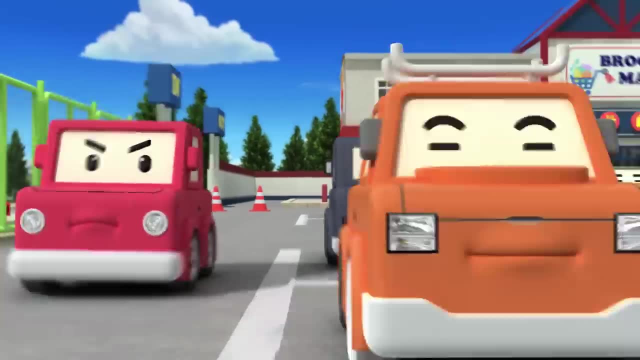 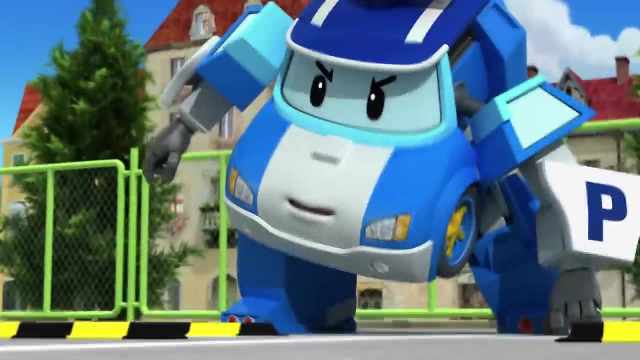 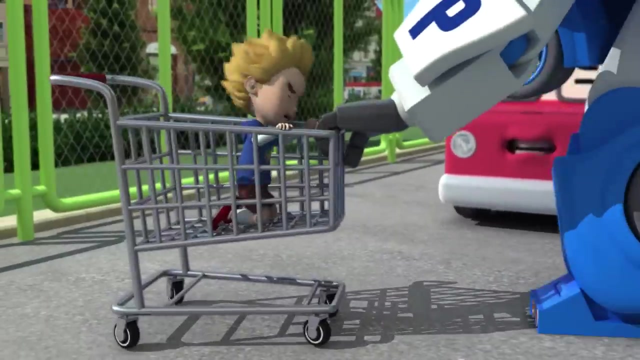 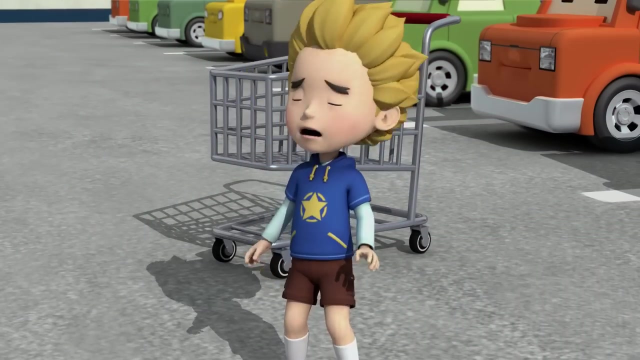 Oh yeah, Full speed ahead, Awesome. Ah, Oh, there's nowhere to park Kevin, Watch out, No, stop Kevin, Oh, Kevin, Kevin, Huh, Huh, Huh, Oh man Oh. 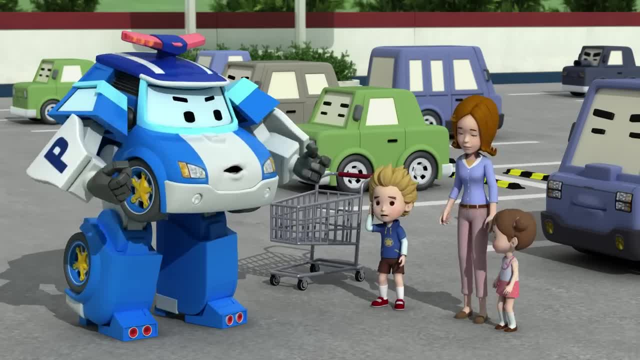 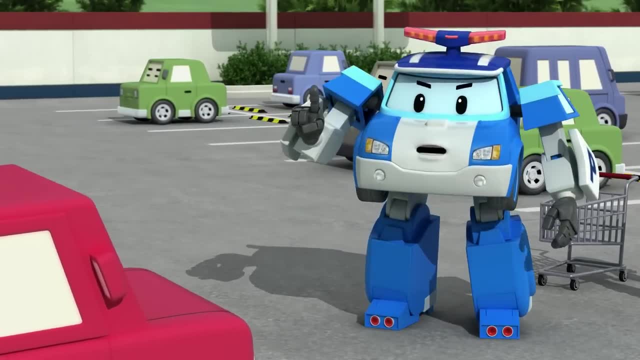 Parking lots are dangerous places. You should always watch your children in them. Oh, it happened so fast. As for you, ma'am, you cannot drive that fast when you're in a parking lot. I'm just so sorry. I was afraid I'd miss the sale. 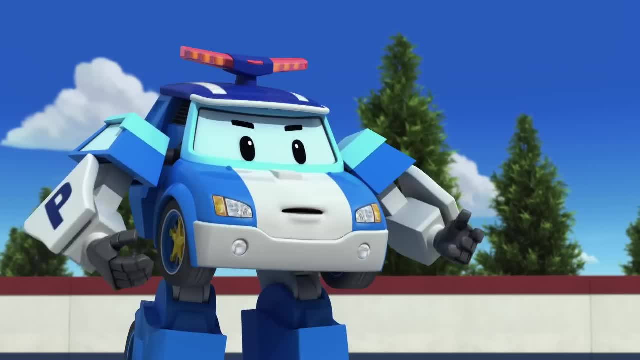 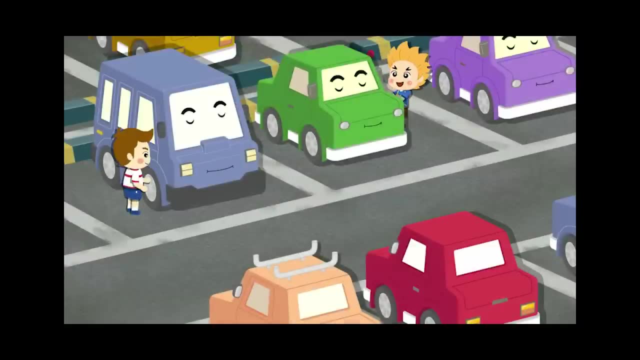 Kevin Susie, you both need to listen to me carefully and be cautious from now on. Right, You should not run or play in a parking lot because you never know when or where you're going to be. You should not run or play in a parking lot because you never know when or where you're going to be. 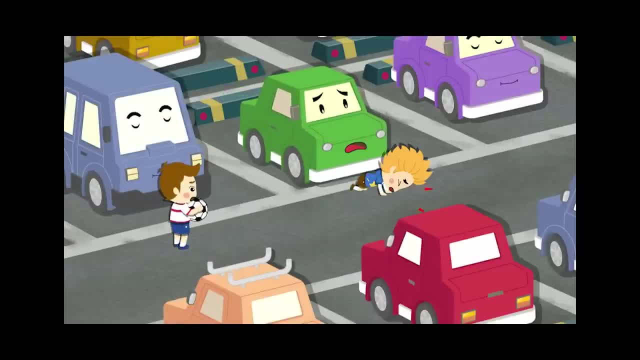 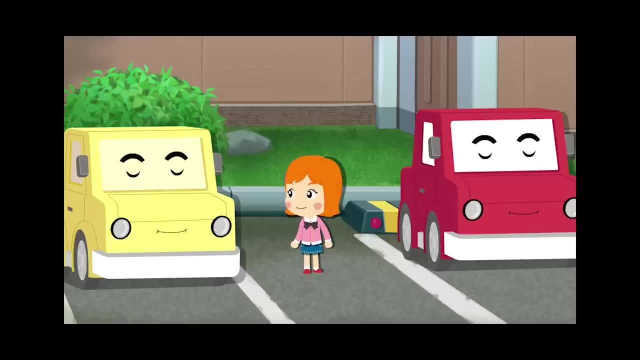 You should note that it's dangerous to make either a free Betty's sleigh or a twix. Yes, you should never use that해. You should always be very careful, especially when you're trying to stop the car, And you should know where a car may pop out. it's very dangerous. 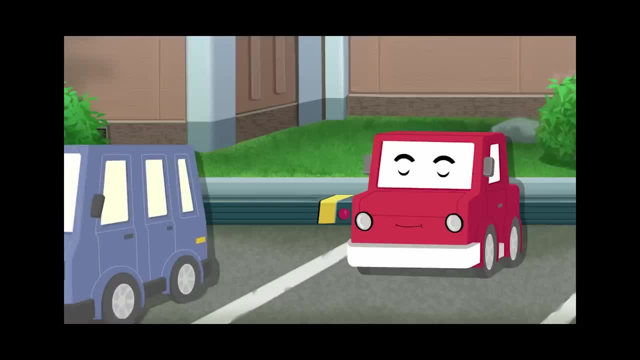 Kapoo, Kapoo, And it's easy to stumble over a speed bump or parking block, so you should always walk slowly and look where you're going. Also, remember before you get out of a car to make sure the car has completely stopped and make sure no cars around you are moving. 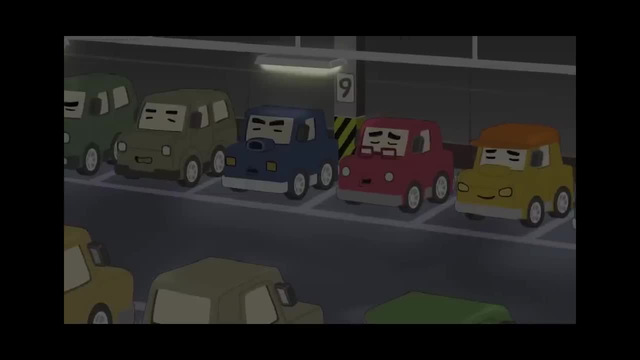 And make sure no cars around you are moving. When you are in a parking garage it is very dark and hard to see, So always be sure to show car. if there are peopleрушv. always be sure to walk with an adult. 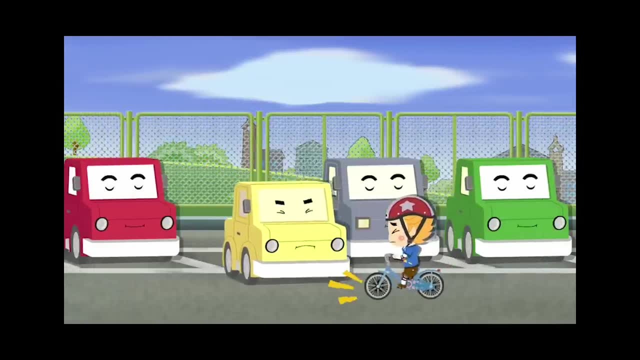 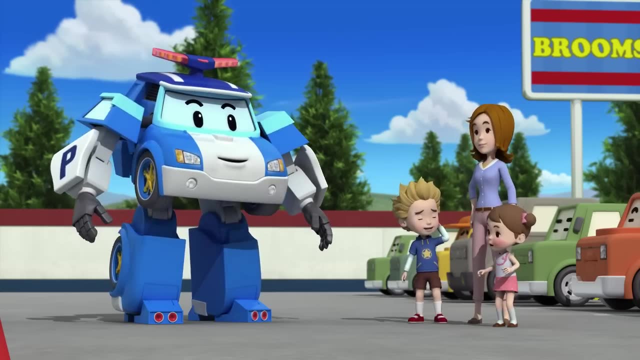 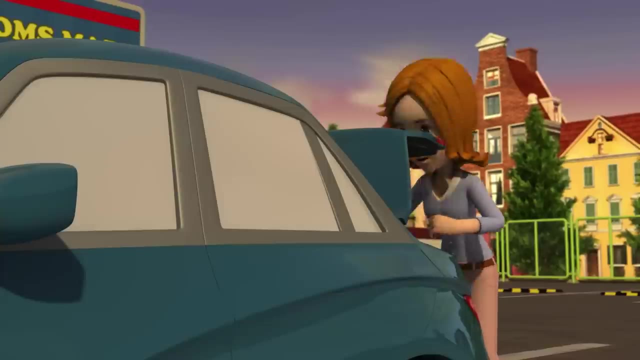 And also Kevin, you have got to know it's extremely dangerous to ride a bicycle or shopping cart in a parking lot. Understand- Yes, I do, Polly. Listen, Mom, are we ever going to get home? Almost done. 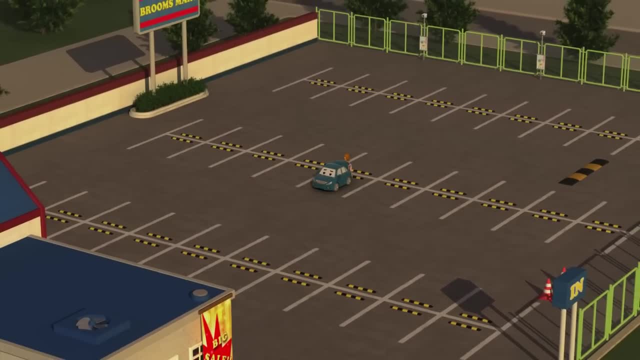 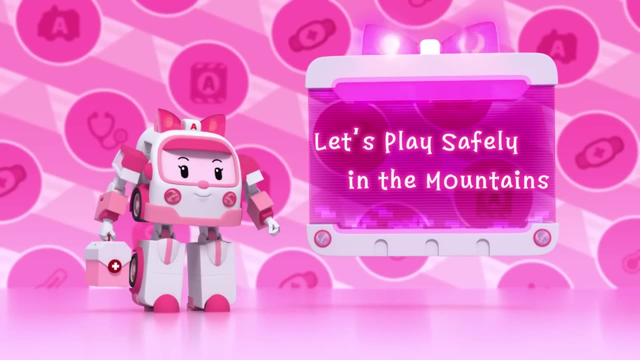 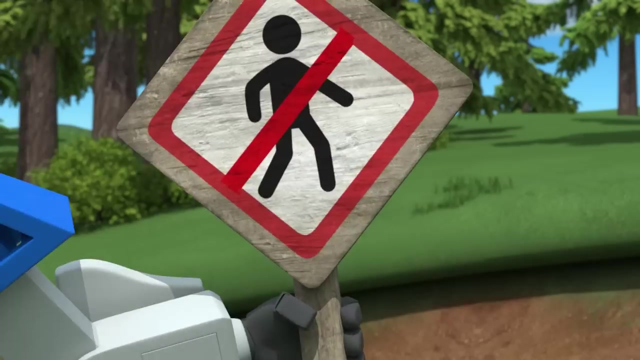 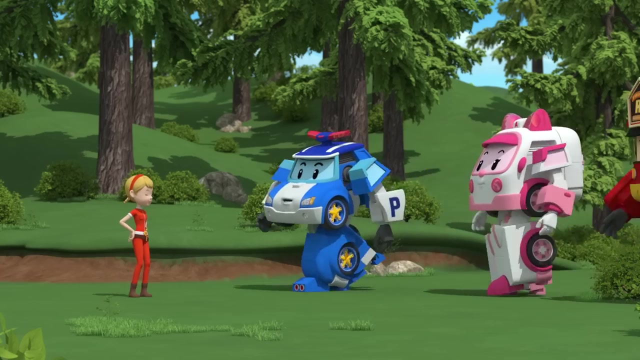 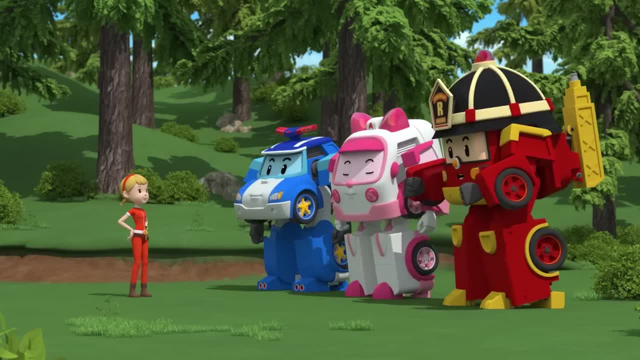 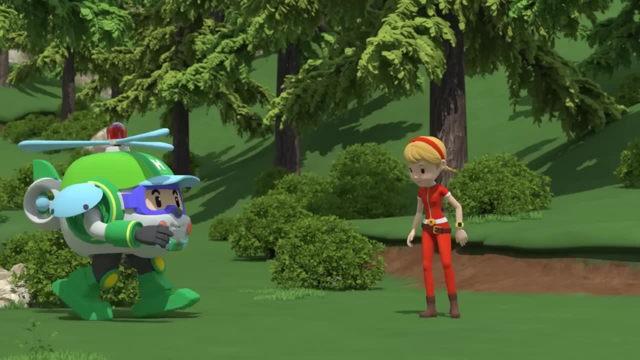 It all looks good. I didn't see any beehives or snakes around, Mm-hmm. thanks a lot, guys. Now this will be a safe place for the children to play. Jin, we're all ready for the treasure hunt. 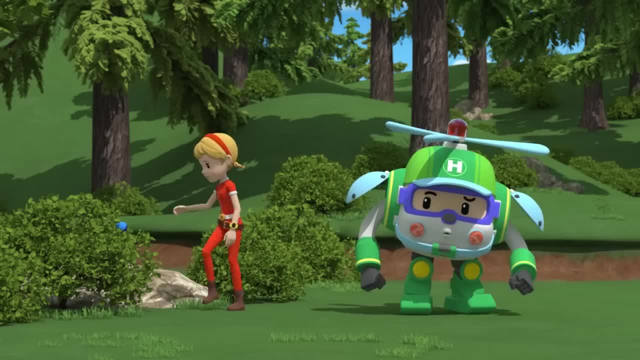 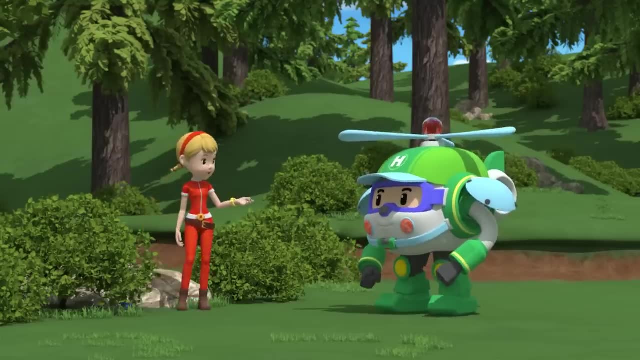 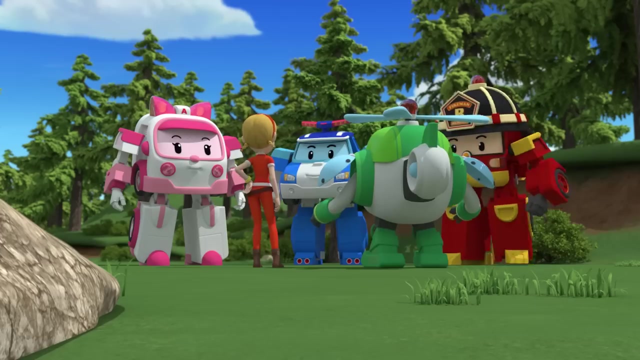 Mm-hmm, all right. Oh, Hallie, come on, That was too easy. Ah, A treasure hunt is the most fun when you really have to search to find the object That makes sense. Jin, if we're all done, we'll go on patrol. 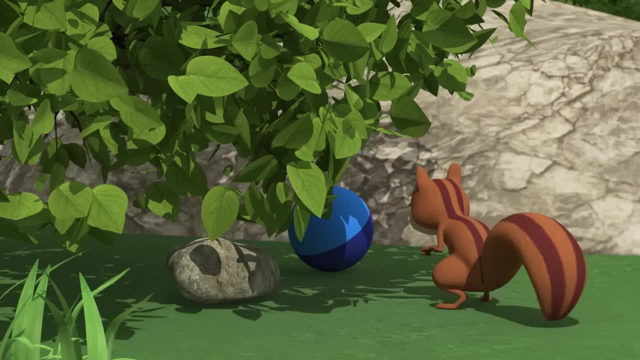 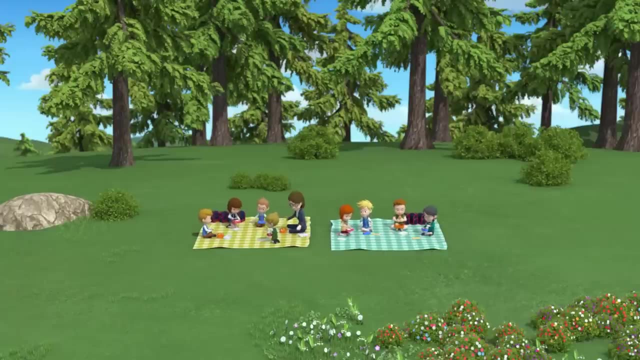 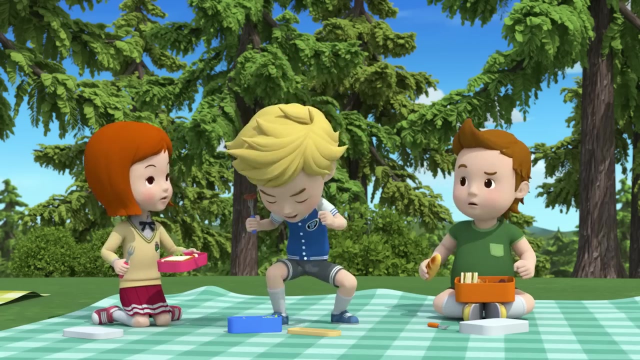 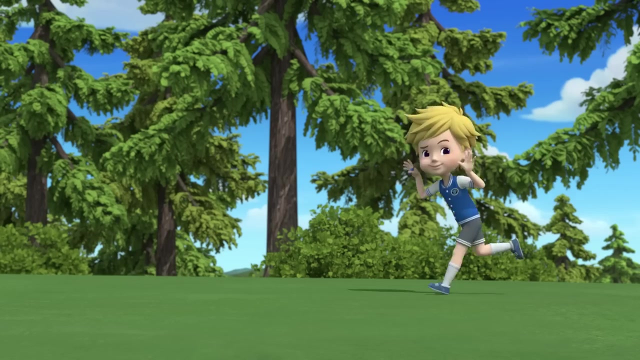 Mm-hmm. Okay, thanks again. Oh, that looks good. Look, It's a bunny. What Really She always falls for that. What, Peter? Give that back. No way, It's so delicious I'm gonna eat it. 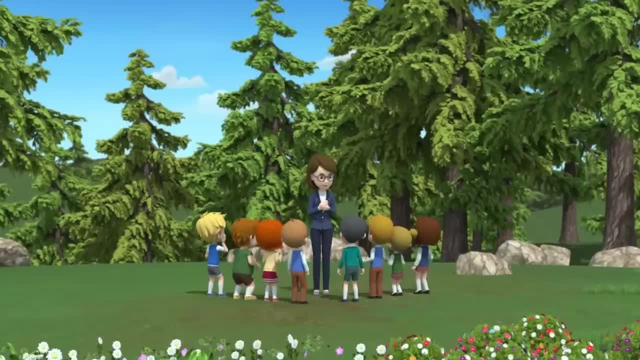 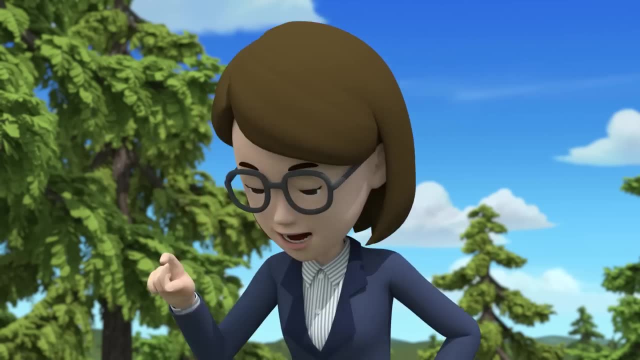 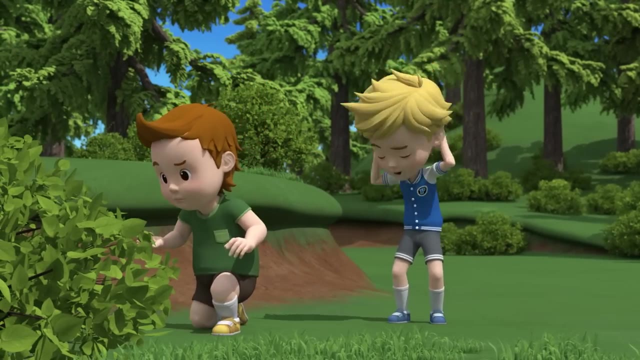 Give it back. All right, Are you ready for a treasure hunt? Yay, A treasure hunt. Just please stay in this area so nobody gets lost, understand? Yes, Where do you think it is Johnny? that spot's way too obvious. 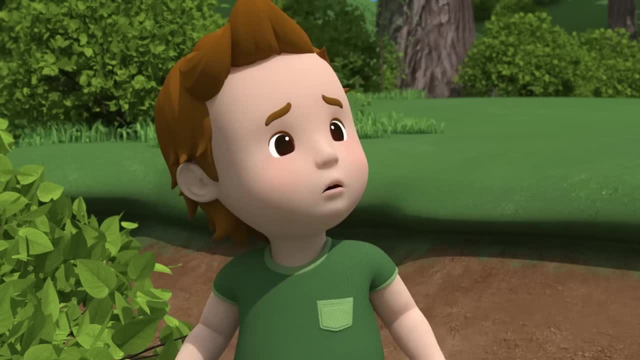 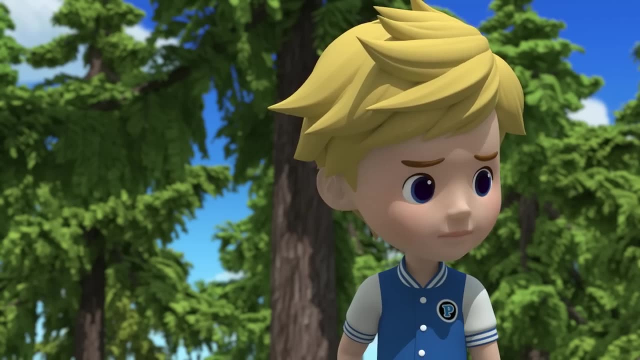 I found it. I got one too, Peter. they're gonna be all gone, Don't worry, Johnny, You're with me, aren't you? I'm a treasure hunt expert. Oh, They always hide it somewhere, like this. 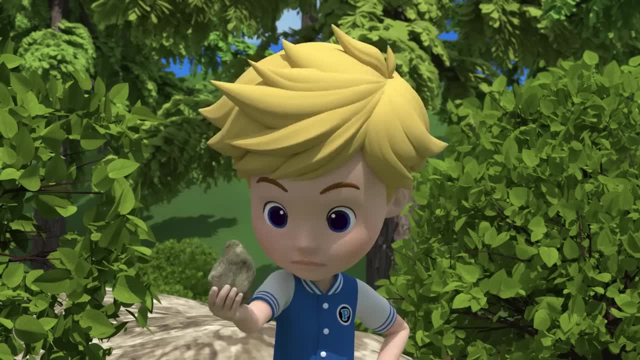 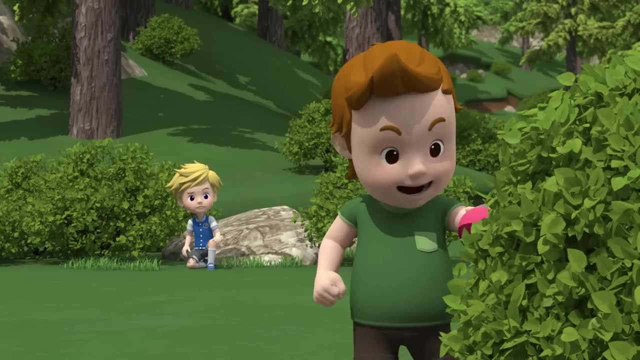 Stop, Peter, That's just a big rock. Huh, Well, that's odd. This looked like the perfect spot. Oh Look, I found one. Huh, I wonder what's in it. Hmm, Well, there's only one way to find out. 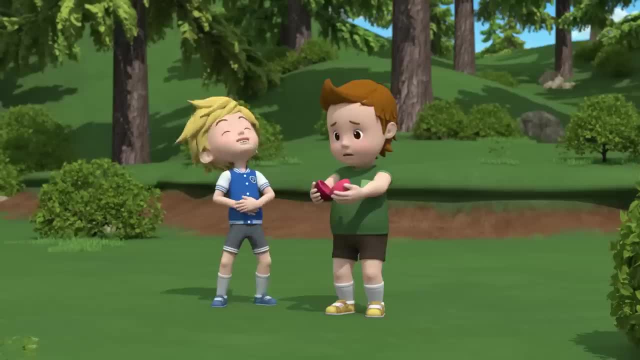 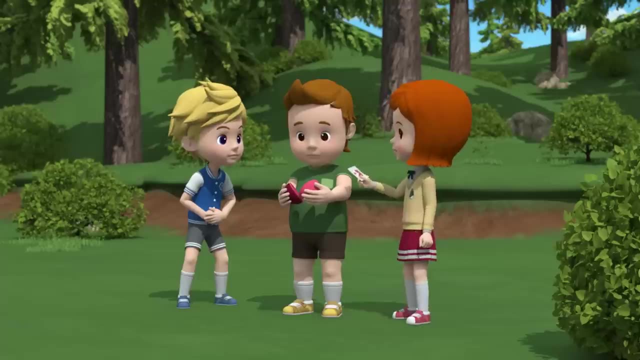 Huh, Huh. What's this? It's a ribbon. How pretty, Johnny. Johnny, I'll trade you my cake for that ribbon. All right, Thank you, Cindy. What You're not allowed to trade, what you find. 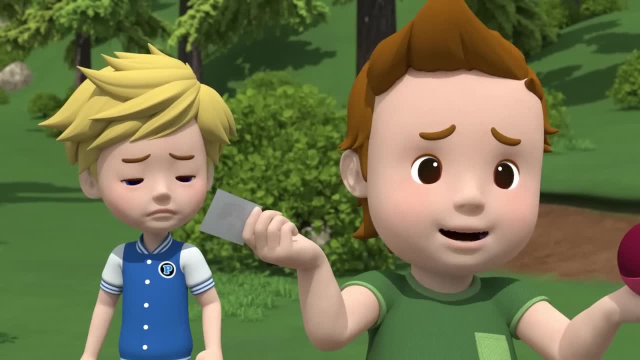 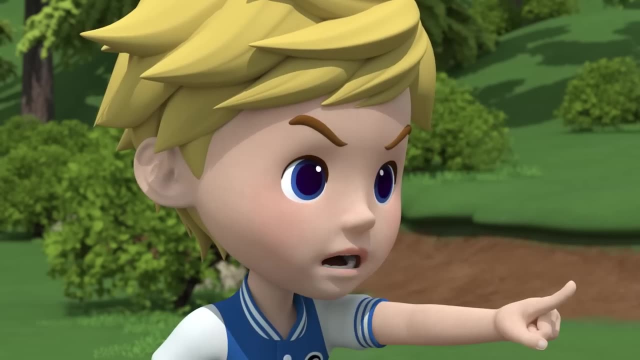 Peter, have you found one? The only thing he's found is a big rock. He told me he's an expert, but so far I don't buy it. You just wait. I'll find a better treasure than either of you. 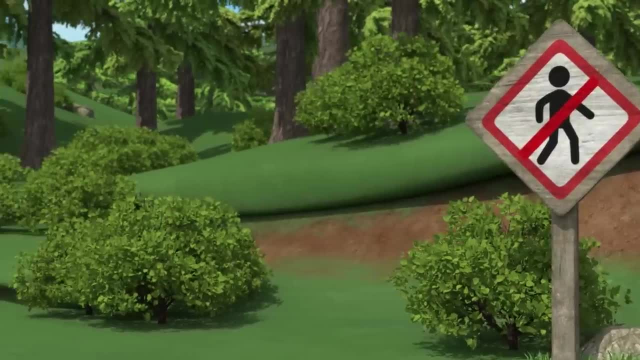 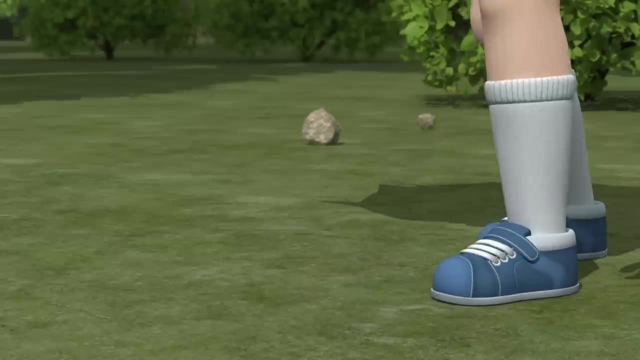 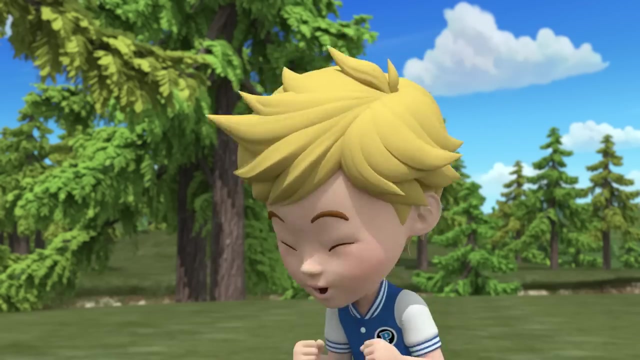 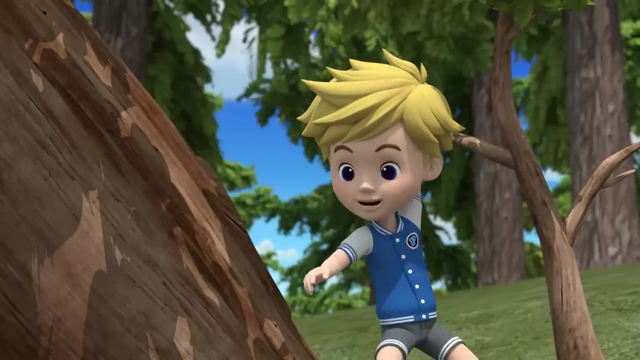 Huh, Huh, Hmm. There's nothing here either. Where did they put them all? Hmm, Huh, All right, It's about time I told them I'm an expert at this. I bet it's a great prize if it's hidden way out here. 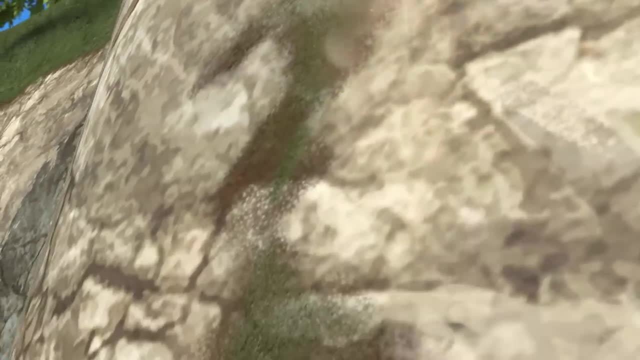 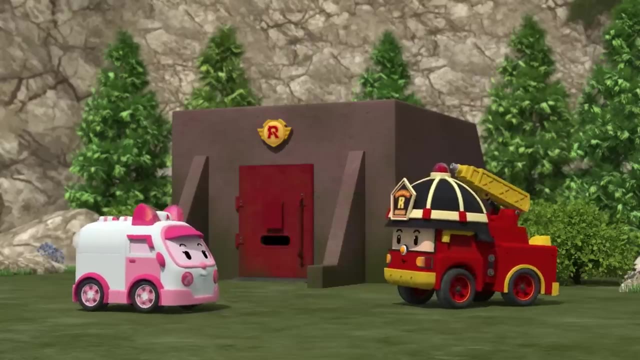 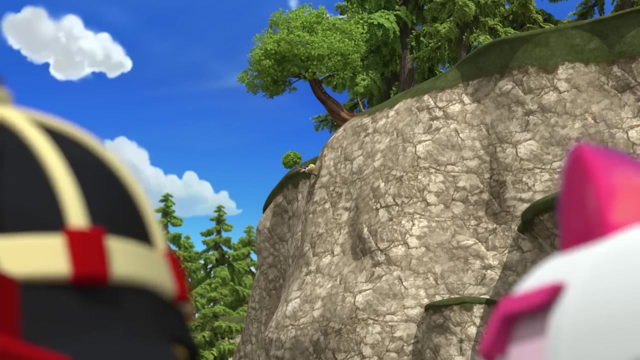 Got it. Ah, Help, Somebody help, I'm done checking the shelter. Should we head back? Can anyone hear me? Huh, Help. Did you hear that It's Peter? Ah, Ah, Oh, no, Please don't break. 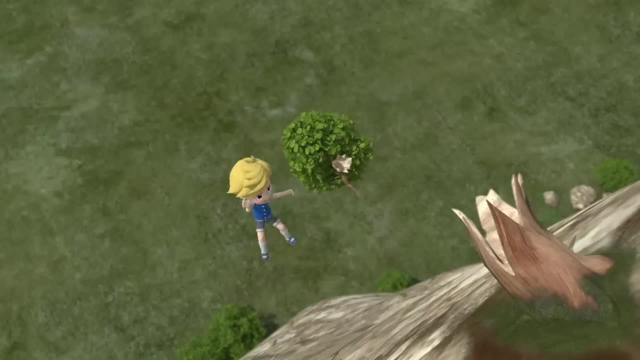 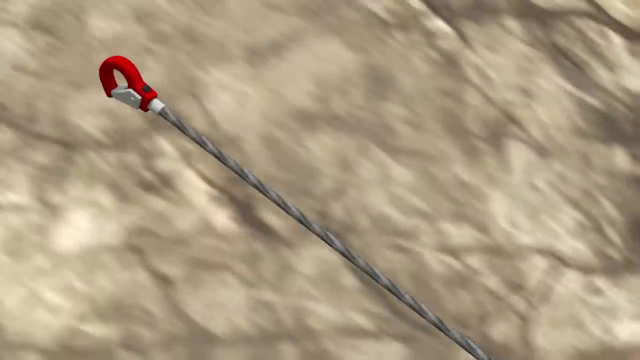 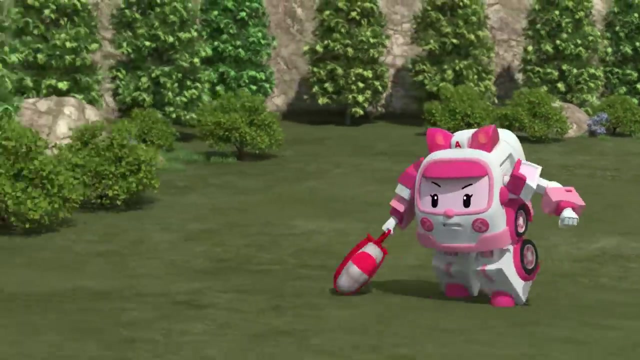 Peter Huh, Roy, Huh, Ahhhhhhhhh, Huh, Huh, Huh, Huh, Huh, Huh, Ahhhhhhhhh, Huh, Huh, Huh Dah. 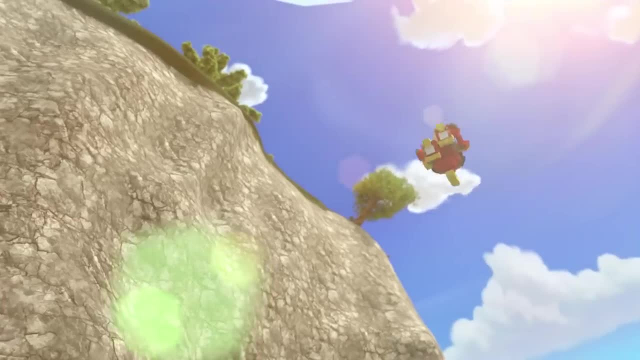 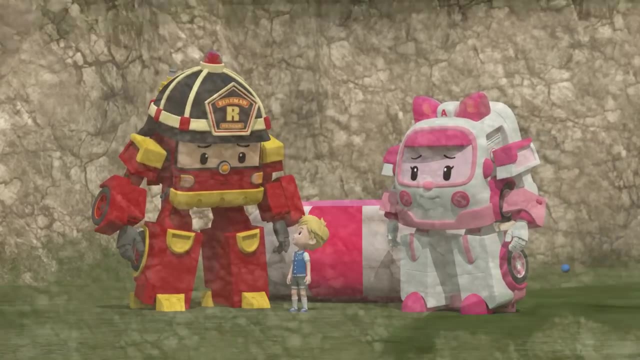 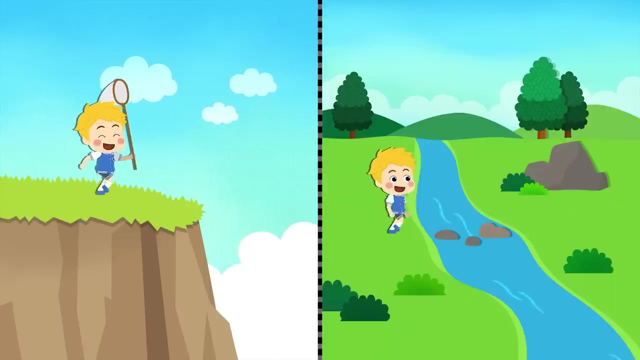 Dah Huh Huh Huh Ugh, Are you okay? Ugh, Huh, Huh, Huh, Huh Huh. That was a close call, Peter. I'm sorry, Amber, You shouldn't go far on your own while playing in undeveloped areas. 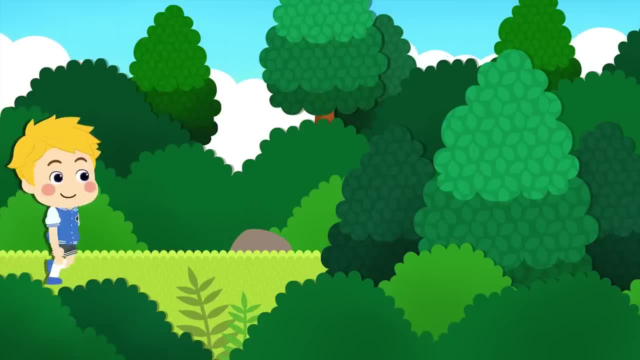 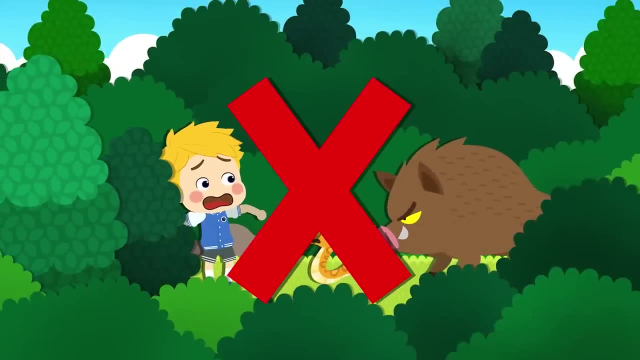 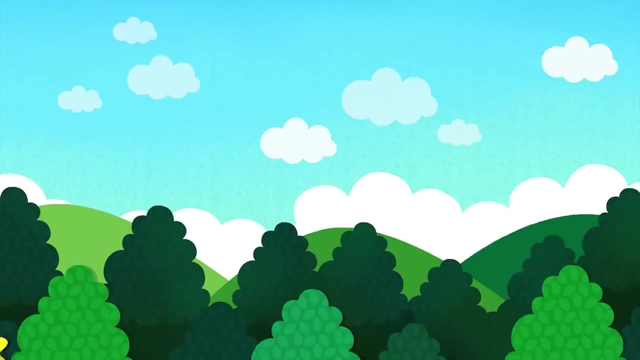 It could be very dangerous. In addition to unfamiliar terrain, you could encounter wild animals who aren't used to humans And don't ever pick or eat anything you find growing. It could be poisonous. There are a lot of beautiful things to see out in nature. 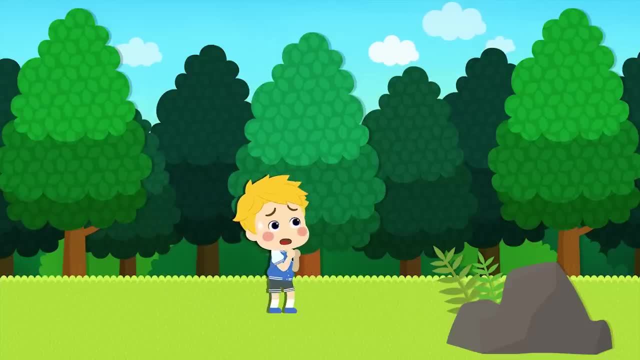 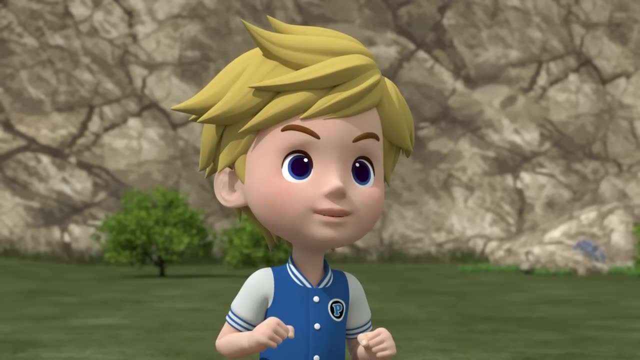 But it's also easy to get lost. Be sure to stay close to an adult. All right, Peter, Sure, Amber, I'll be much more careful the next time. This was a great trip, huh, Yeah, Peter. so did you find anything? 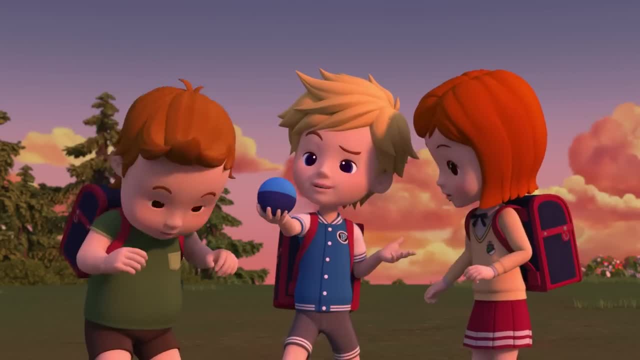 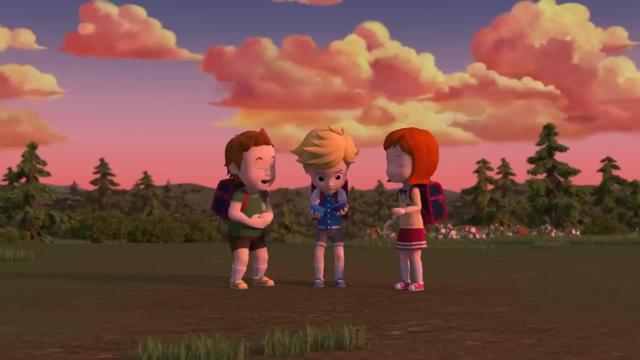 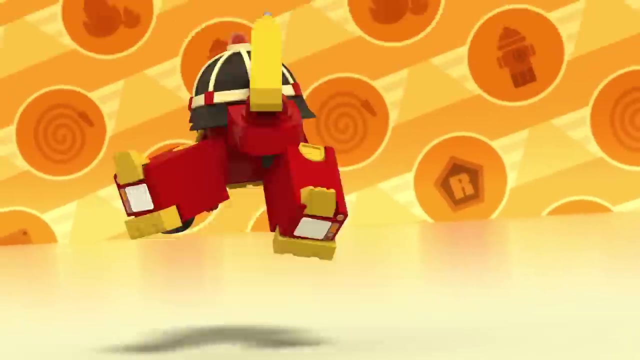 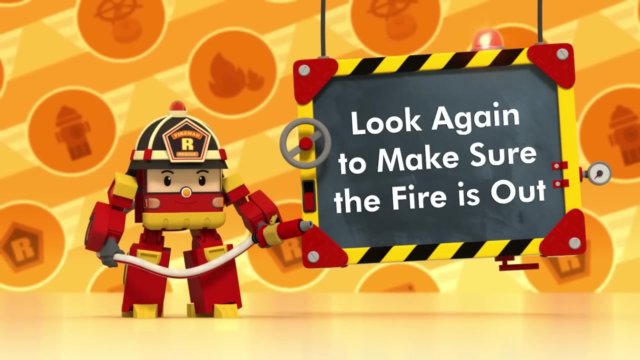 Sure, I did, And I haven't even opened it up yet. Drum roll please, Ta-da. What? Seriously, It's empty After all that. there's nothing, even in here. Look again to make sure the fire is out. 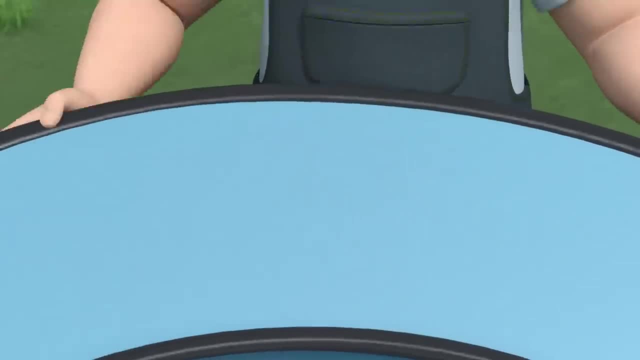 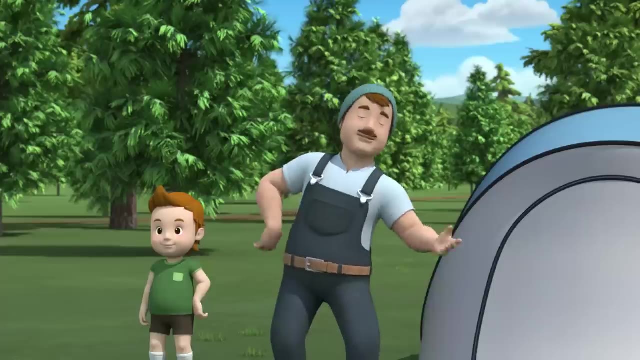 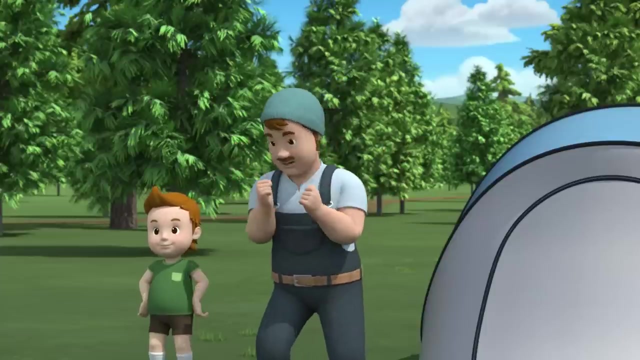 So tired. Huh, Huh, Huh, Huh, Wow, Awesome. Did you buy another new tent? I did, The latest model. It's the highest-priced tent ever: Instant setup, Cool in the summertime, warm in the winter. 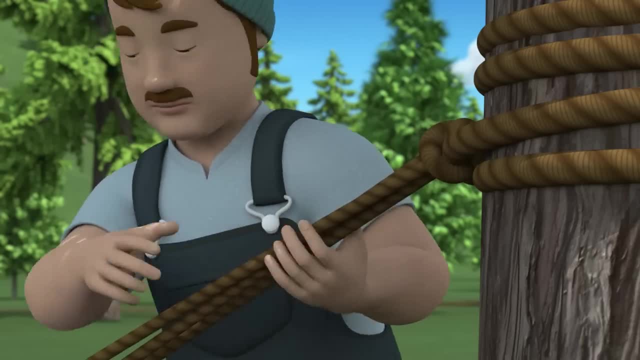 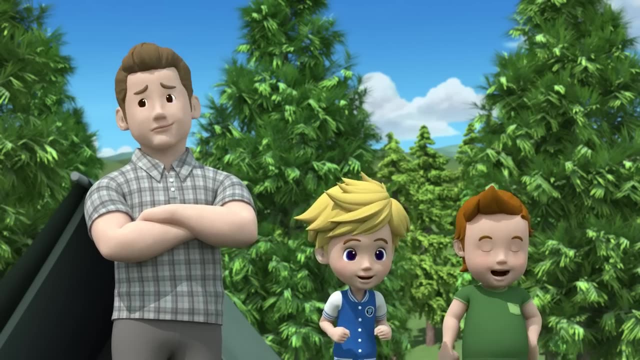 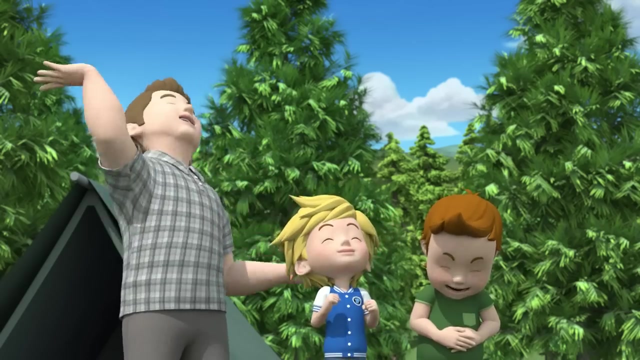 Wow, Ta-da, Johnny. what is that? Well, it's called a hammock. You tie it between trees and use it as a bed. Allow me to demonstrate: Hup, Hup, Hup, Hup, Hahaha. 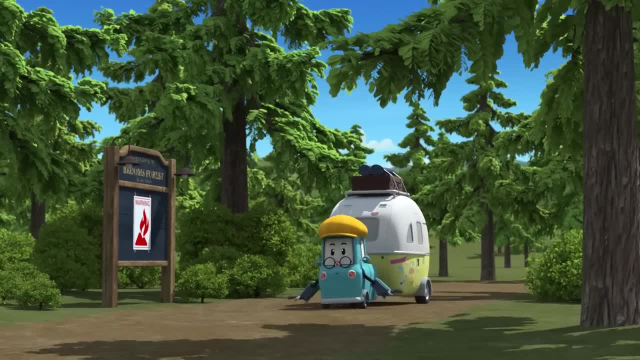 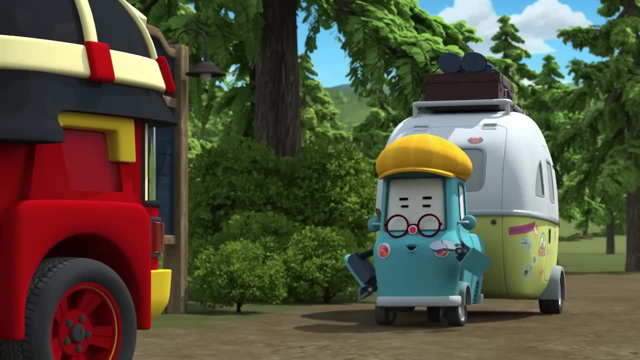 Oohoohoohoohoo, Huh, Roy, hi there. Long time Camp Camping up here. Yup, The weather's perfect for it. How on Earth could I stay home? Look around The world is so wonderful, Haha. 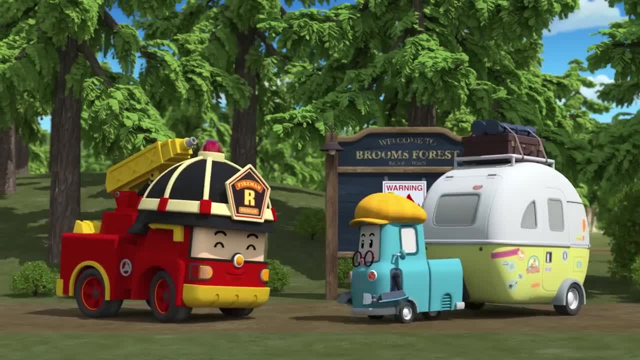 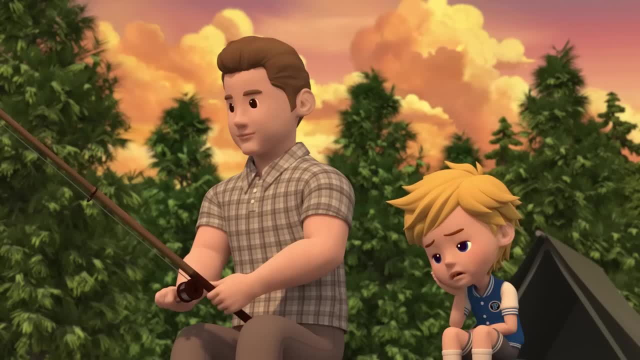 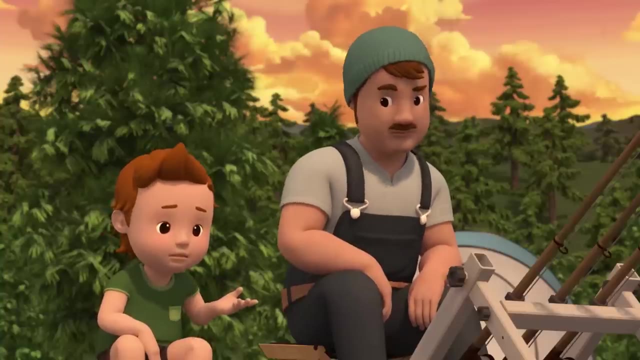 Then have a wonderful time. Camp Always do. Mmmhmm, I must remember to check the camping ground tonight. Oh Dad, you still haven't caught one. Just keep waiting. Fishing is all about patience. Are you certain there's fish in there? 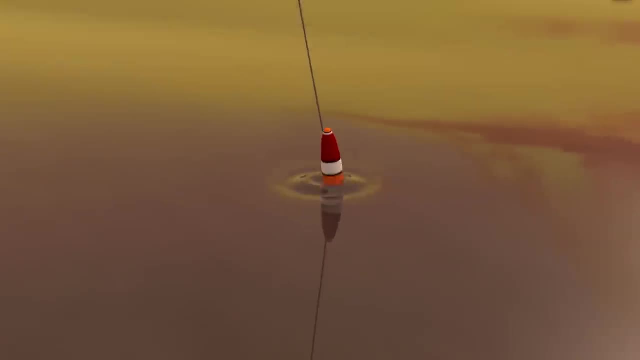 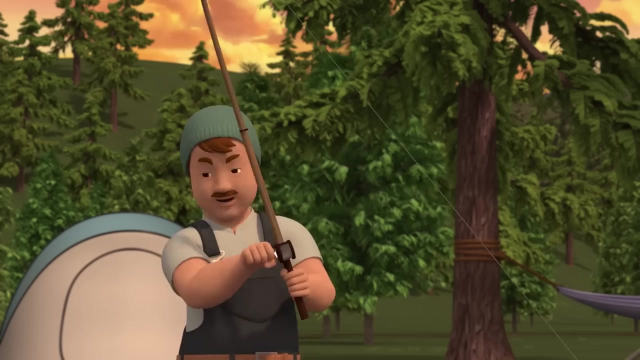 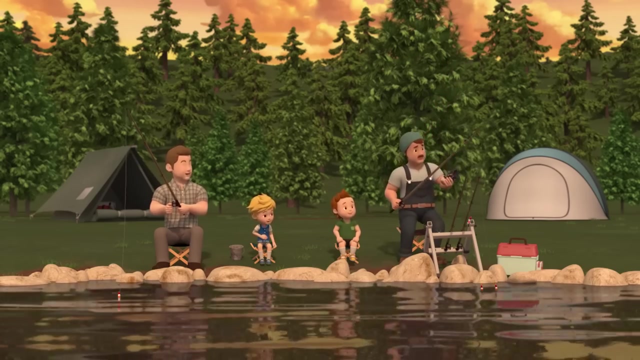 Shh, The fish will never come near us if they hear you. Huh, Dad, The floaty thing just moved. Yeah, It's on Heavy one Feels like a giant one too. Come on fish, Peter. just keep your eyes on your dad and see how a real fisherman does it. 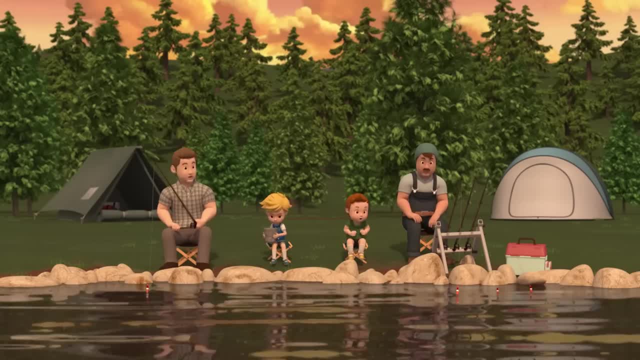 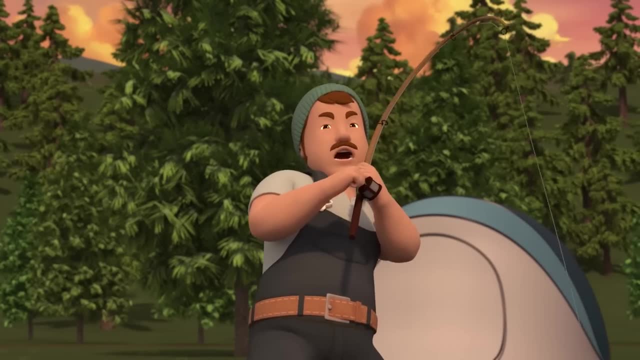 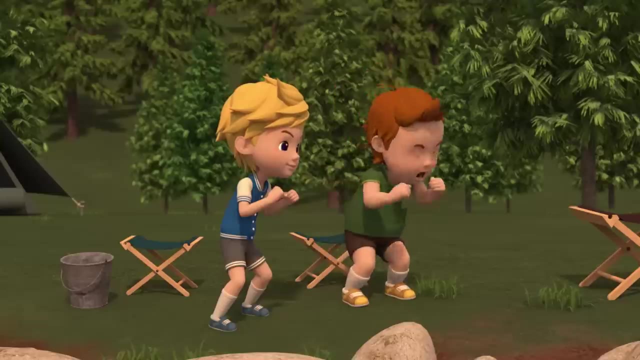 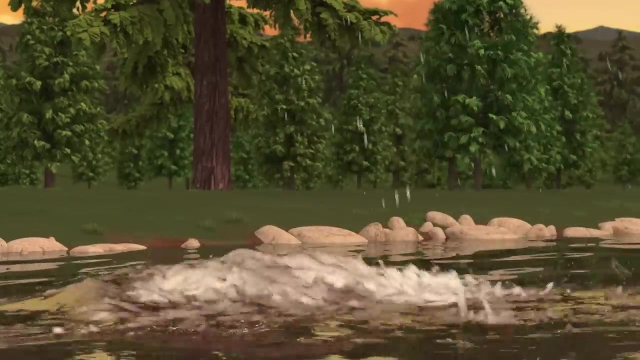 Uh, you've said that like a dozen times though. Huh, Robert, a little help, Hang on, Come on, You can do this. Dad, Dad, Go get him D-Dad. Wow, It's so big. 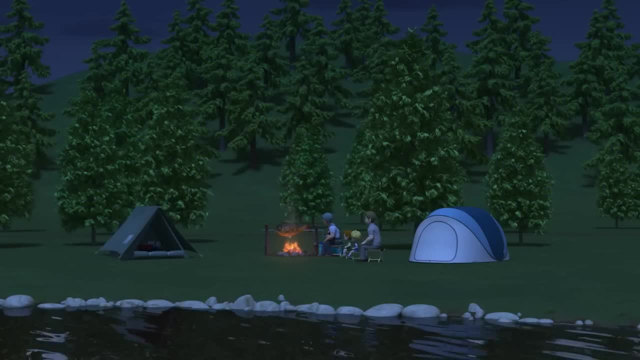 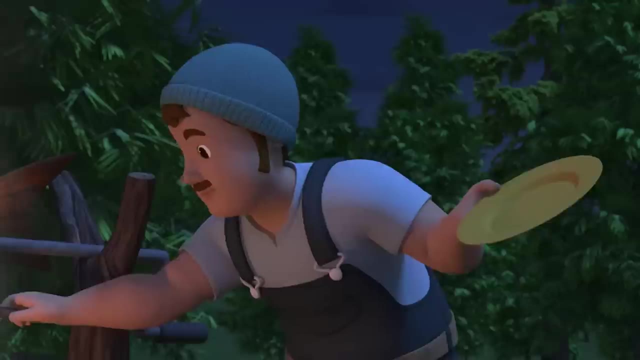 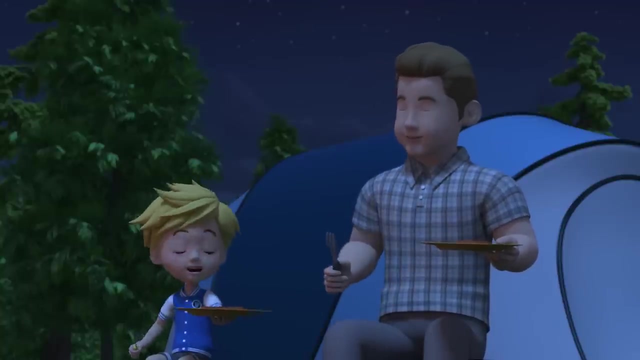 It's so big. Wow, It smells great, Dad, I want to eat it right now. Well, it's all cooked. Try some. Wow, Thanks, Dad. Wow, So good, You're right, It's awesome. Sure, That's because I'm the one who caught it. 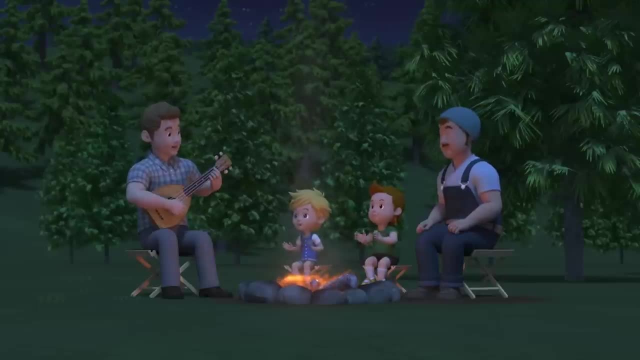 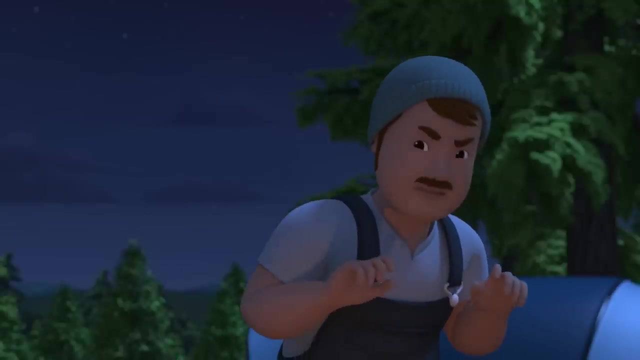 Ha-ha-ha-ha-ha-ha-ha, Ha-ha-ha-ha-ha-ha-ha-ha. The girl was just walking along and she heard something, And then the monster went Gah. 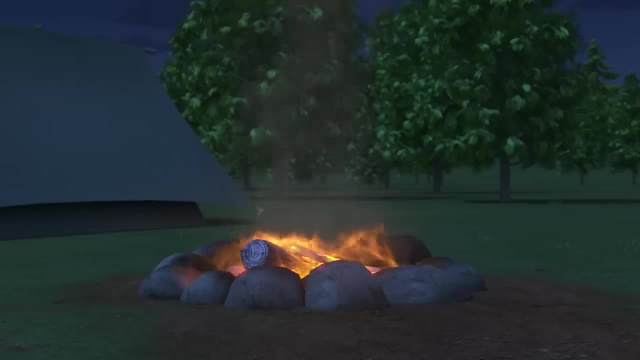 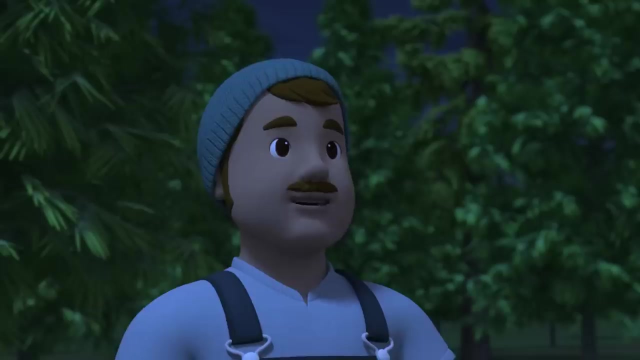 Wow, Ha-ha-ha-ha-ha-ha-ha, That one. there is the North Star. Long ago, sailors used that star to navigate. And see that one. Huh Shh, We should call it a night. 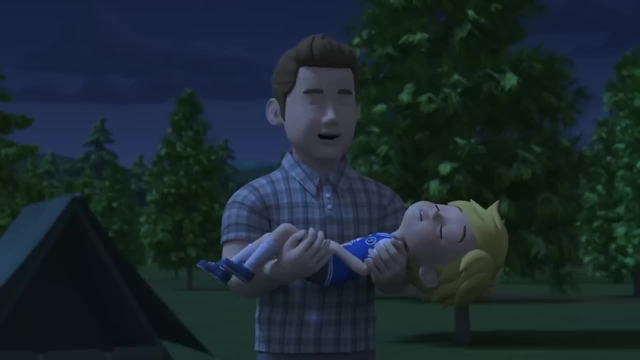 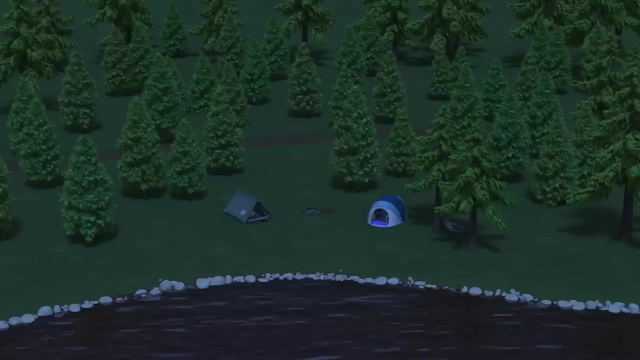 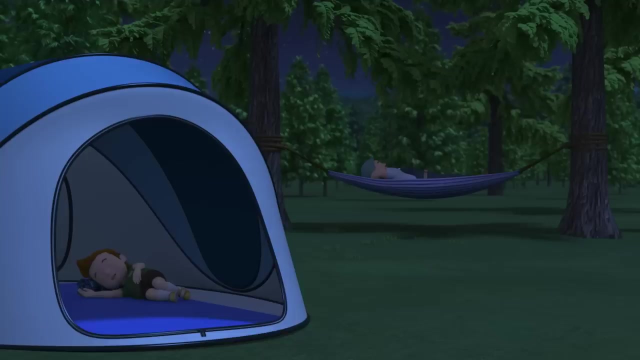 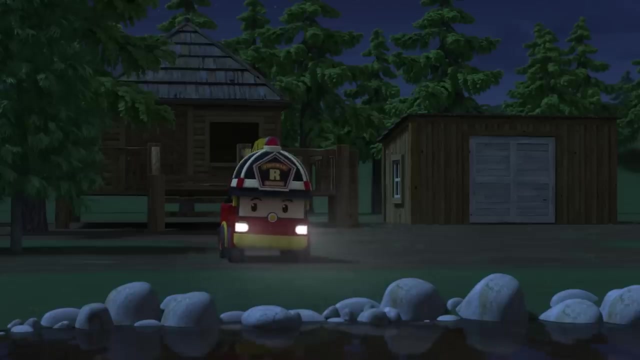 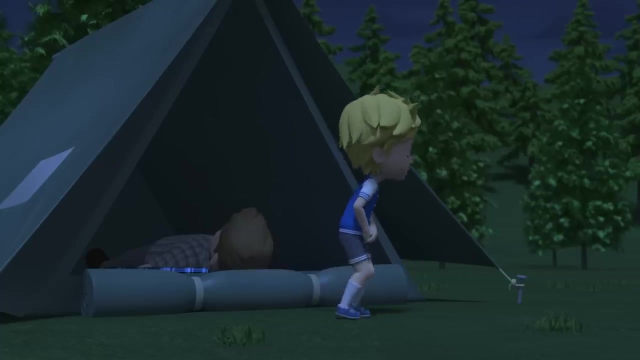 I'll clean up the campsite. Turn in. They're having a great time. Well, looks good. Now I'll check the other site: Bathroom, Bathroom. Huh, F-fire. The tent is on fire. What Johnny? 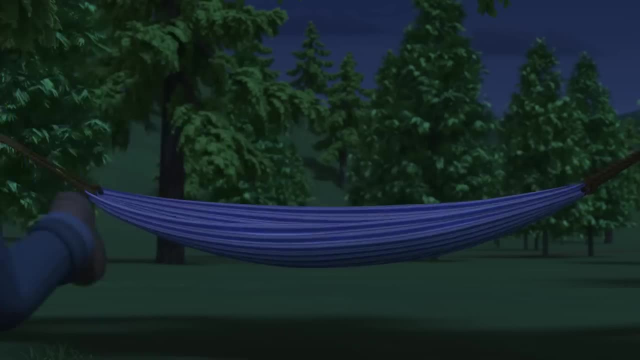 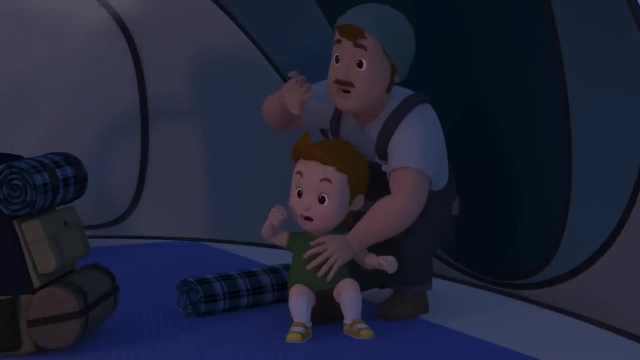 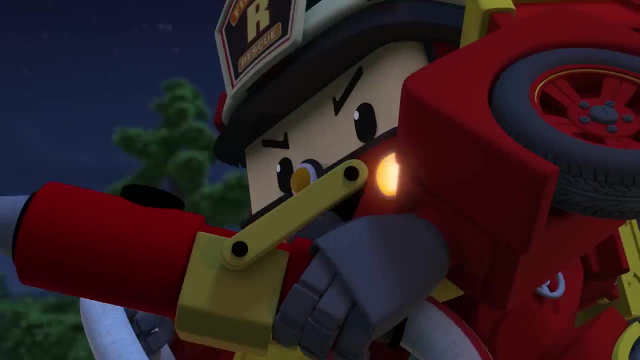 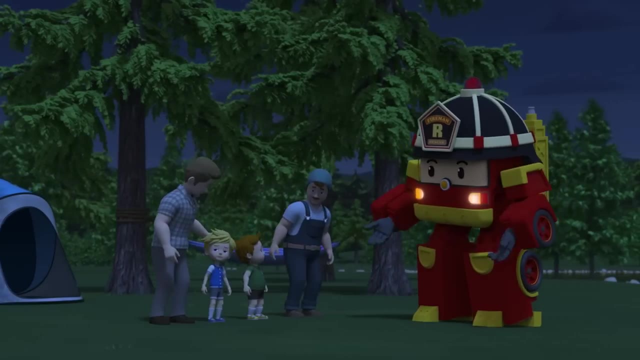 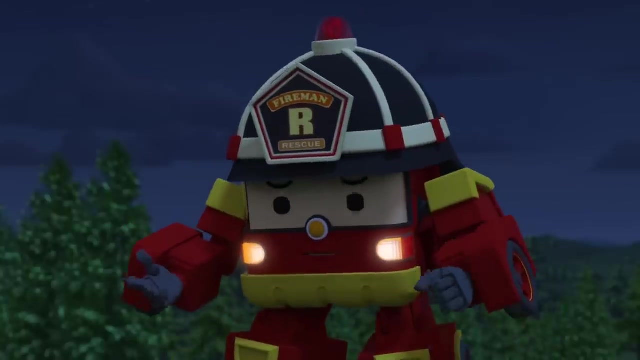 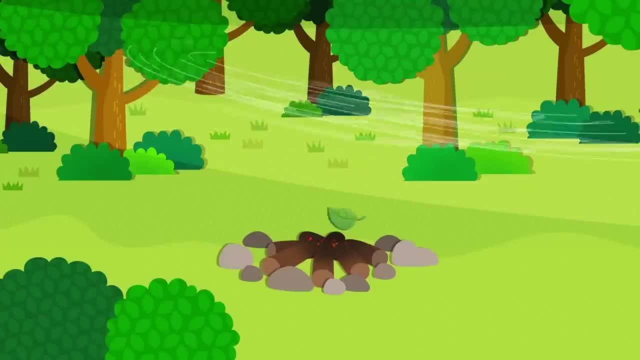 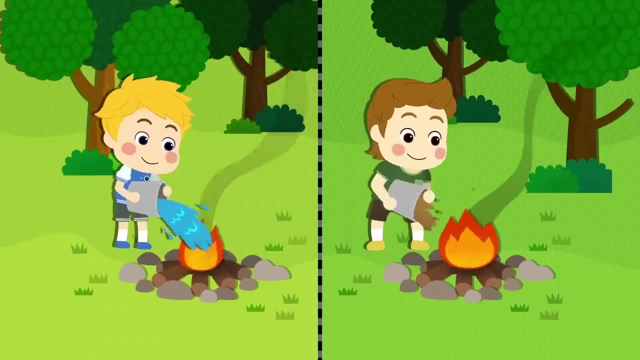 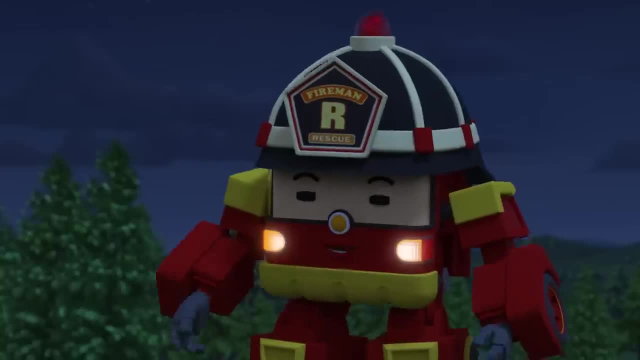 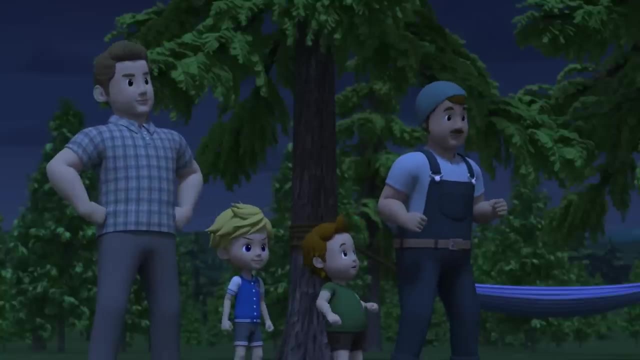 It means a lot of things: to be sure the fire is absolutely out and bring a fire extinguisher, That way, if there's a problem, you can handle it. I sure will Thank you, Roy, But Dad, where will we sleep though? 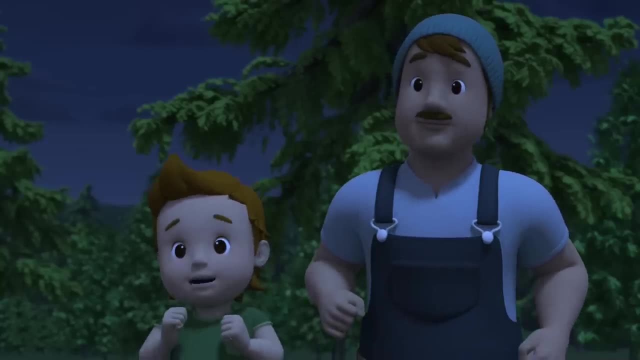 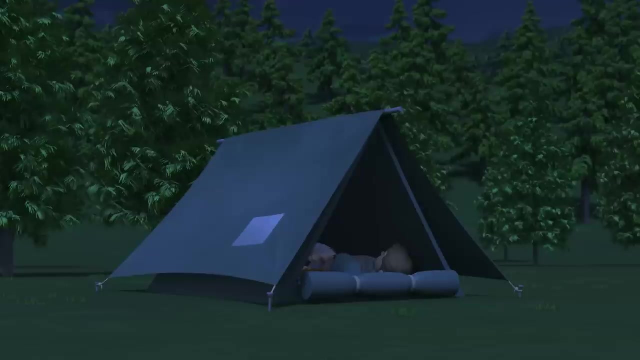 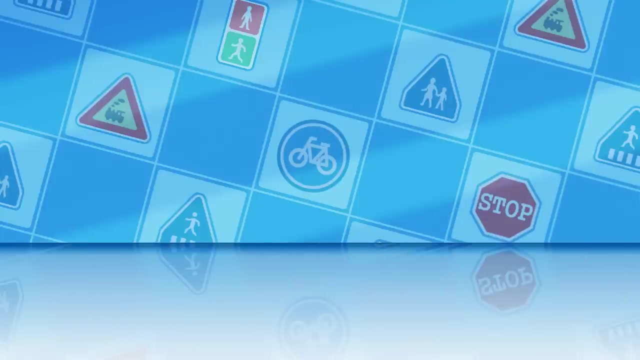 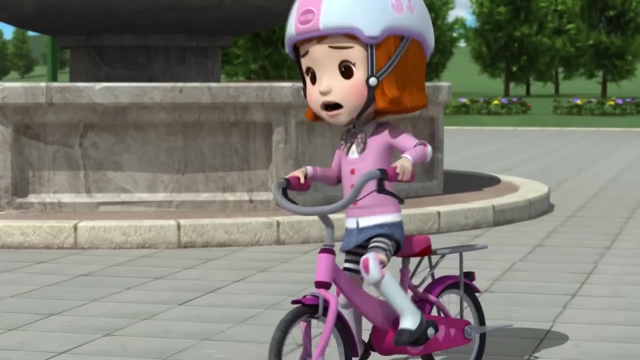 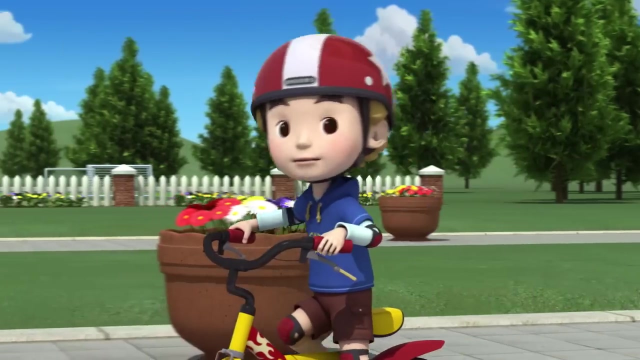 Come on, you can share our tent, Are you sure? Thank you, Mr Robert. It's so packed, Jenny, just try to balance. okay, I am trying to, but I can't. How are you going to pass the bike exam riding like that? 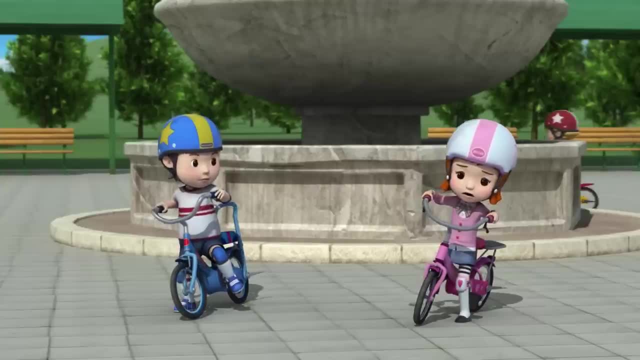 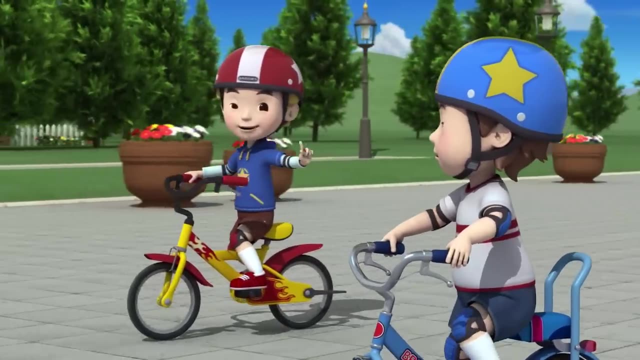 I will pass it. Look here, Jenny, Watch me do it. Here goes, Doug, you're kidding me. No way you're going to pass like that. Watch how it's done. Yeah Well, look out, Ta-da. 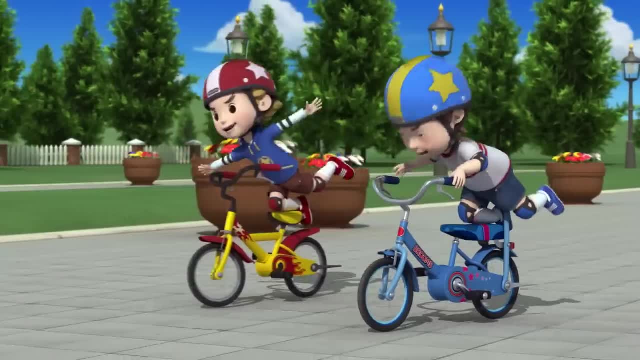 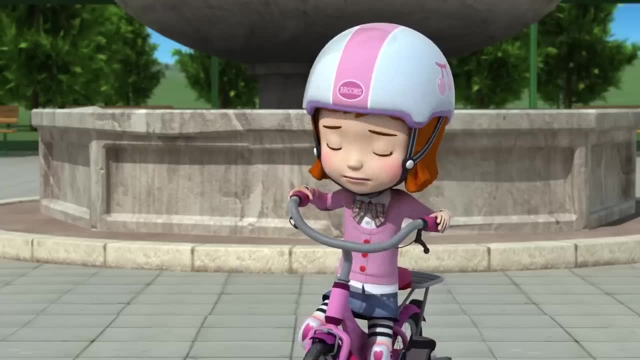 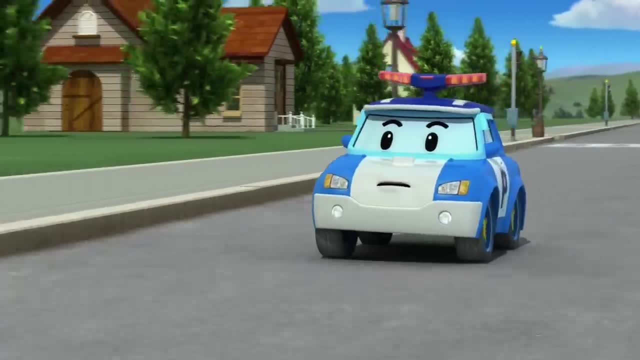 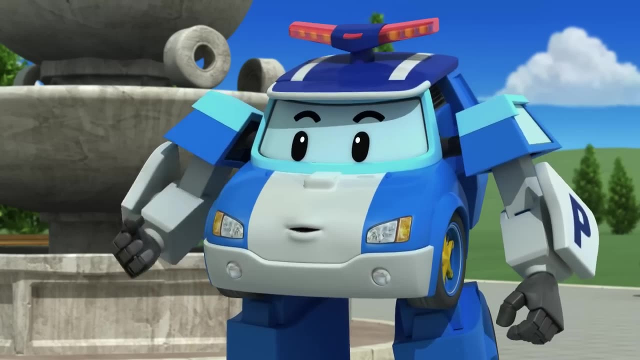 Ah, Ah, Ah, Huh, Ah, Ah, Ah, Ah. Ah, You all right, Yeah. Thanks a lot, Polly. Practicing riding your bike? Yeah, But it's hard to learn to ride all by myself because I keep on falling down. 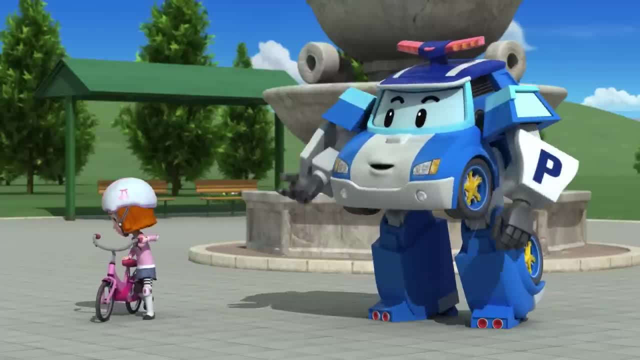 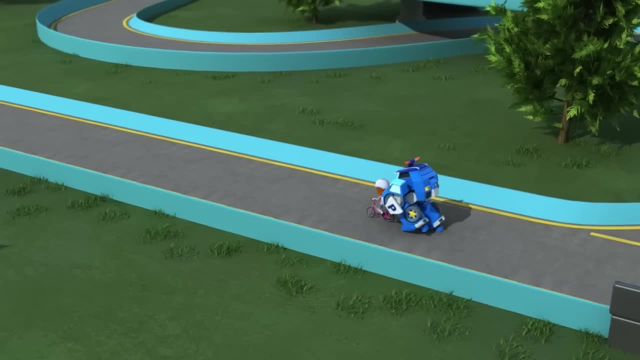 Oh no, I've got an idea. I can help you learn how. Yeah, Mm-hmm, Hooray, Hooray, Ha-ha-ha-ha-ha. Ah, I think I'm going to fall down. 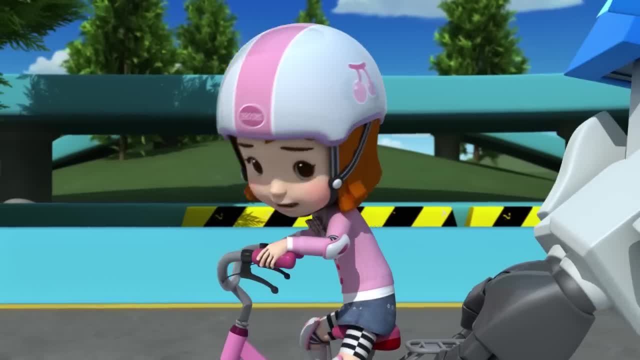 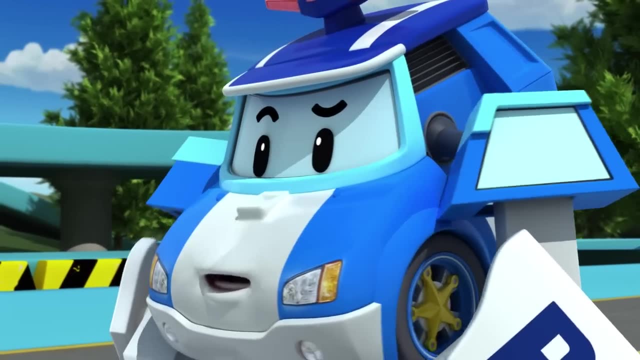 Jenny, don't look down at the wheels, Look ahead. Uh, I'll try, That's good, And pedal a bit faster too. I'm scared You can do it. If you pedal too slowly, then you'll fall down. 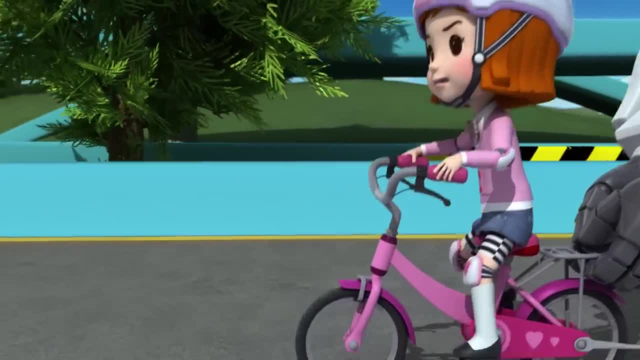 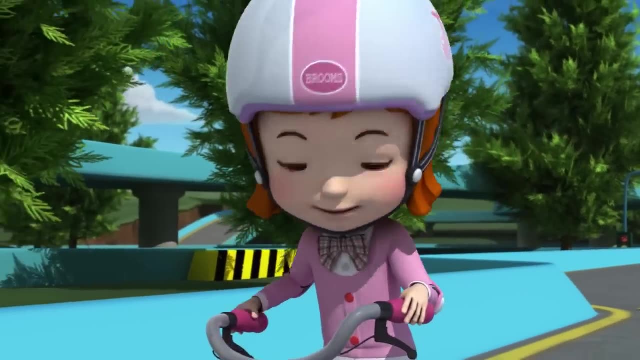 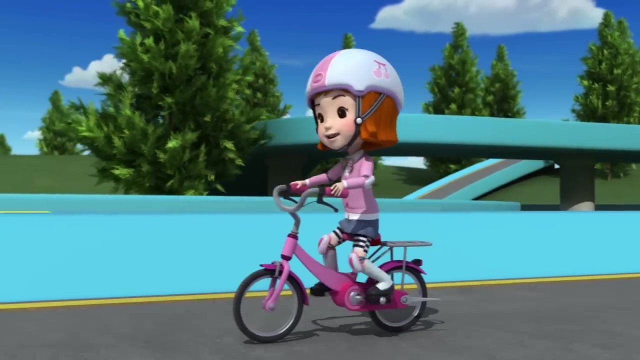 You can trust me. Here goes: Wow, I'm doing it. Polly, are you holding on tight? No need, You're doing fine on your own, I am. Ah, It's working. I'm riding all by myself, Be careful. 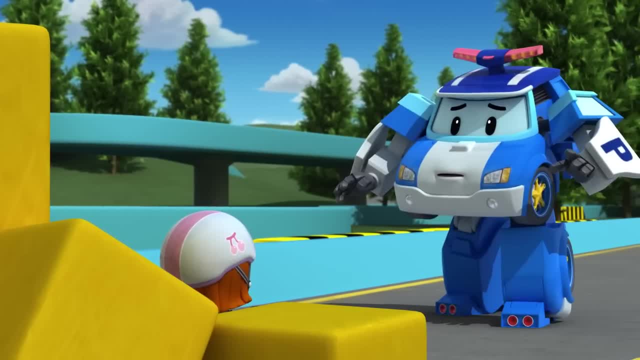 Ah, Are you okay? Ha-ha-ha, I'm doing just fine. From now on, look ahead, You've become quite a rider, Jenny. Well, if so, it's all because of your help. Remember, Jenny, when you ride your bike, rule number one: safety first, at all times. 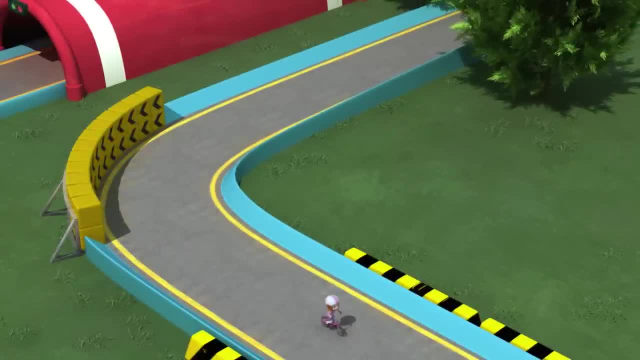 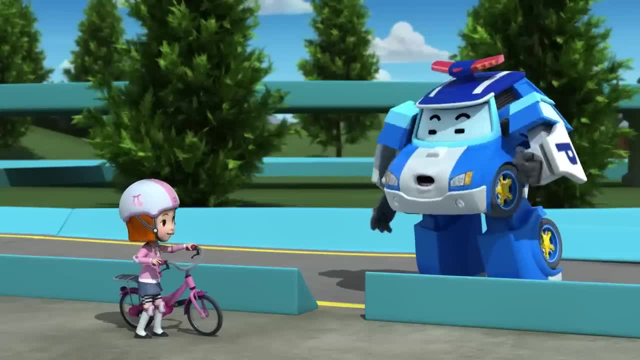 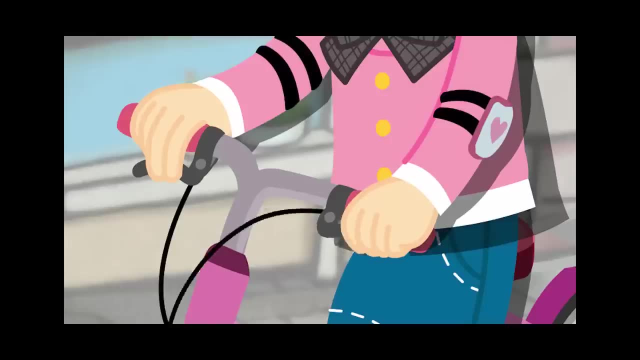 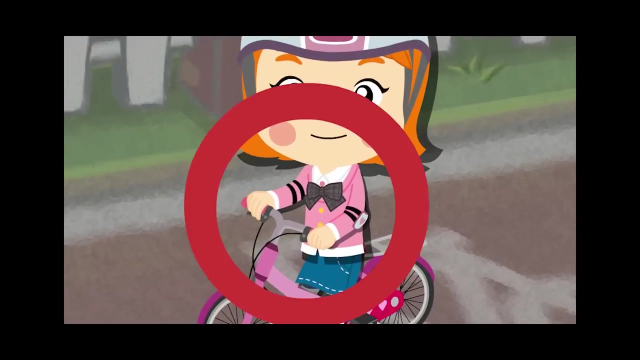 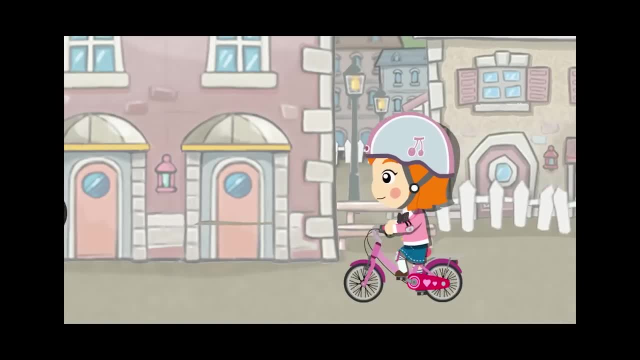 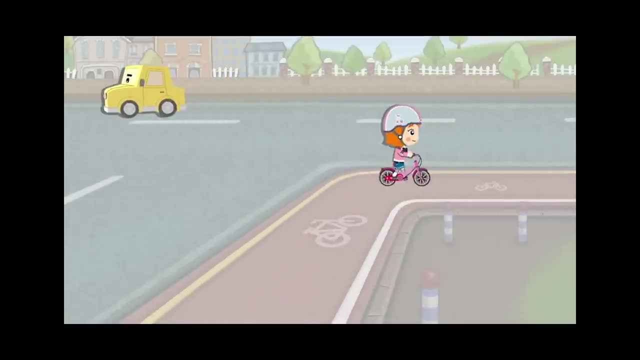 When you're going downhill, you can build up speed quickly, so it's important to use your brakes and stay in control. When you're riding on the road, it's very important to use hand signals to let others know when you're turning, slowing down or stopping. 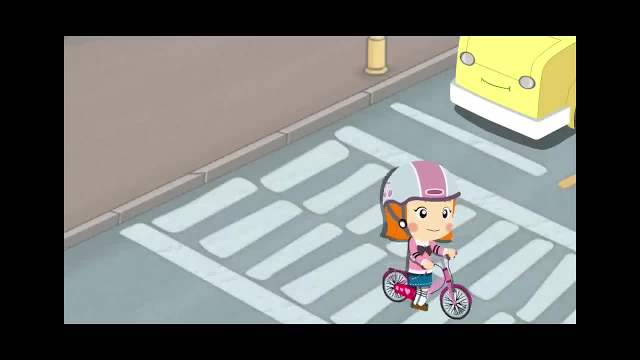 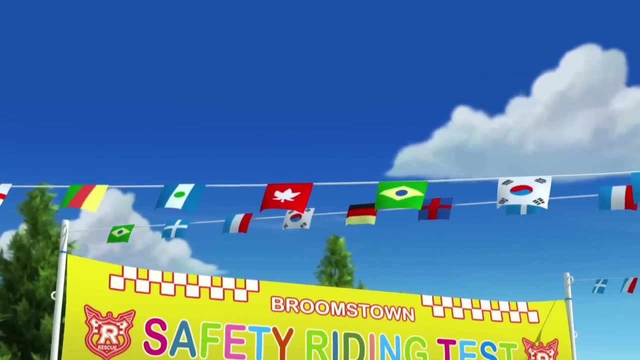 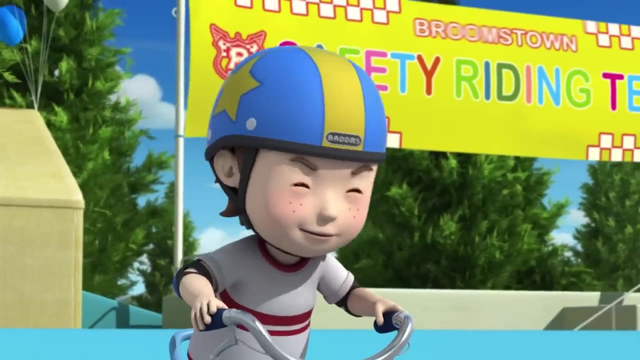 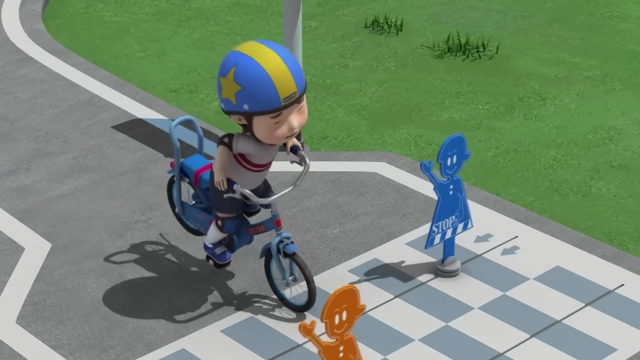 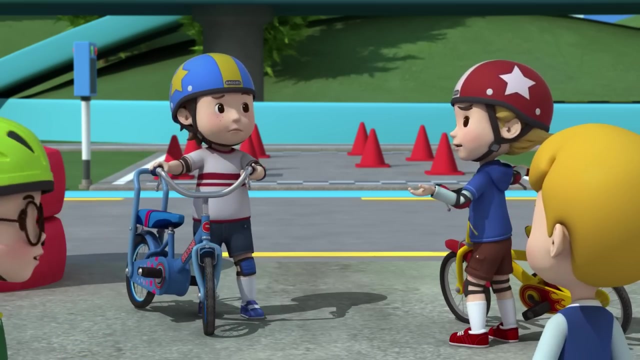 And when you cross the street you must get off and walk your bicycle. Ha-ha-ha, You're doing great, Jenny. Thanks a lot, Polly. attention, the bicycle safety exam is about to begin. wow, that test was too hard, that's too bad. watch and learn, I'll show you how it's done. oh yeah, let's do. 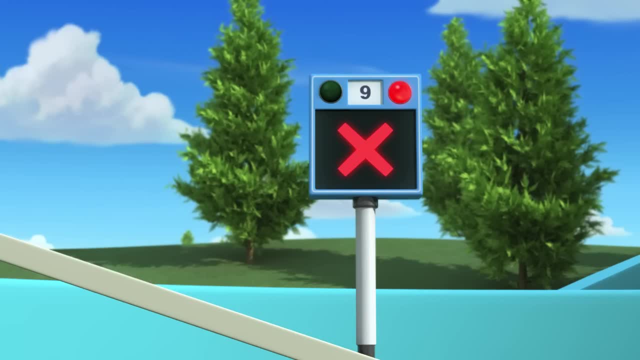 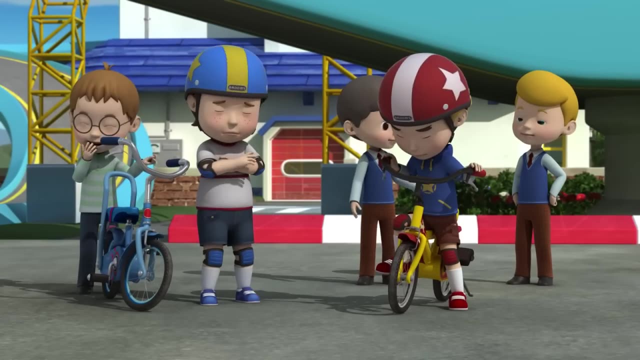 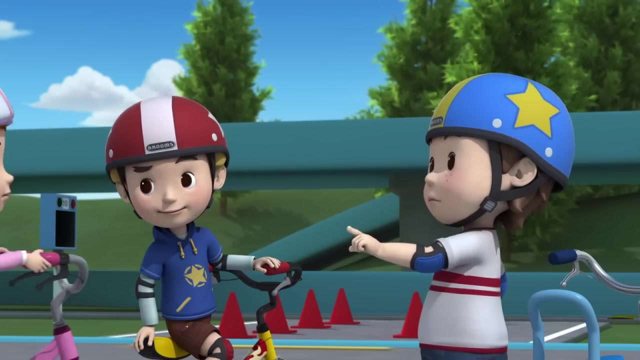 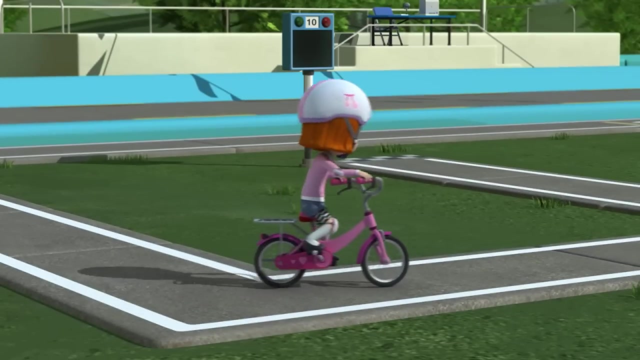 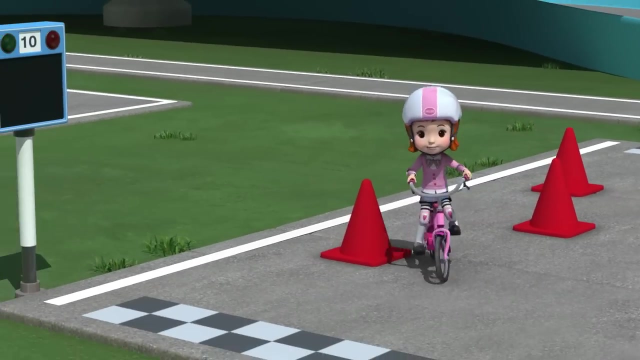 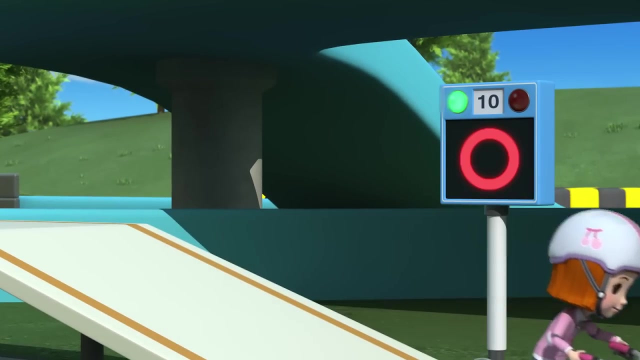 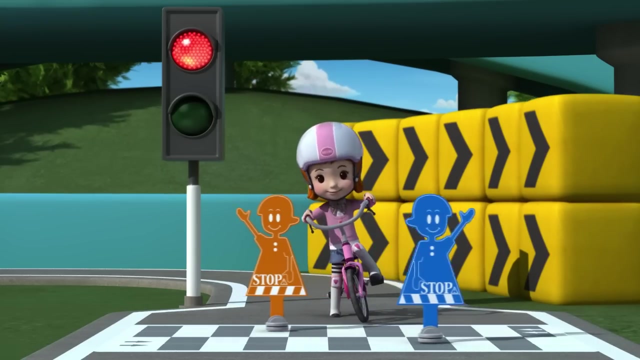 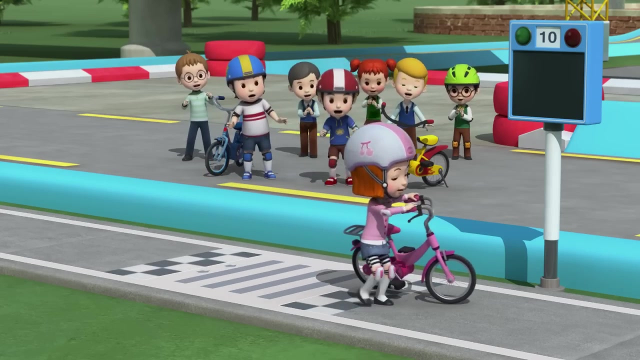 this points off, points off, Kevin. you fail. there's no way I could have failed. please get ready. excuse me, oh, Jenny. hold on, you don't even know how to ride. you're going to look like a fool. now here goes all right. a crosswalk means I should walk with my bike, congratulations. 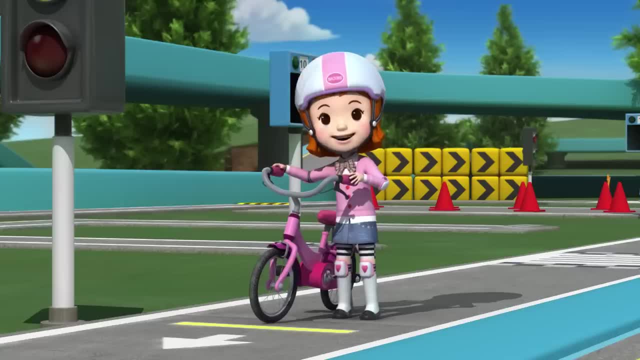 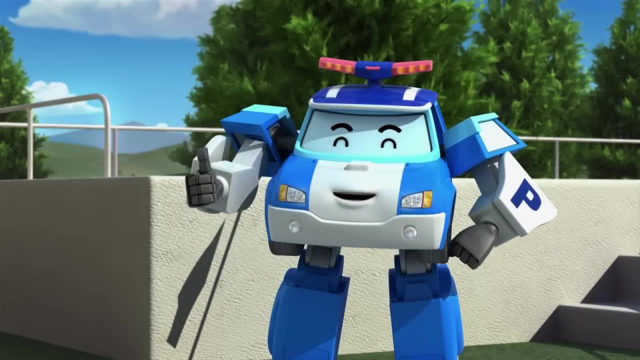 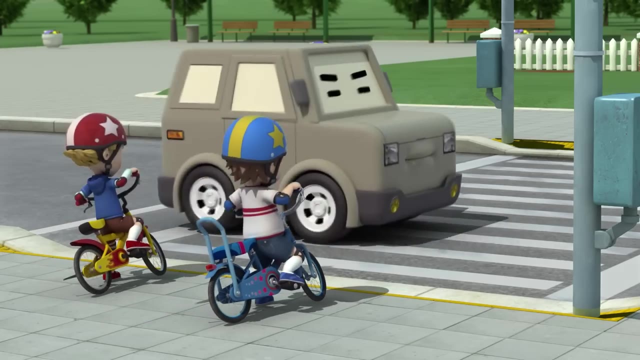 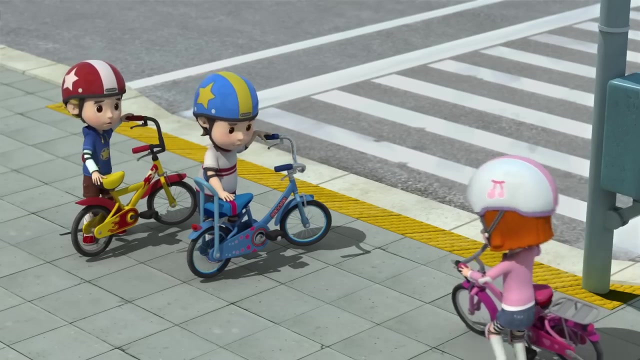 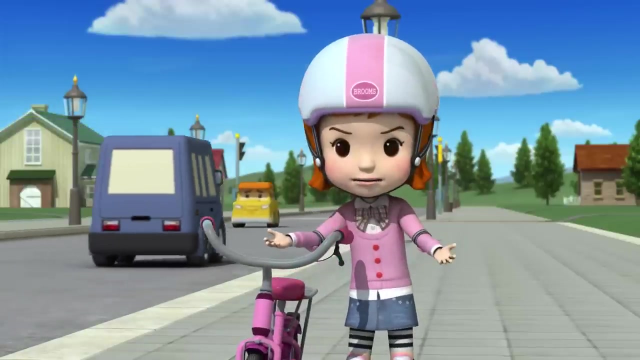 entrance number 10. Jenny, you passed the test. hey, don't you remember what I said: get off and walk when you cross the street. Jenny. rule number one: safety first at all times. that's right. you're the ones who failed the test, remember? you two should be extra careful. all right, we've heard it a million times before. 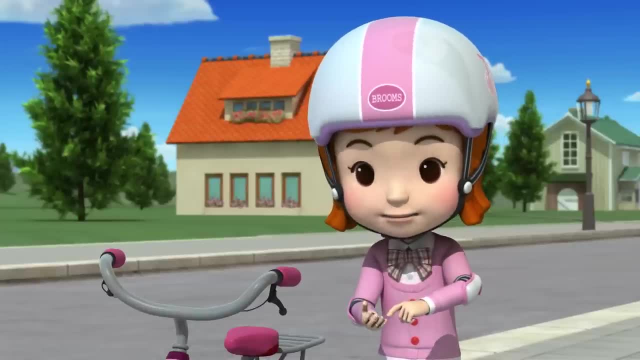 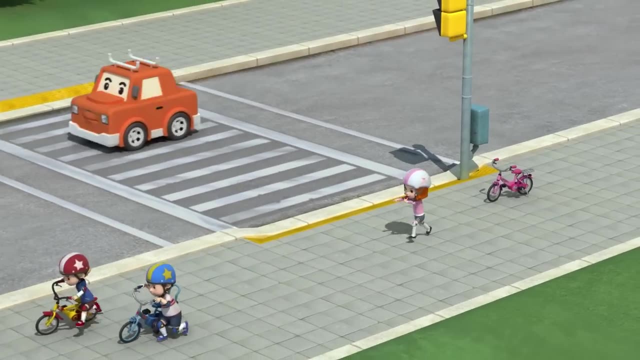 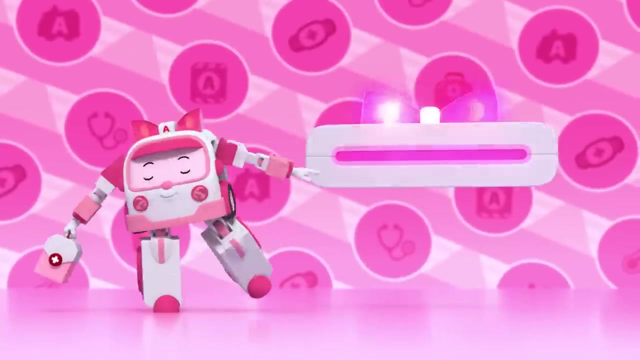 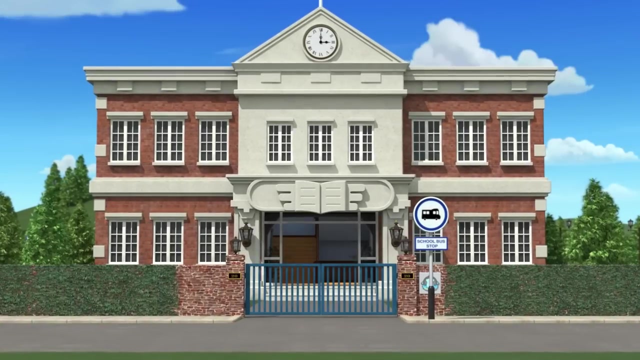 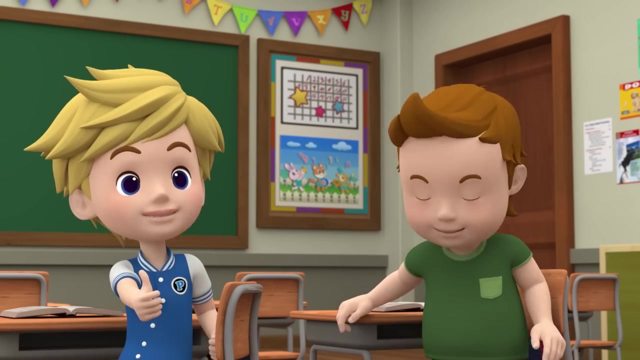 listen, did you check your bicycles, Kevin? your seat looks like it's too high. stop, see you later, stuck in the elevator. how should I know where camels live? camels live in the desert- you're so smart- and gators, they're in the swamp. oh, this is the last one, do you? 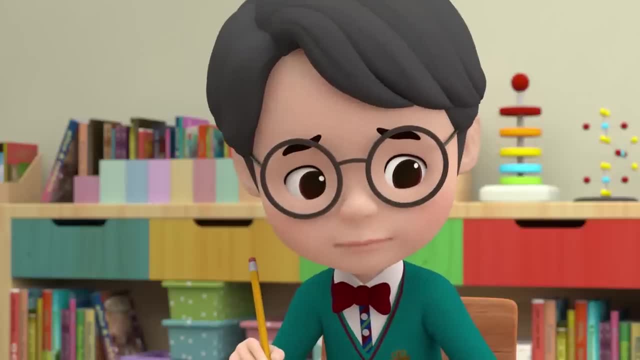 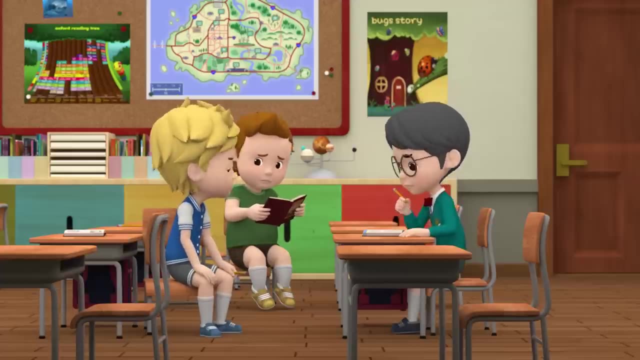 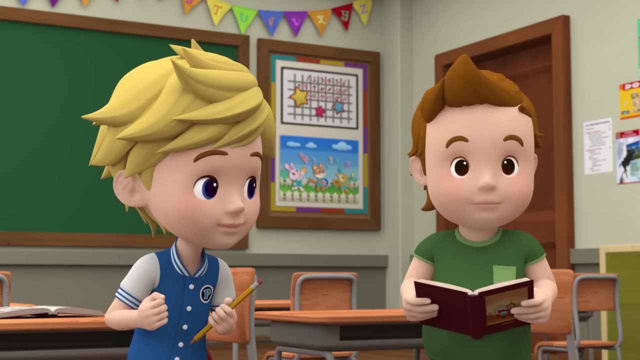 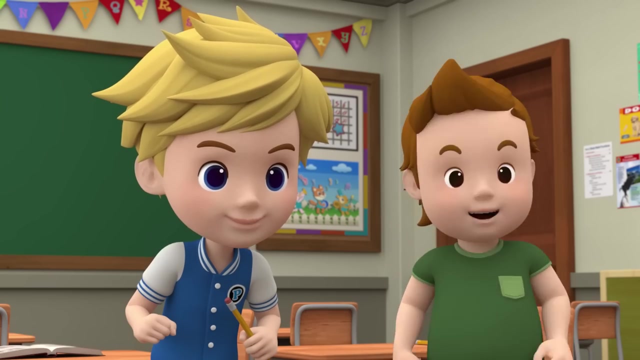 know where gorillas live. oh, I think that I forgot that one. what really? hmm, and I still have one left. so what? now I got it? we can search the internet. we can use the computer at my house computer. come on, let's go play video games lots more. I hope nobody has a lunch of each other. 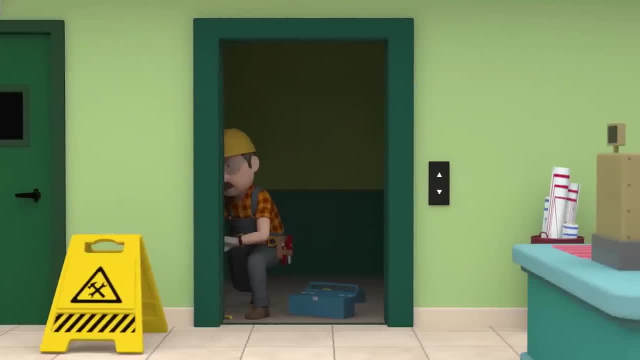 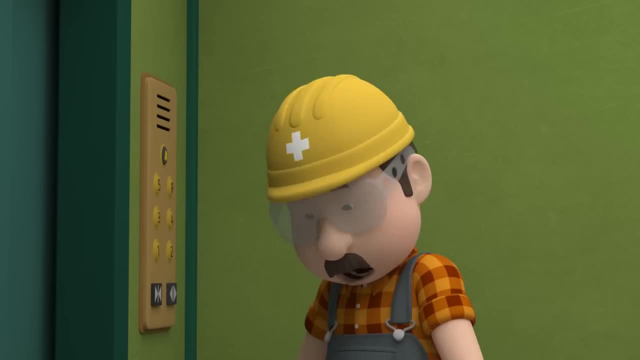 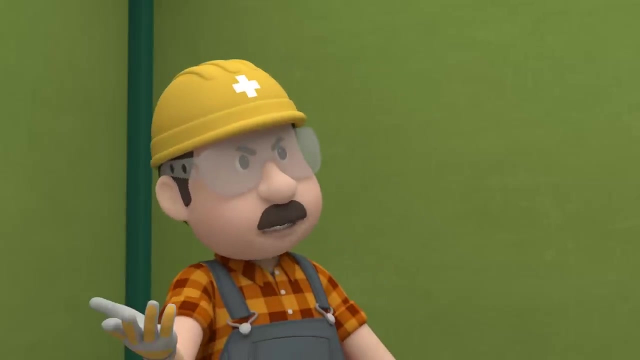 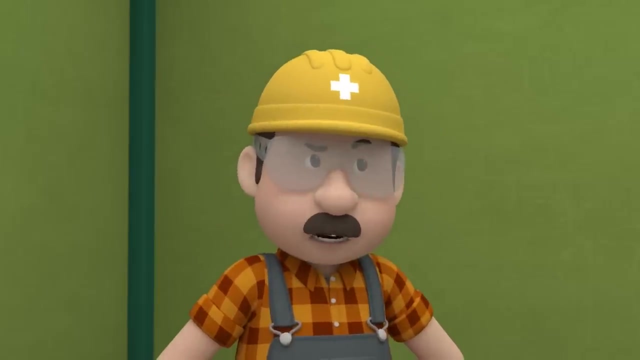 oh yeah, we're all in the same little bunch. so whose kid is good at playing computer? yeah, I mean, do this research project, let's go do it. what? hmm, huh, looks like we're back in business. 이�wno, The elevator's frequently out of order. 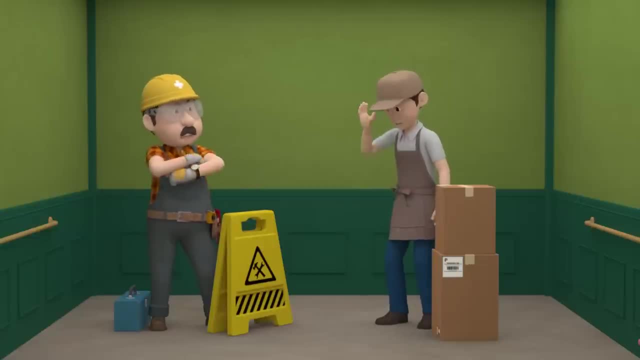 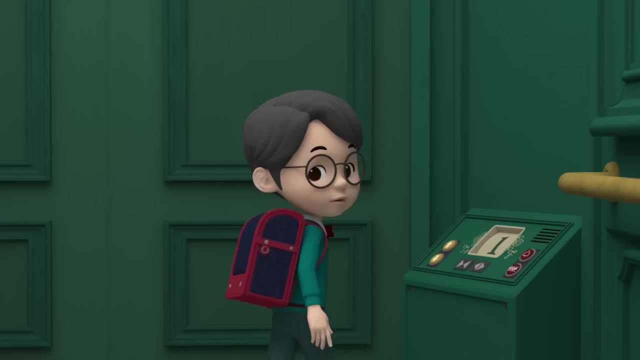 It's because of carelessness. I'm so sorry. I won't do that anymore, Charles. what kind of games have you downloaded? Peter, we're here for homework, not games. Let's play for a little bit and then do homework. 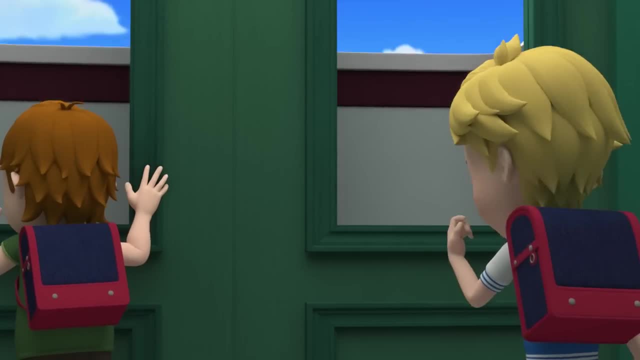 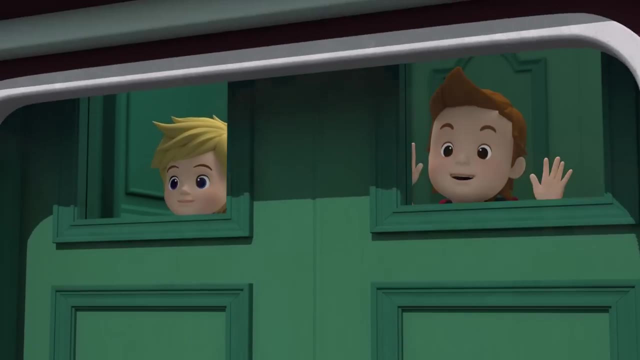 Peter, check this out, Johnny. it's just an elevator. It's like it's your first time. Whoa, look at that awesome view. Look right there We can see City Hall. I see it. Hey, you guys, you're not supposed to lean on there. 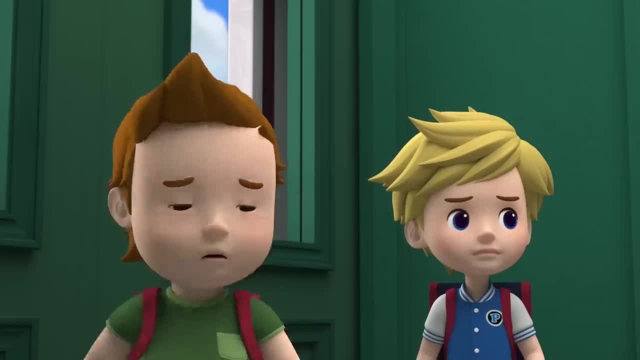 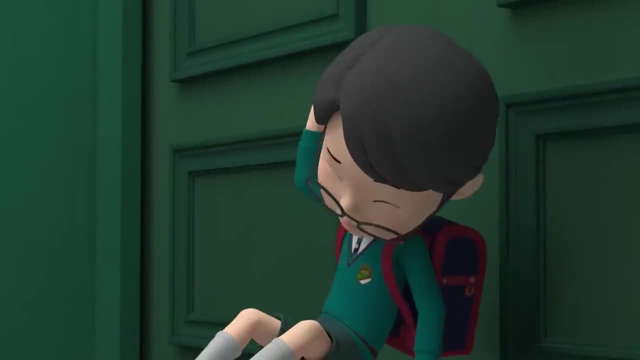 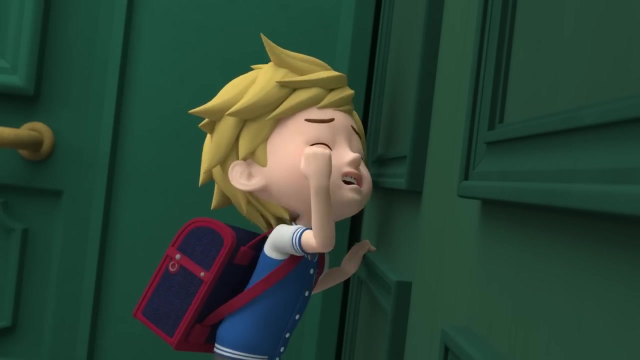 Are we there already? Not yet. What happened? Do you think that it's broken? Hey, you guys, you all right. So how do we get out of here? I have an idea. Somebody help. we're stuck inside here. 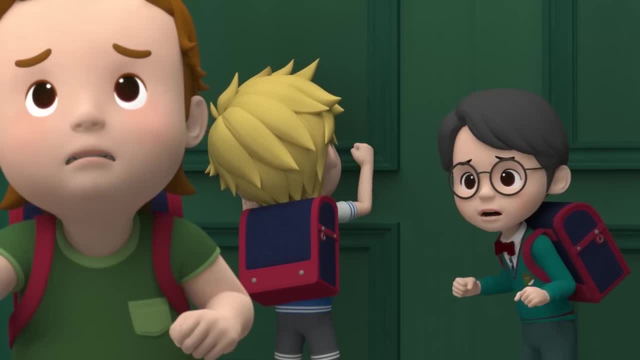 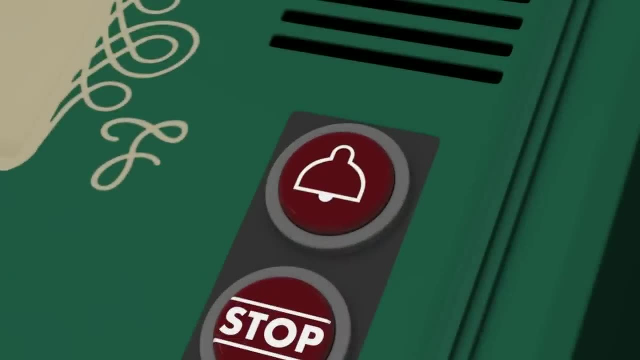 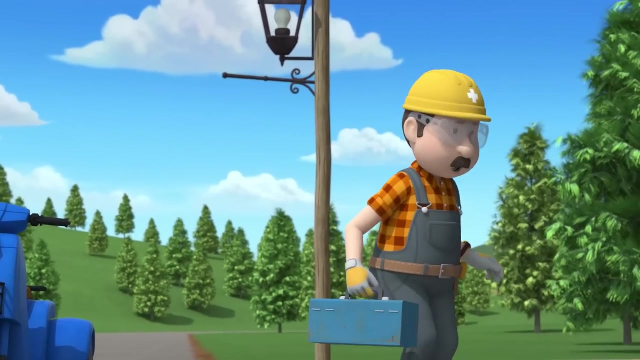 Anyone? can you hear us? Try to calm down. We don't want it to fall any farther. Then how do we get out The emergency button? I'll just check in here and then I'll be finished. Can anyone hear me? 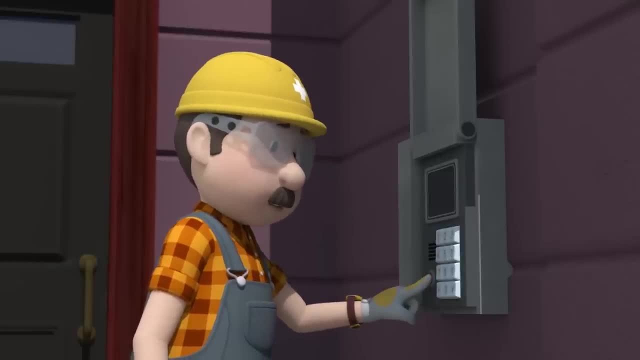 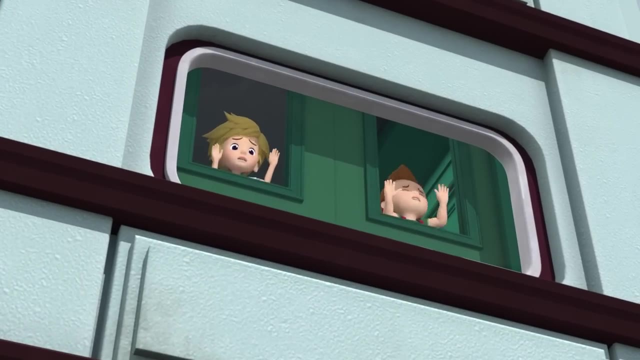 Huh, What's the matter? The elevator stopped suddenly and we're stuck in here. I'm coming, Get us out. Oh my goodness, Come in, rescue team. I need you all at Broom's Villa right now, Right away. 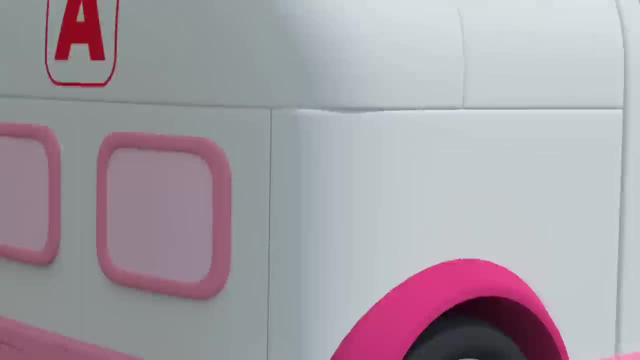 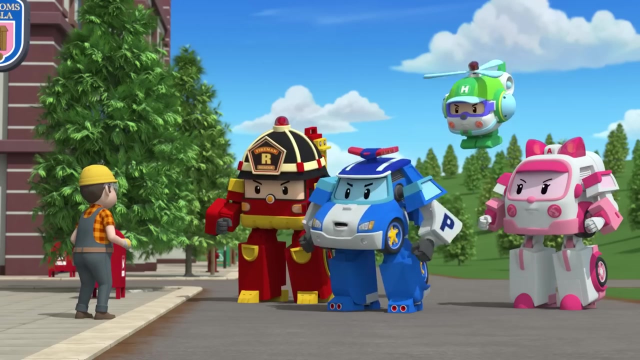 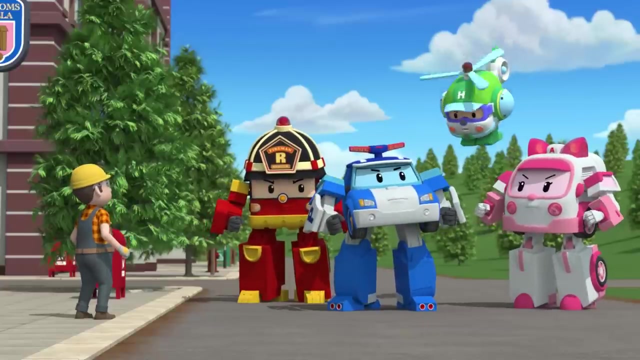 There's been an accident. All right, Right here, right here, Don't worry, Mr Builder, we'll get them out. Roy and I will go to the roof to get the children. Heli, can you install the loop to hang the rope? 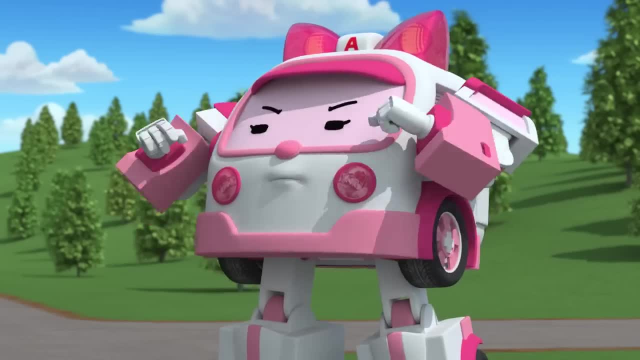 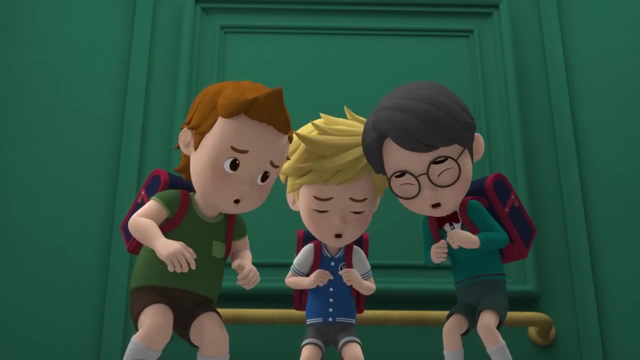 Of course, Amber. can you make sure the kids stay calm? Sure, Polly, Hey guys, are you there? Amber, Ah, Please get us out. We want to go. We might start to fall again. Don't worry, The rescue team is here. 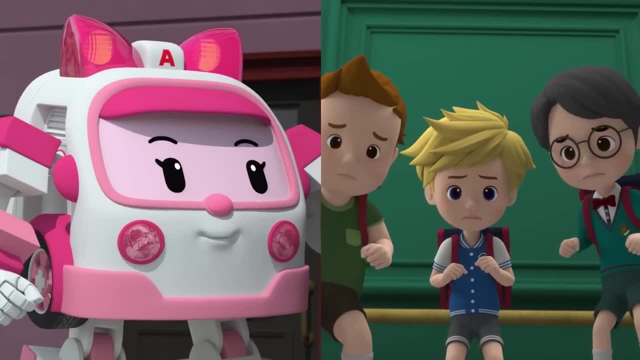 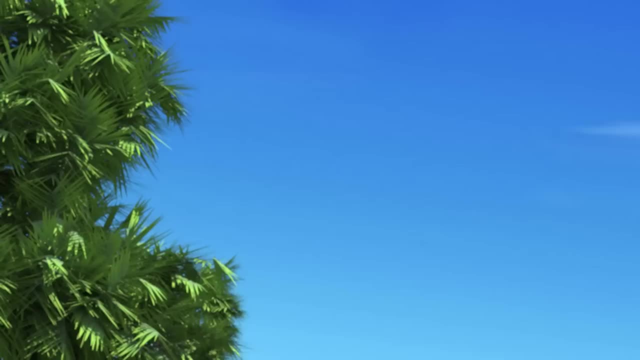 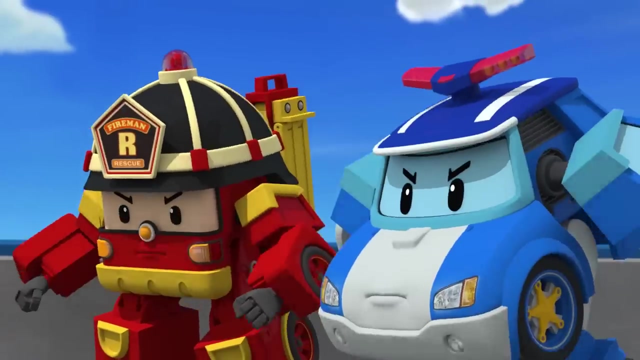 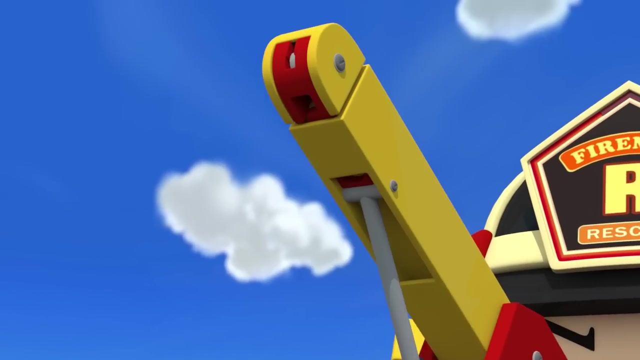 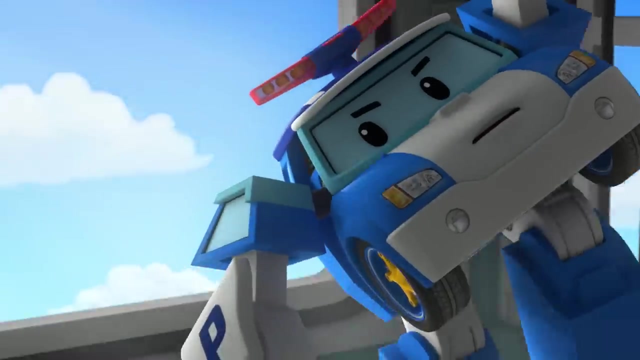 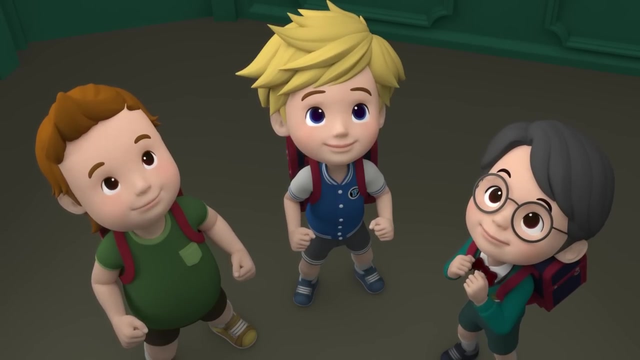 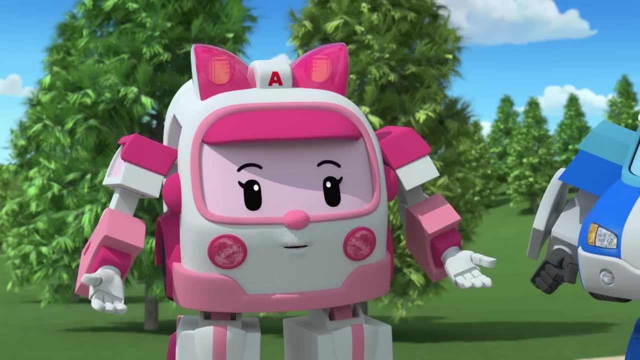 We just need you to stay calm. Okay, we'll try, Polly, you're all set. Go, Roy, Right, Roy, prepare the crane Right, Find the onto the roof. Yes, Are you guys? all right, Polly? 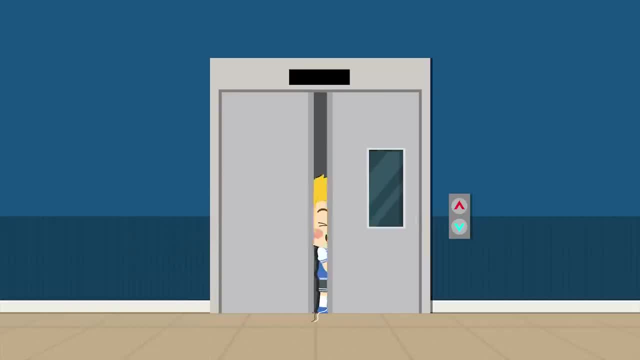 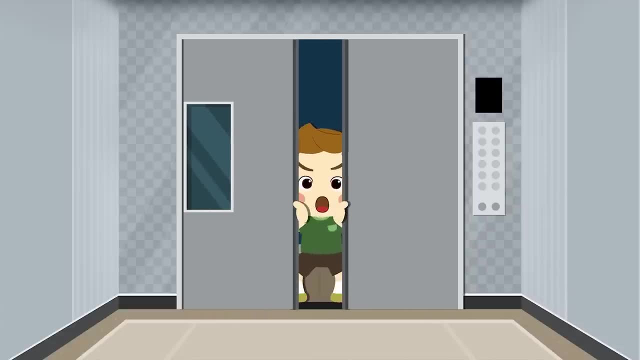 We're so glad you're all safe. Thank you for saving us. Ah, When riding in an elevator, be sure that your shoelaces and clothing don't get caught in the doors. Don't hold the doors to keep them from closing. 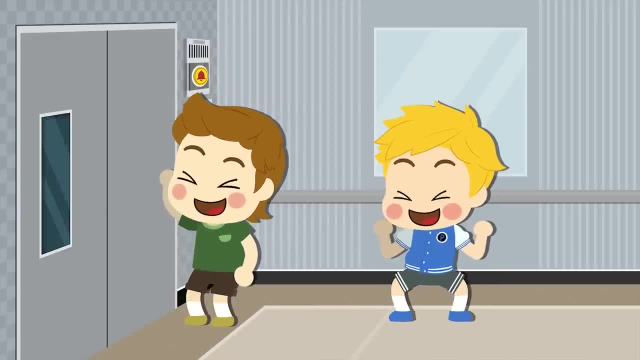 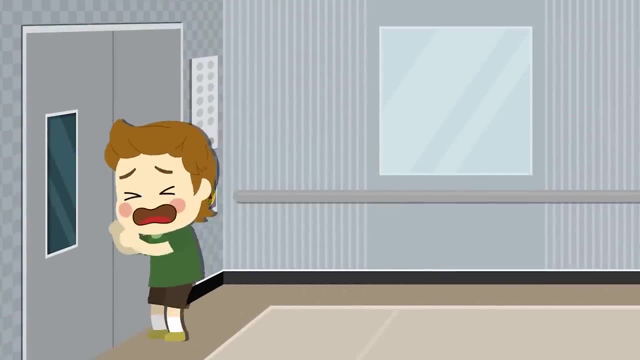 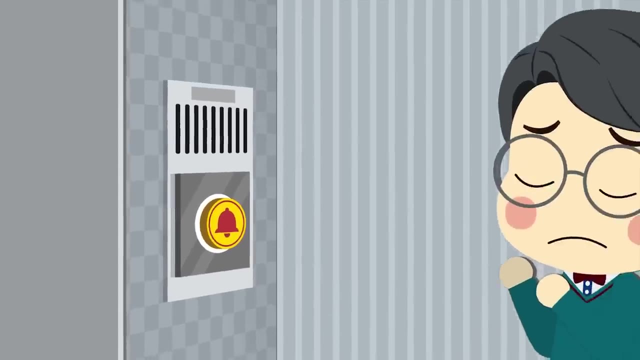 Don't ever jump up and down in an elevator or pound on the doors, or the elevator may stop. If the elevator does stop, don't ever try to force the doors open or you could risk falling. The best thing to do is to remain calm, press the emergency button and wait for help to arrive. 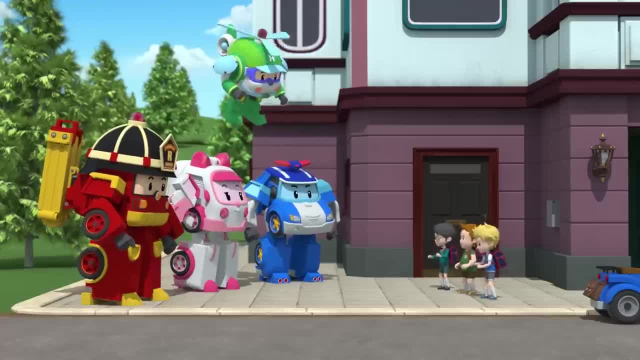 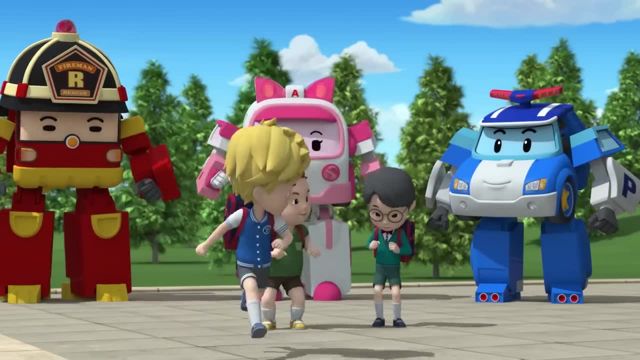 That's easy, right? Yep, We got it, Amber, All set. The elevator should be good to go now. It's all fixed, Charles, let's go play video games. Come on, Charles, Hold on, We're supposed to do our homework. 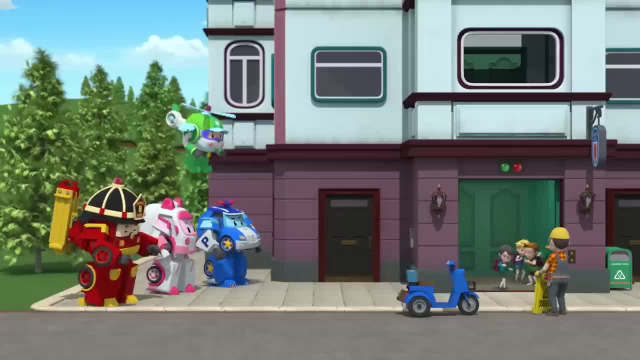 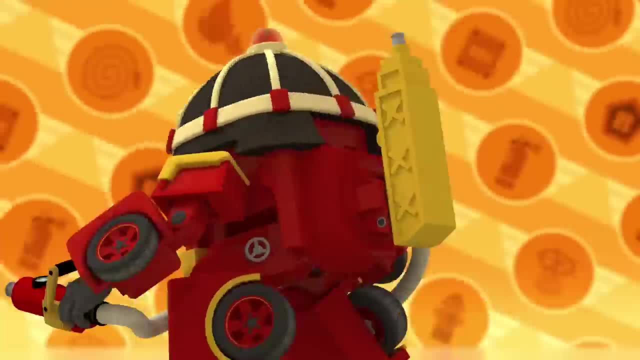 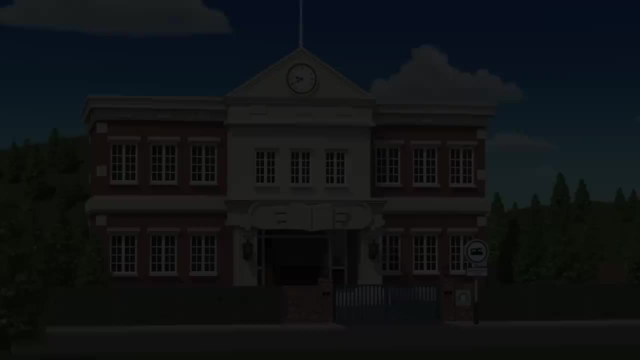 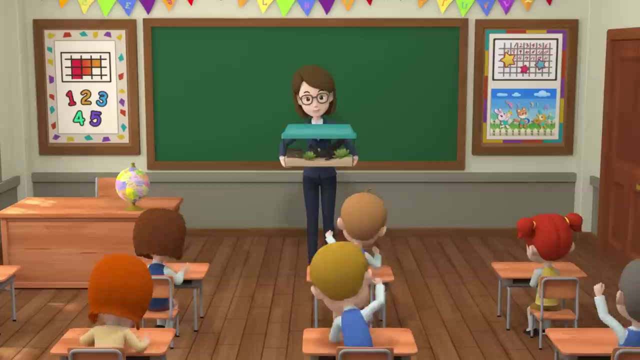 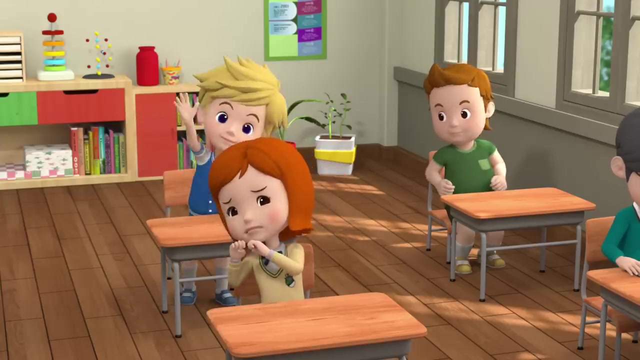 Hey, you kids Don't run in the elevator, remember? Oh yeah, that's right. The School Fire Drill Everyone. we have a new friend today, Whoa. Someone needs to be in charge of feeding him. Pick me, I can do it, Pick me. 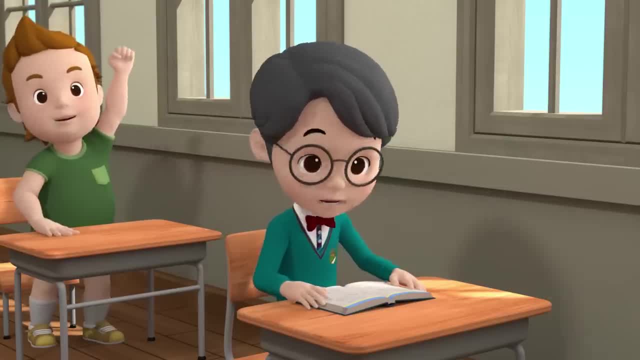 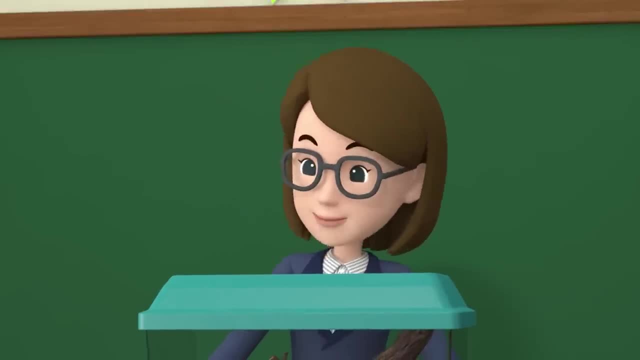 Um, Oh, Charles, I'd like to take care of him this week, Me Really, ma'am, Mm-hmm, Since I know you love animals, I'm sure you'll do a good job with our class pet. Are you up to it? 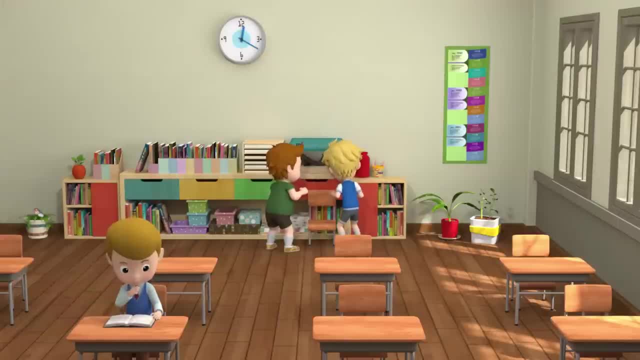 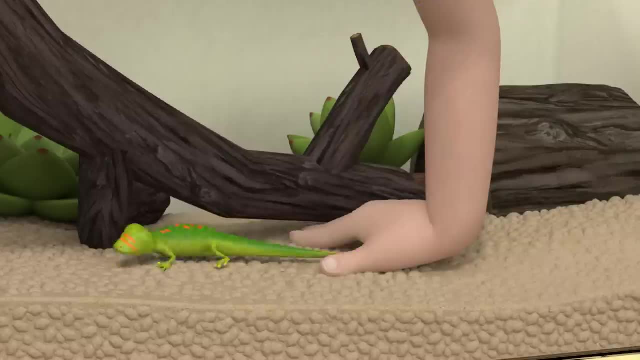 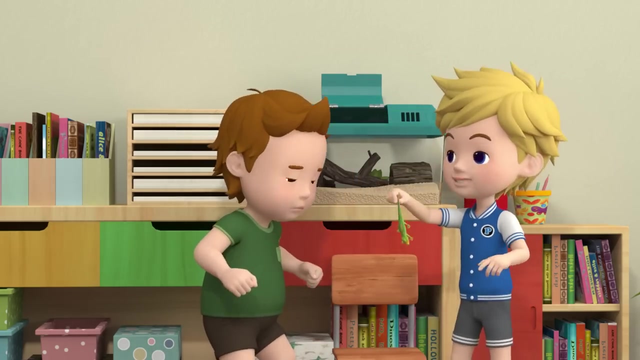 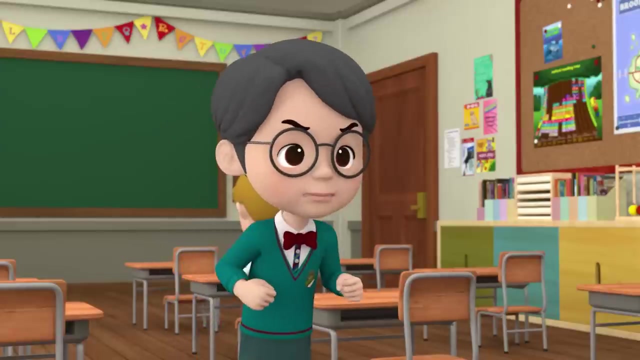 You bet I am Whoa. Why can't you stay? still, I got him Whoa. Come on, let me hold him Me first. Hey, stop it. Huh, You're being cruel to him What We're not being cruel. 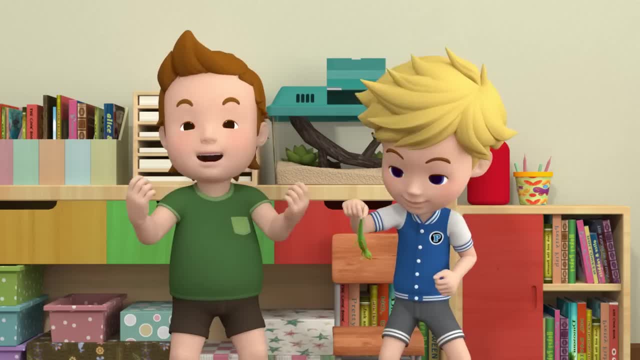 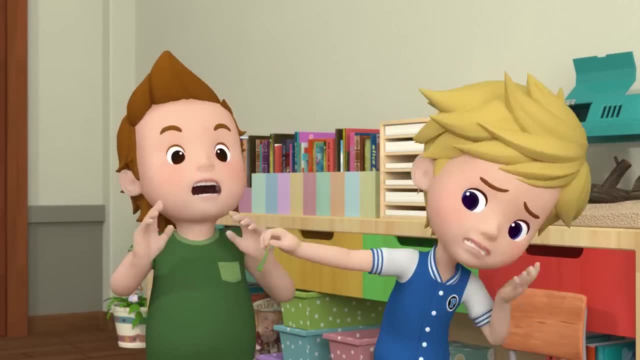 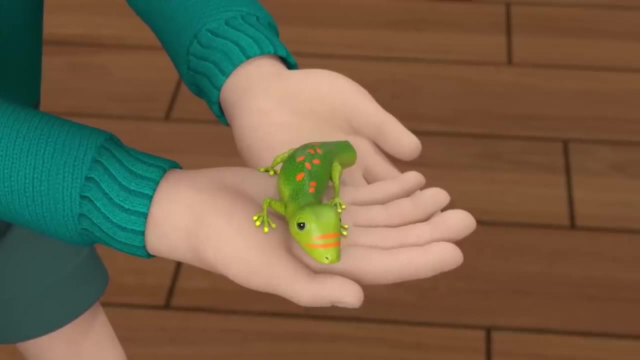 I just wanted to play with him, that's all. That's right. Come here and give it a try. No, I broke his tail. Some lizard and gecko species drop their tails when they feel they're being threatened. Oh man. 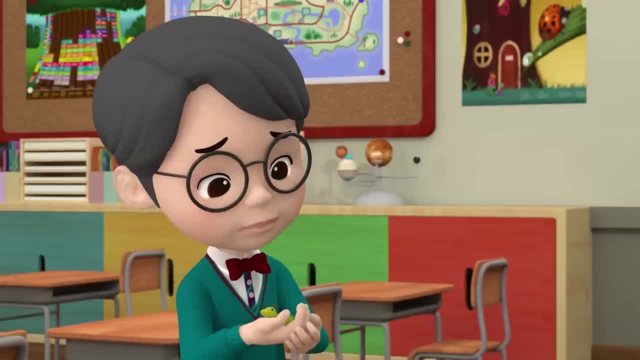 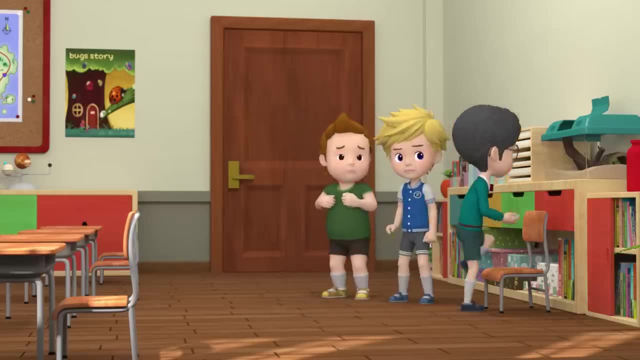 That's gross. Listen. their tails hold valuable nutrition, so losing them can be really bad. I'm taking him home to keep him safe and you can't touch him anymore. Okay, I'm sorry, little guy, It'll grow back soon. 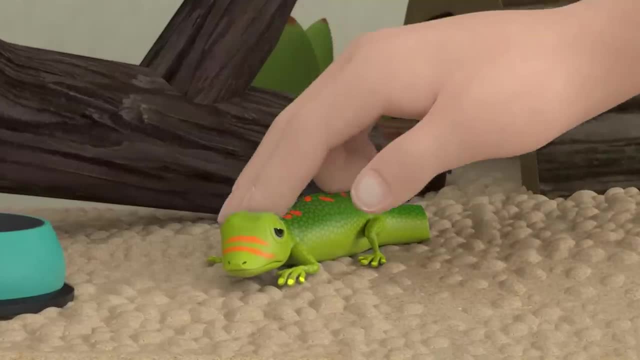 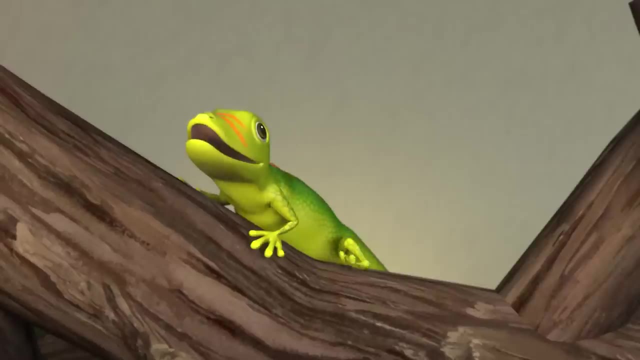 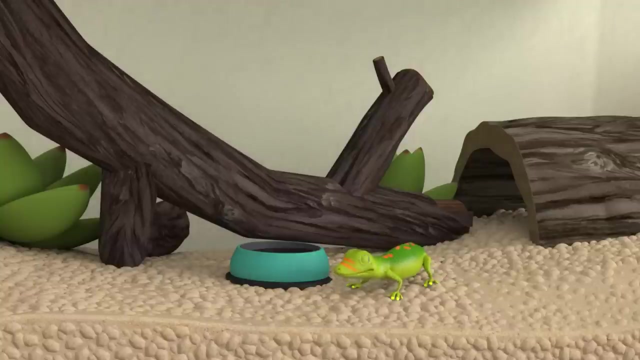 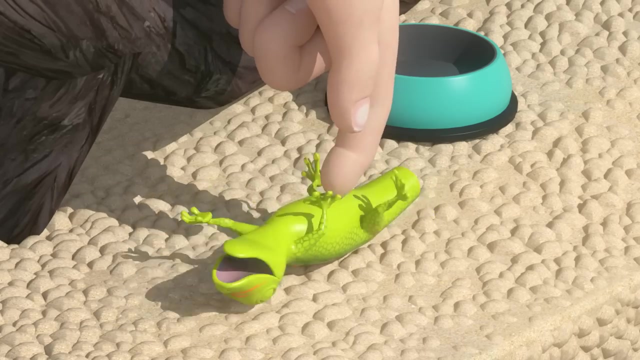 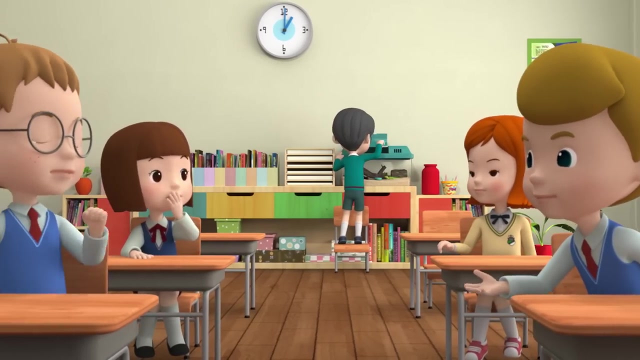 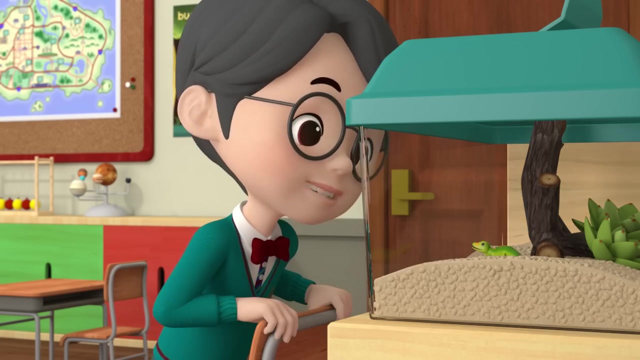 You need a name, huh, From now on, I think I'll call you Finn. Haha, Is that better, Finn, Eat up. okay, We should play dodgeball. Yeah, That good, I see your tail grew back. That's great. 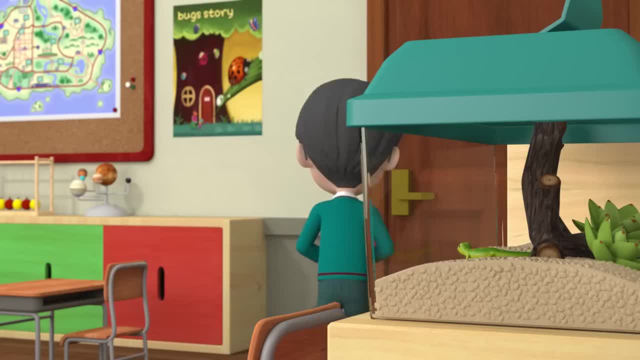 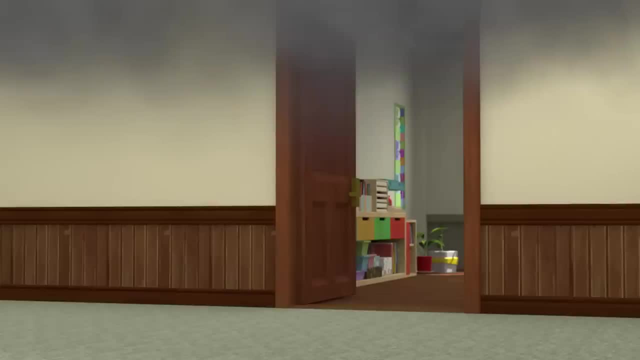 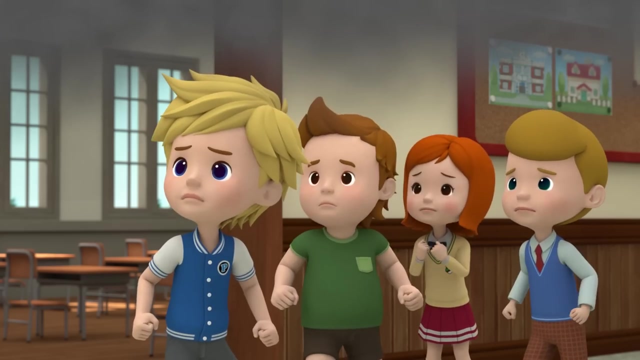 Oh, your water's empty, I'll get you some more. Huh, What's this Fire? Fire. I didn't do it this time. It wasn't us, Everyone this way. What's happening? There's a fire downstairs. Single-file line and follow me. 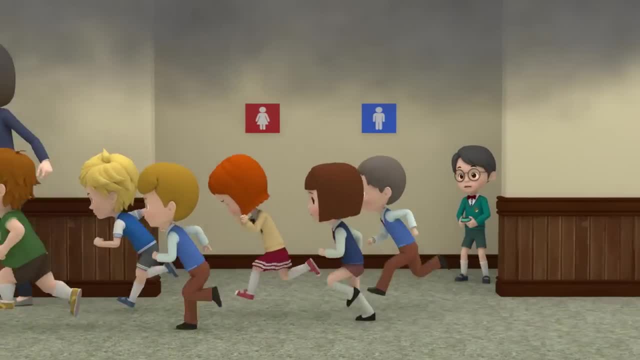 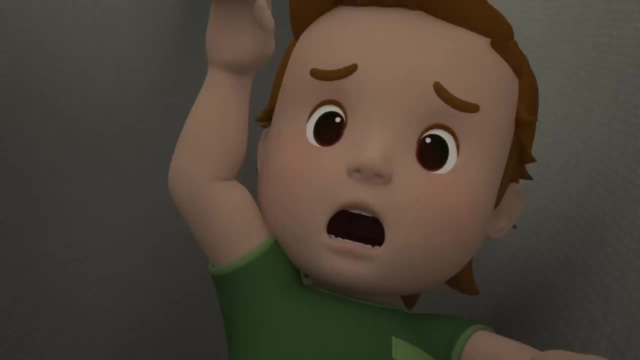 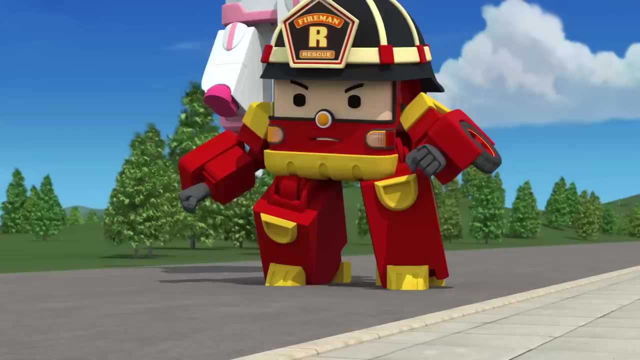 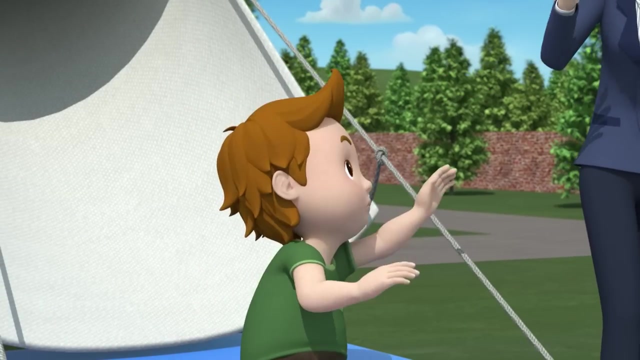 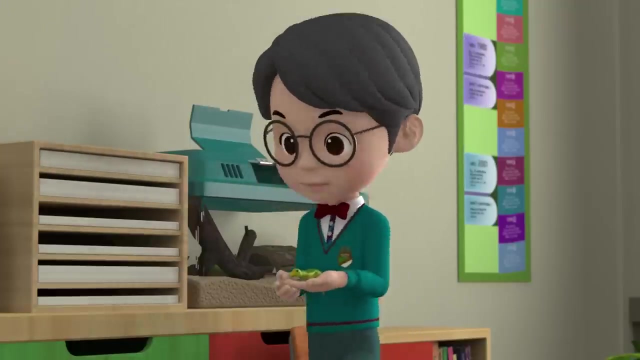 Right, Huh, But Finn, Whoa, Everyone all right. Yes, I think we've got all the students outside. Wait, Hang on, Charles isn't here. What, Charles? Hey, Finn, Now we can go, But we can't go that way. 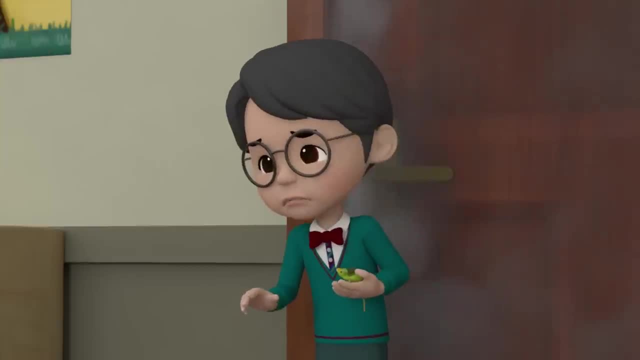 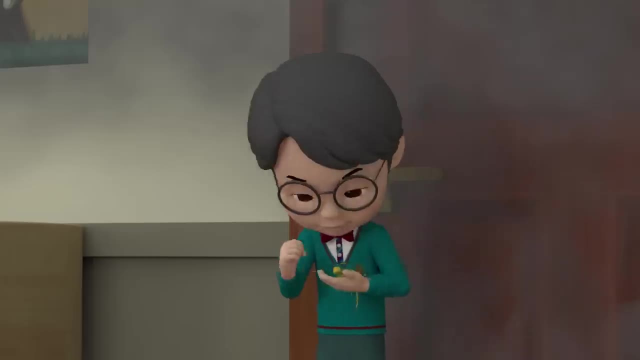 This is bad, huh, Don't worry, We'll make it out of here Over here. Look, I can't get out. It's Charles, He's in the classroom. Charles, Charles, Charles, Huh, Roy, he's in their classroom. 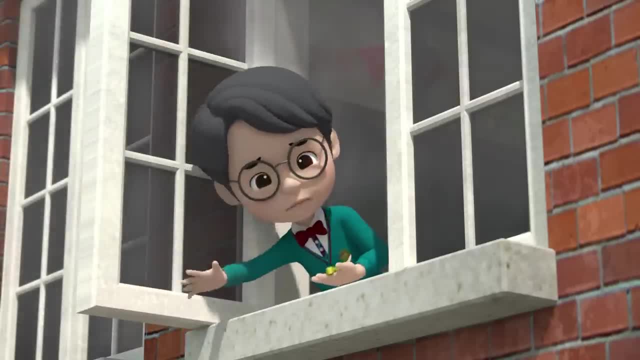 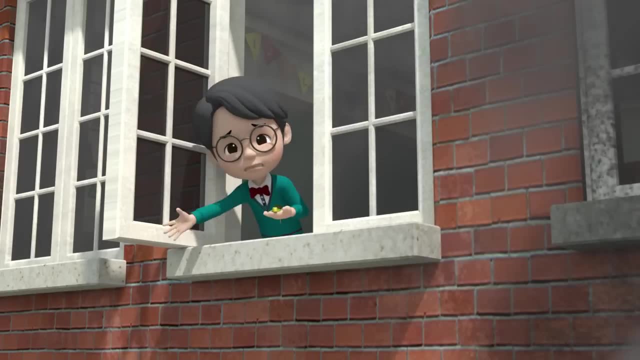 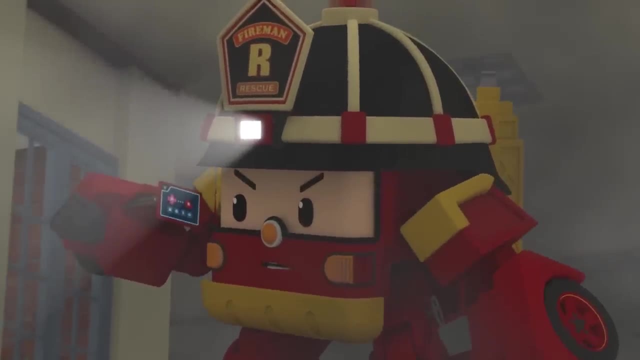 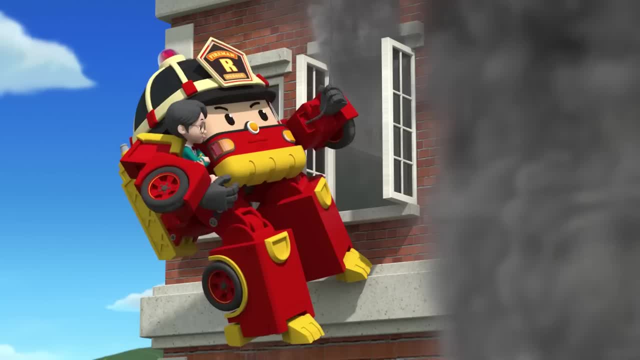 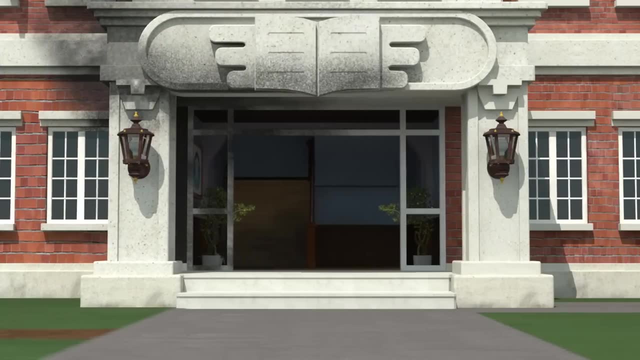 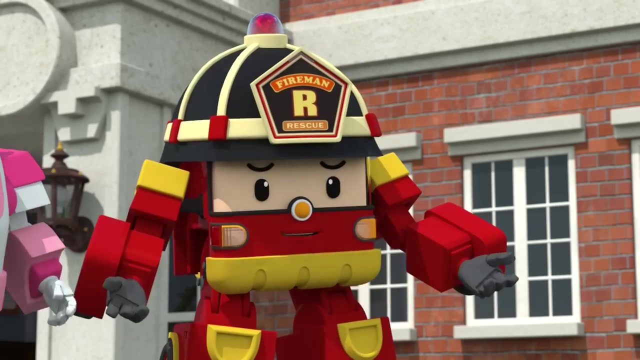 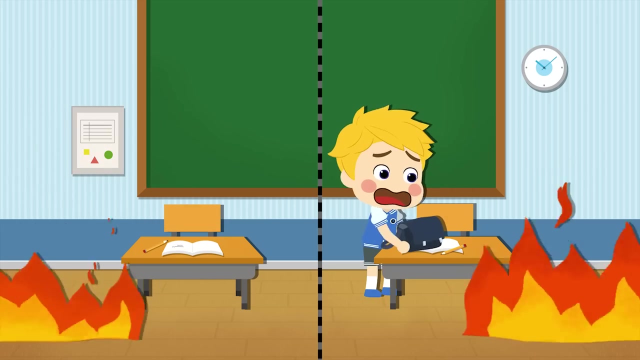 I'm here, Roy. Okay, You ready? Yes, Here we go. The fire's all put out now. Thank goodness no one was hurt, Roy. thanks for saving me today, Charles. what you did was incredibly dangerous. When a fire breaks out, you must leave all your belongings and get out as fast as possible, no matter how important it might be. 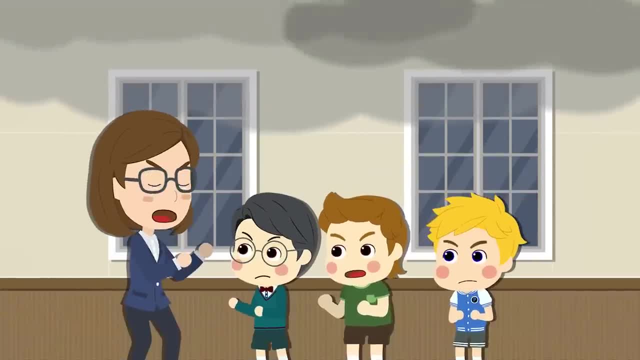 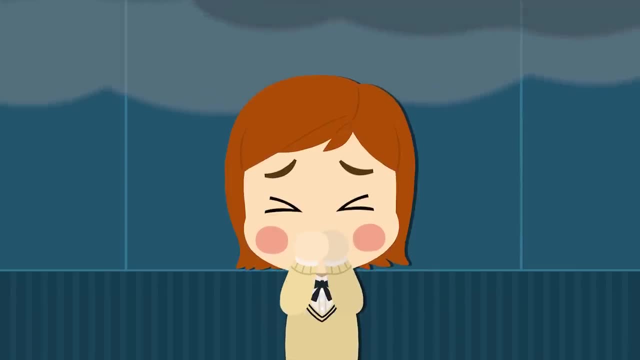 Don't run off by yourself. Listen to your teacher and follow their instructions till you get to a safe place. Hit the fire alarm if you're the first one to see it. Cover your nose and mouth from smoke, duck down and leave quickly. 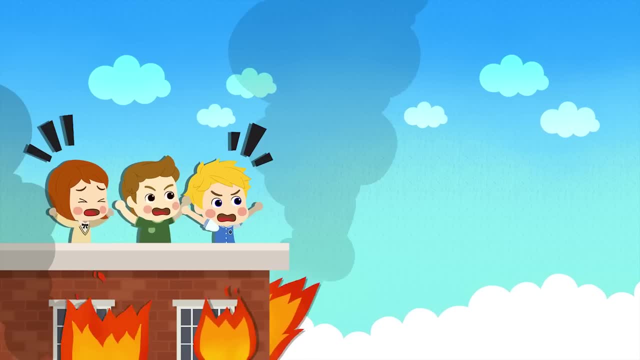 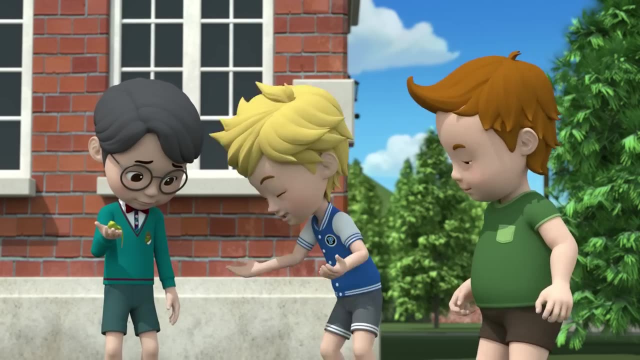 If the fire gets so bad you can't escape, run to the roof and yell for help. Got it, Roy, I'll remember. Sorry for making you guys scared, That's all right. Since you did that, you saved our class pet's life. 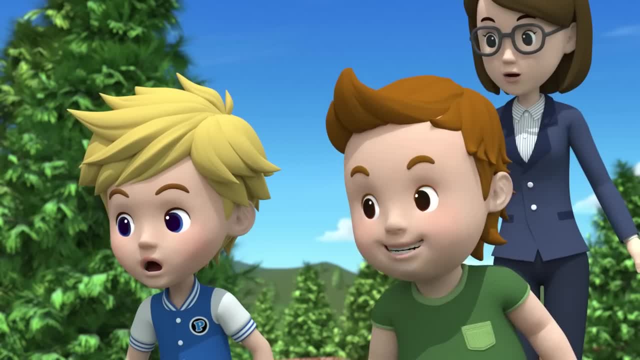 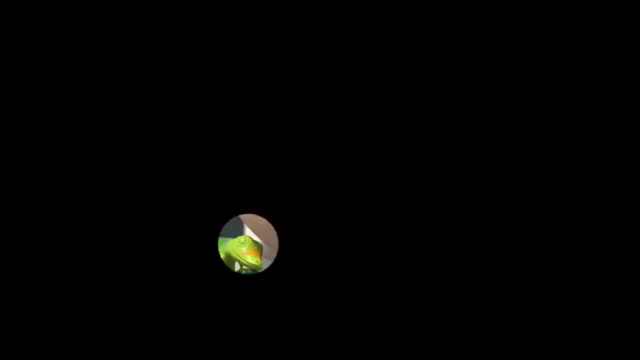 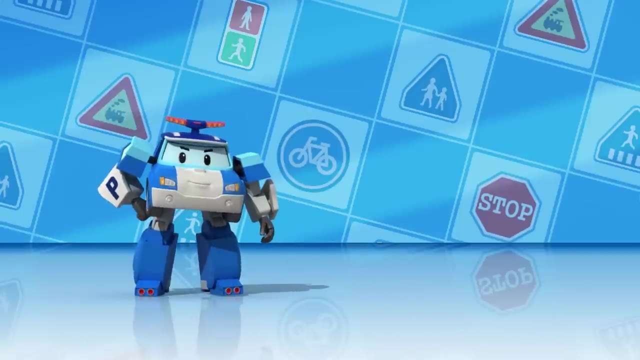 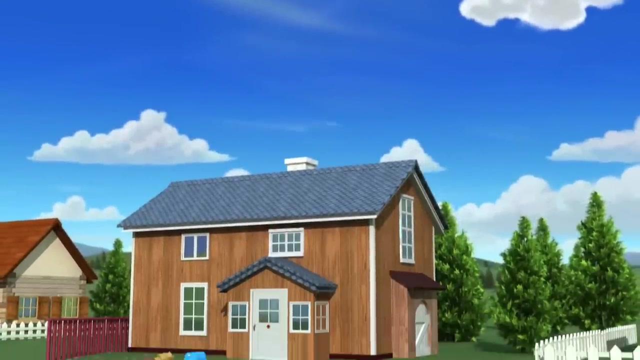 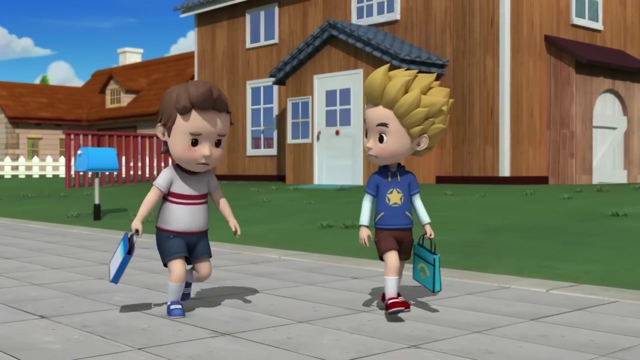 Yeah, you saved him. Hey, Finn's trying to say thank you. The tickle, The tickle. Ah, I really don't like homework. Yeah well, I'm so hungry, Doug, why don't we go play for a little while? 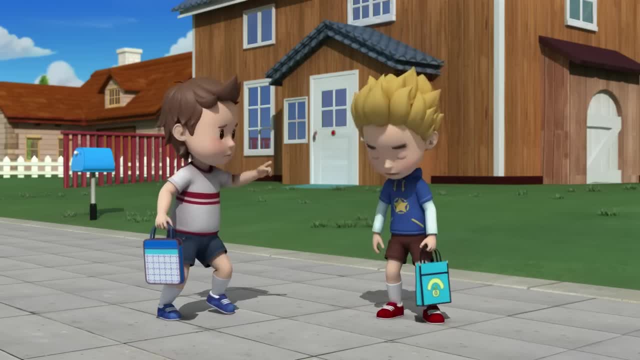 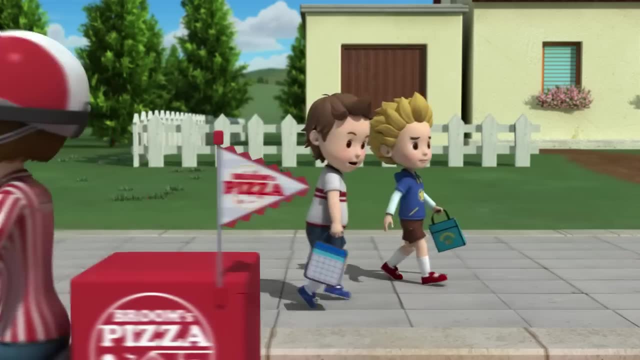 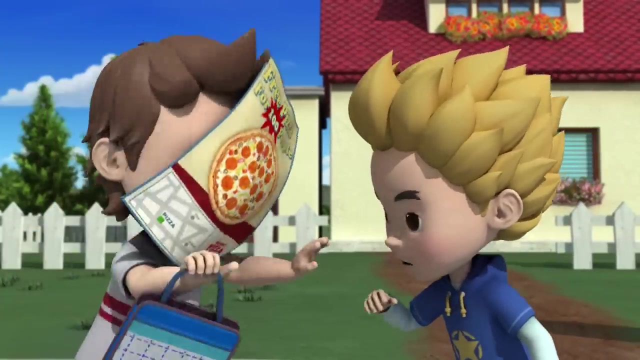 We can't. If we're late, Jenny will be mad. Yeah, you're right about that. Oh wow, Pizza Pizza. The first 100 customers get free pizza today. What Free pizza? Yeah, Let's go get some. 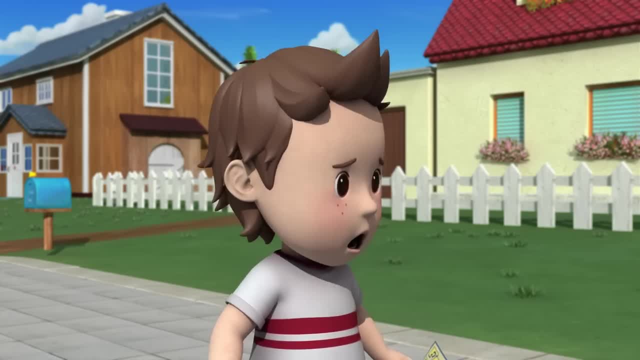 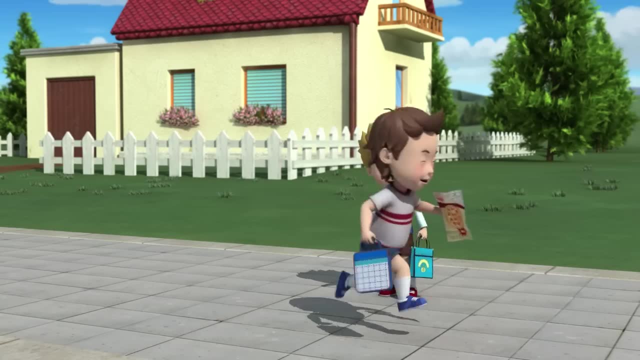 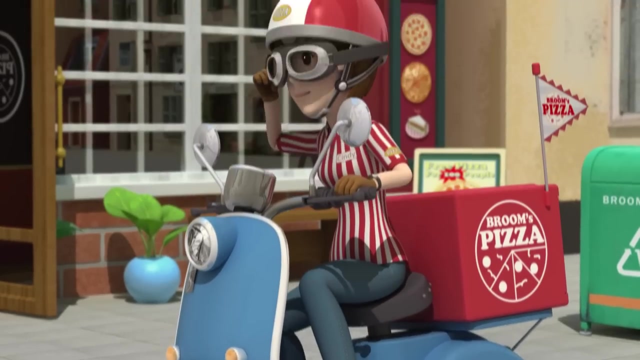 Uh, hang on, But Jenny's still waiting for us. If we bring her some pizza, I bet she won't mind so much, right? You think so, Of course. Ha, ha, ha, Phew, Excuse me, Excuse me, please, Pardon me, sir. 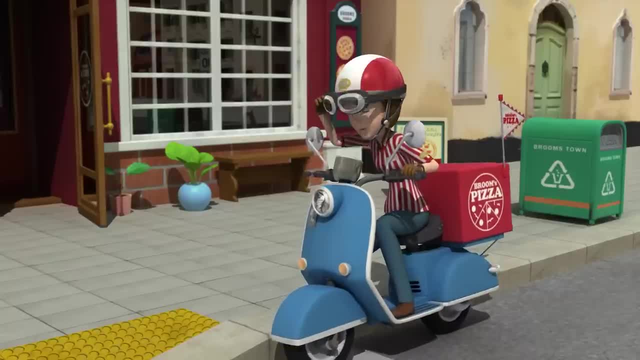 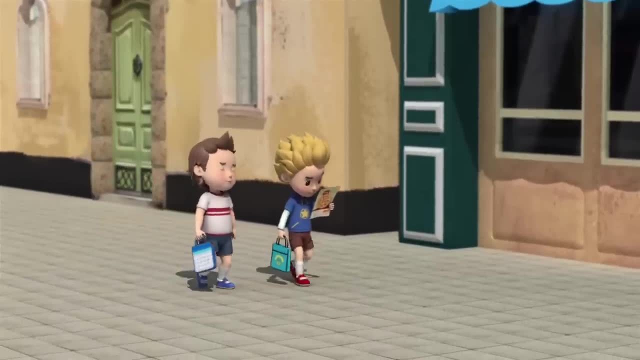 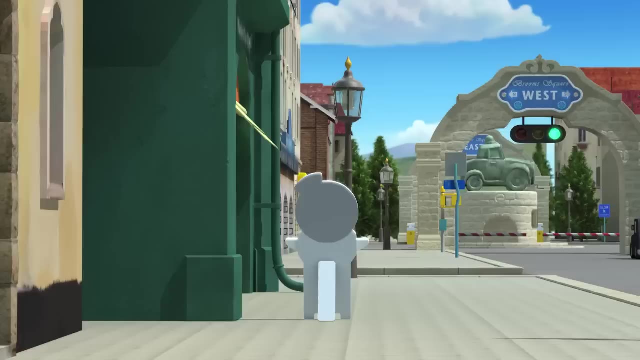 Wow, There's no time to rest today. Okay, Pizza's on the way. Kevin, are we almost there? Yeah, We should be just about there. Let's see, I think it's right around here. We found it Time to eat. 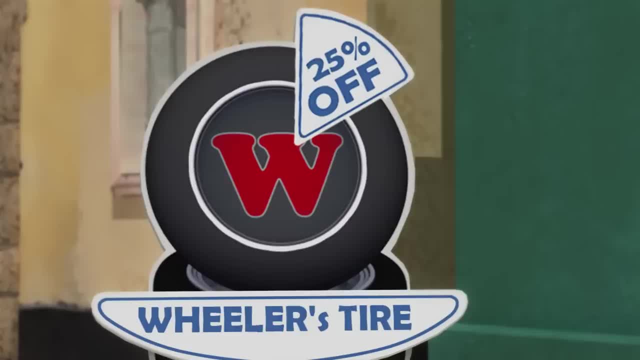 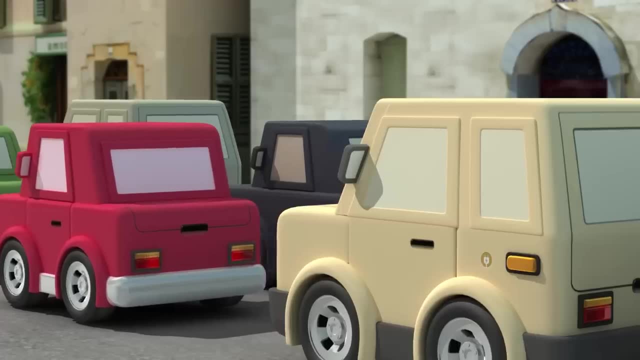 Ha, ha ha. Huh. This is not the right place. We got tricked by that sign. Wow, Traffic is so bad. Well, in that case there. Okay, This is 7th Street, Sorry, Huh. 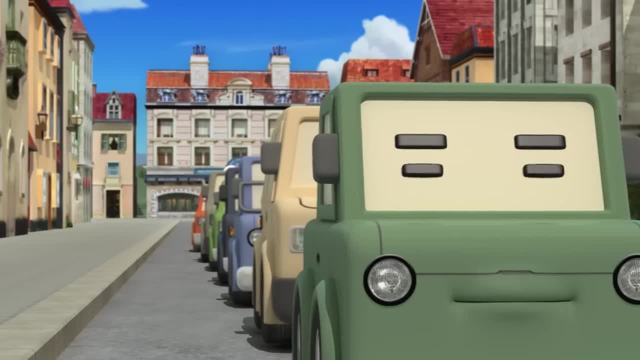 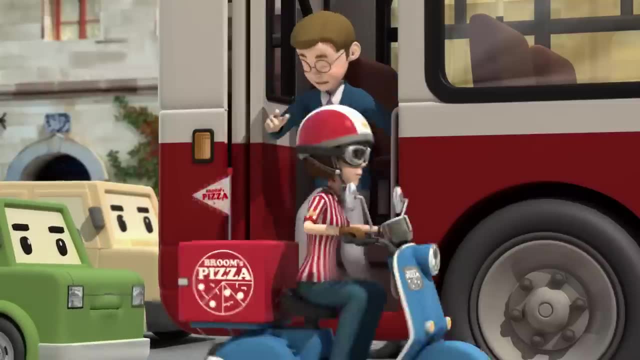 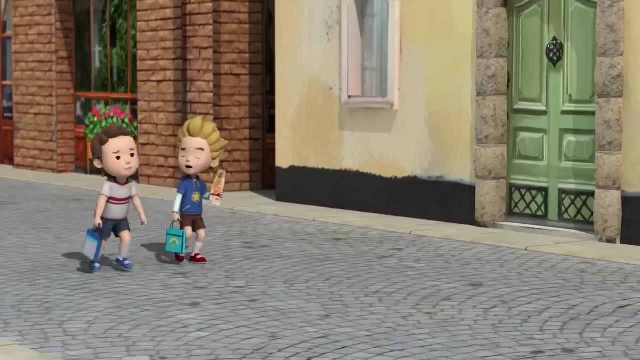 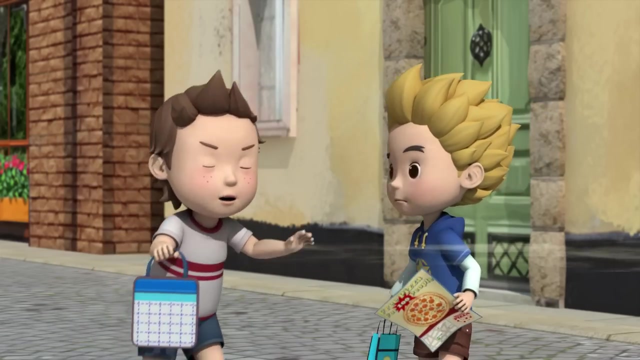 Sorry, Sorry, Sorry, Sorry, Sorry, Sorry, Huh, Uh, Uh. So I'm pretty sure we're just about there. Um Huh, Hold on, Huh, I can smell it, Kevin, I can smell it. 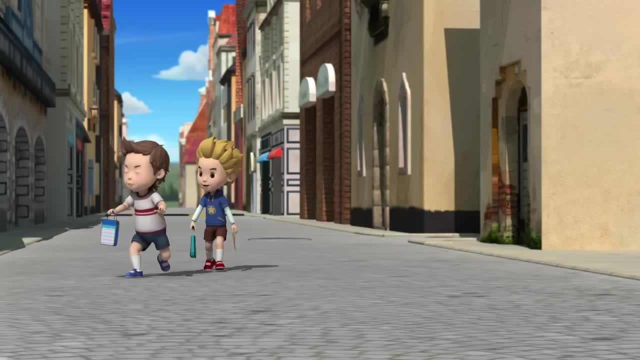 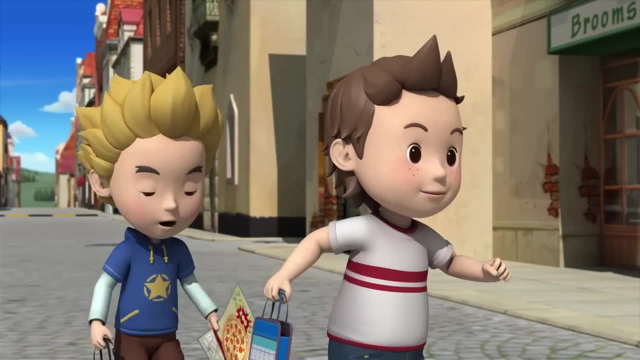 You go. Doug Your nose is never wrong. Ha ha ha, My nose says that we're getting close. Oh, Oh, Huh, I found it. That's awesome. Where is it Where? I'll take a hot dog, sir. 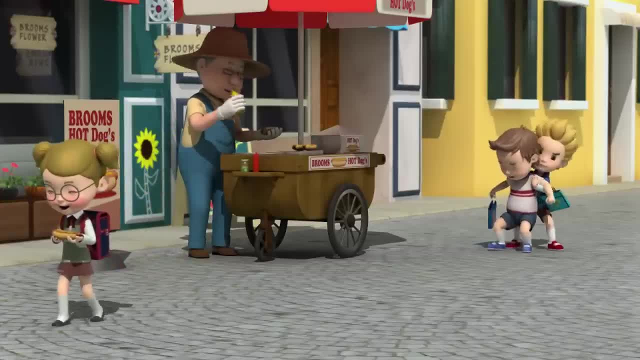 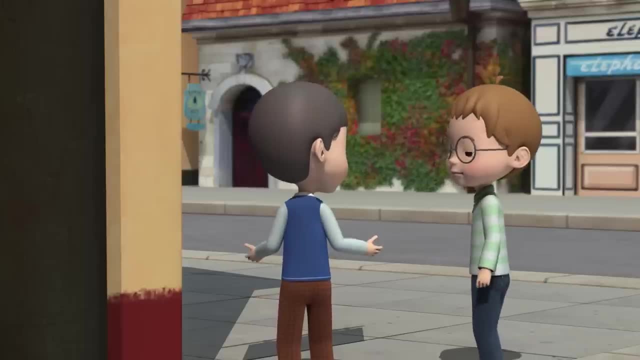 Awesome, Get moving, Doug. We're going to miss out on the free pizza. Hot dog, come back. I think we're almost there. Are they really giving away free pizza today? That's what I heard. Huh, All right. 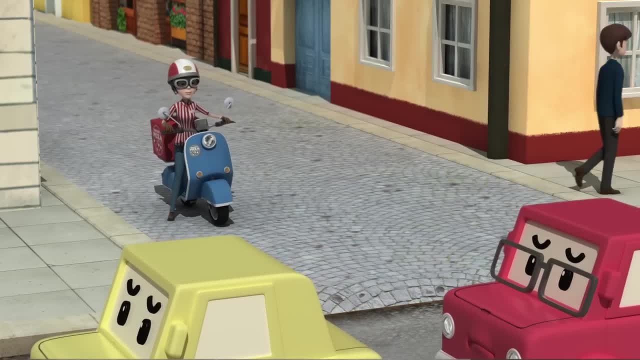 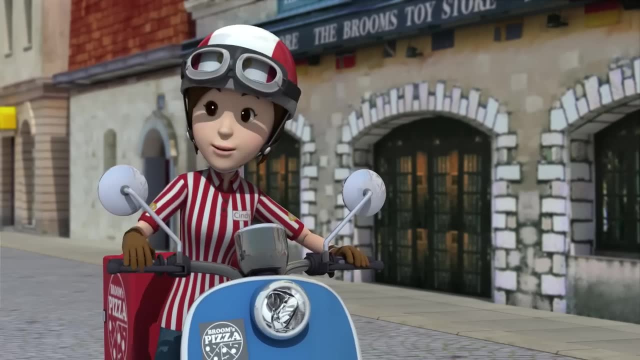 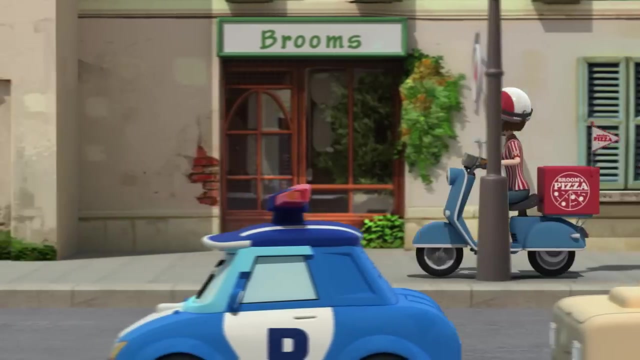 This way. Come on, Let's go. Ha ha Phew. I've just got one more pizza to go. Should be around here somewhere There. Huh, Why is that scooter on the sidewalk? Try to run faster, We're almost there. 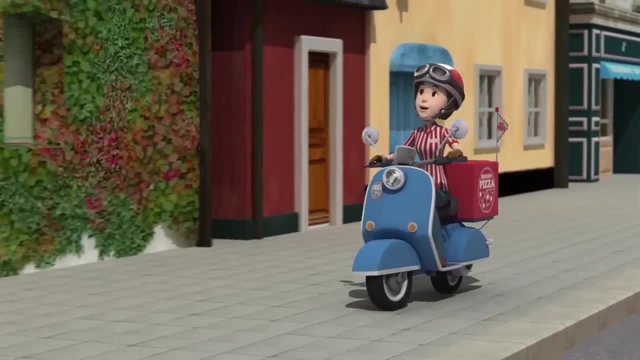 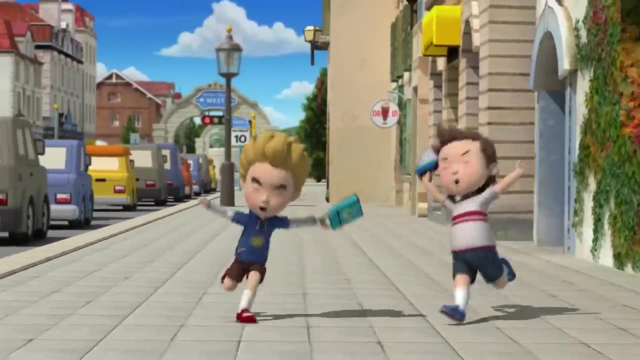 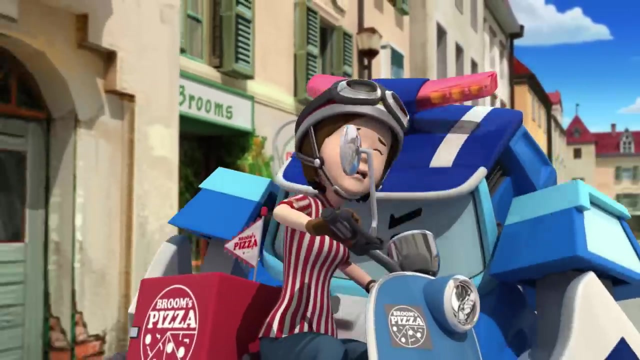 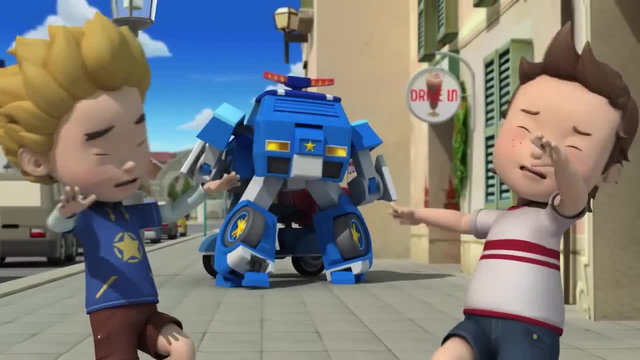 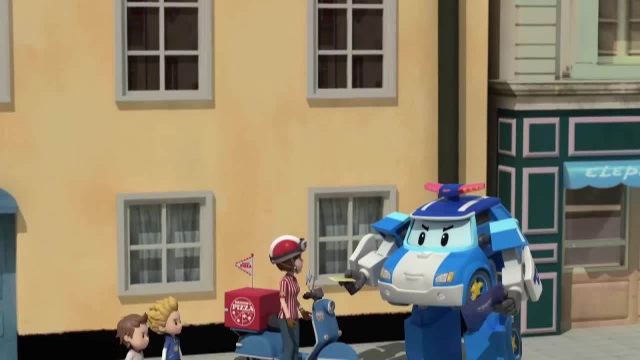 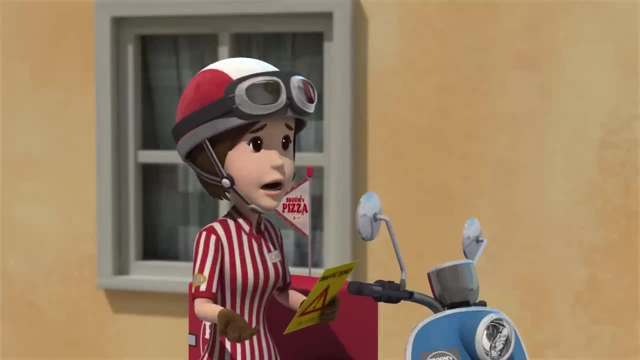 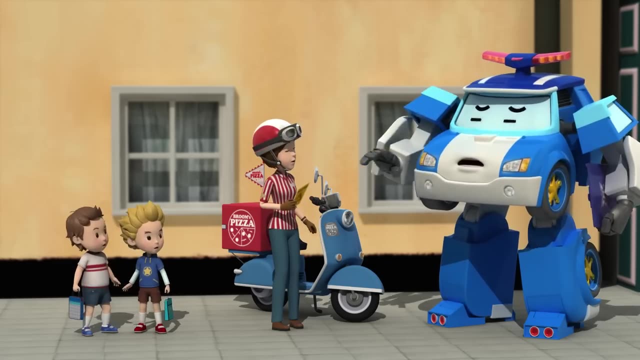 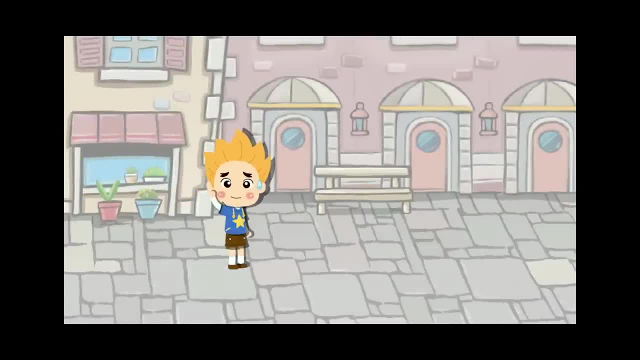 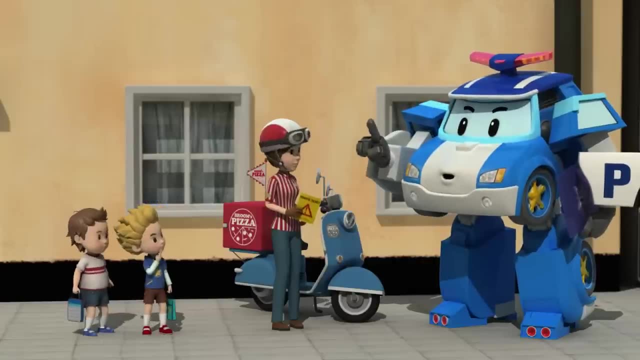 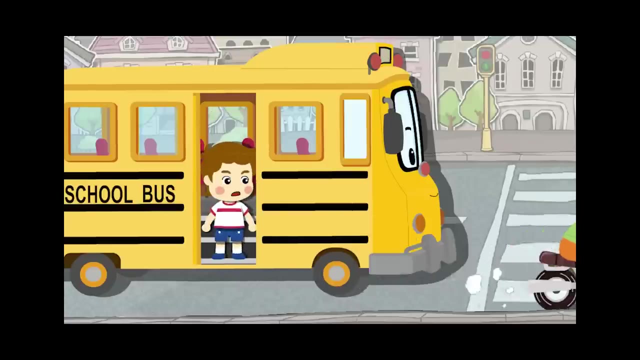 Instead stand in one spot or lean against the nearest wall. So, because motorcycles can move fast, even on narrow roads, you have to be cautiously aware when you're going down a side street, getting off a bus and even when you're walking on the sidewalk. 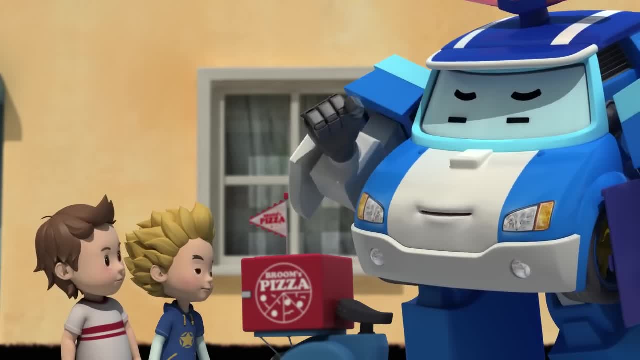 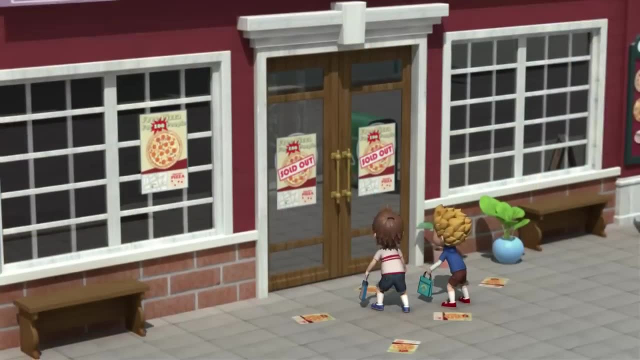 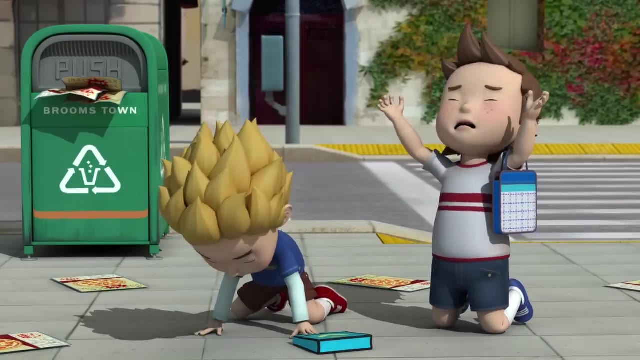 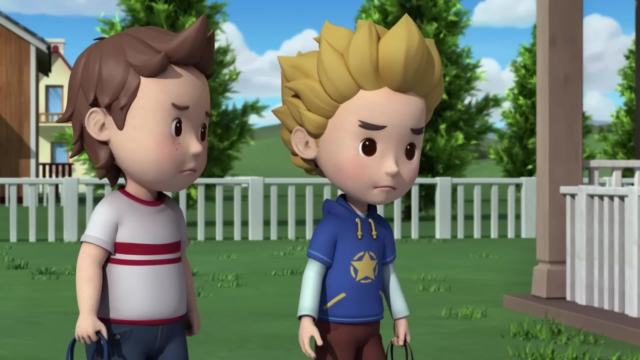 Do you see, kids? You could have an accident if you run around recklessly the way you were. We get it, Polly. No, We missed the pizza. What took you two so long? We're real sorry, Jenny. Yeah, we're sorry. Well, hurry up, Your pizza's getting cold. 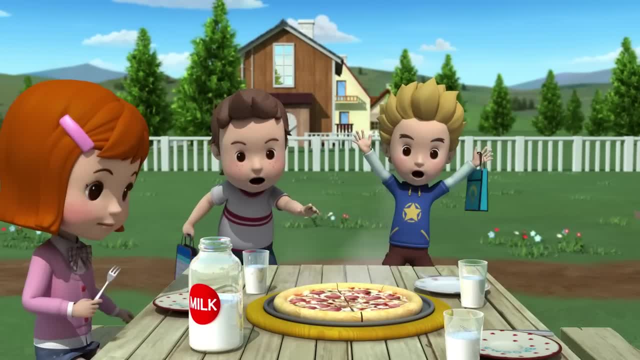 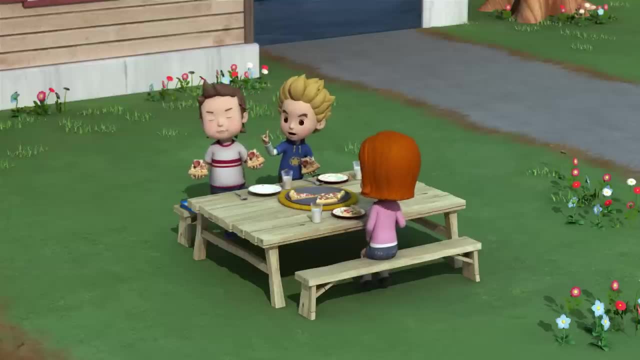 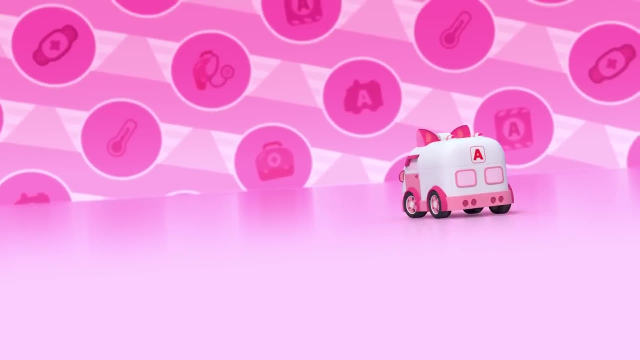 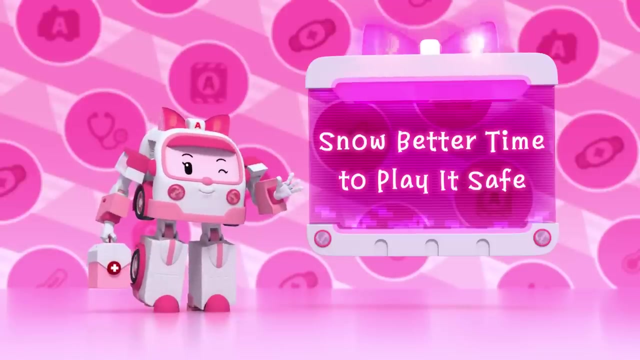 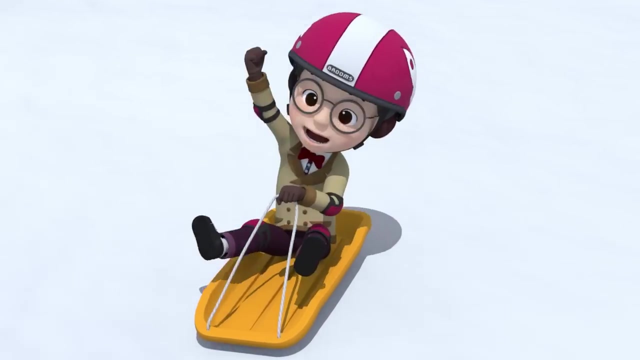 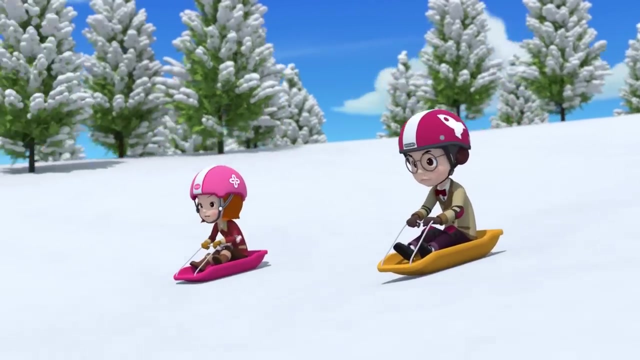 What, Wow, Pizza Delicious. Hey, come on One slice at a time. It's no better time to play it safe. Whee, Yahoo, This is great. Yeah, Heads up, Huh, Whoo, Hey, Don't you know that's dangerous. 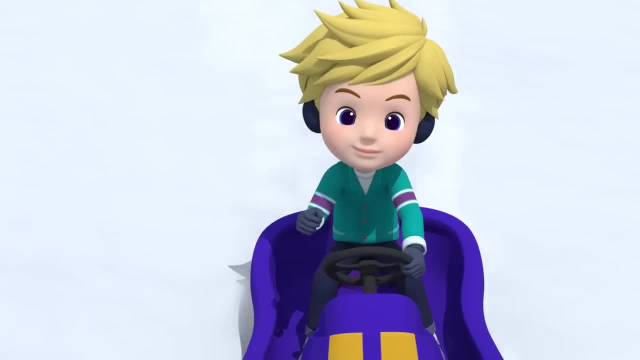 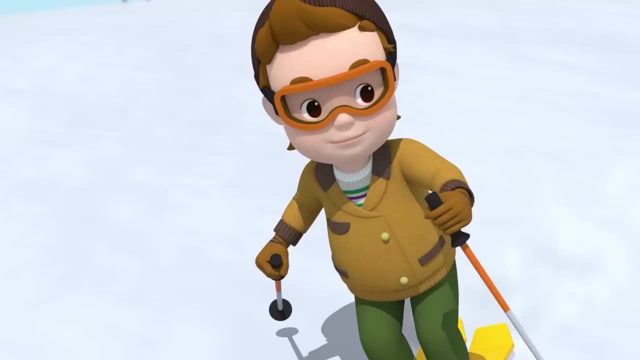 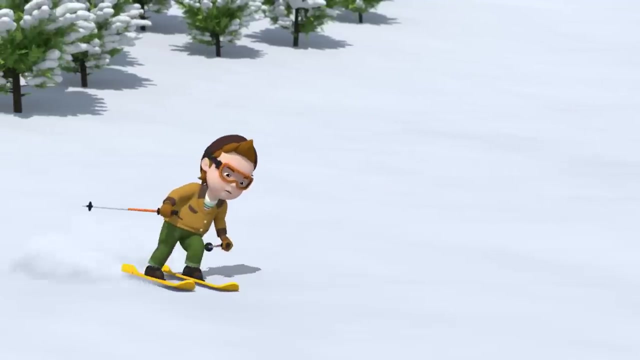 I'm the fastest person here. Oh, is that what you think, Don't? you see, Nobody can even match the speed I go. Huh, When you fall behind, don't get snow in your face. What? No, I'm not that fast. 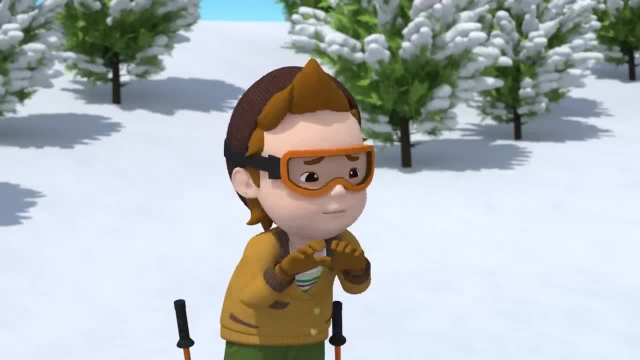 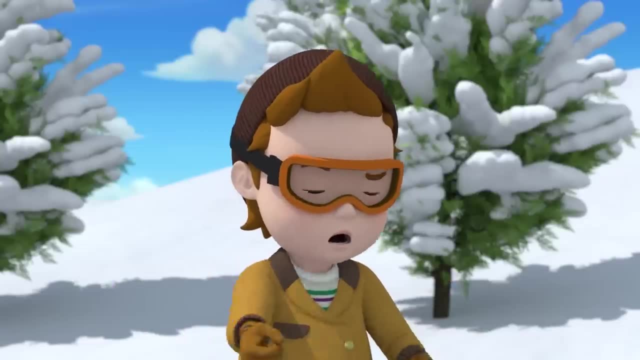 What took you so long? Someone's a real slowpoke, Slowpoke. I'm fast. You don't know what you're talking about And I don't think that you could ever beat me in a race. Hey, come on, I challenge you to a rematch. 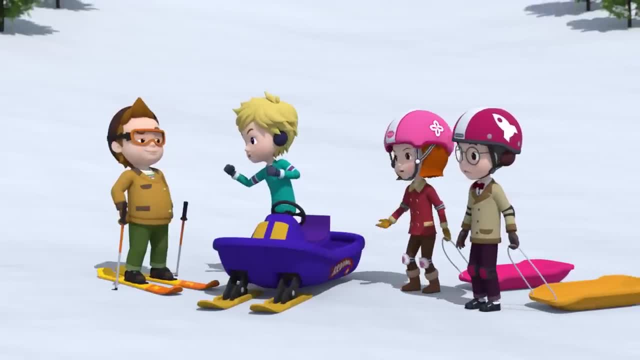 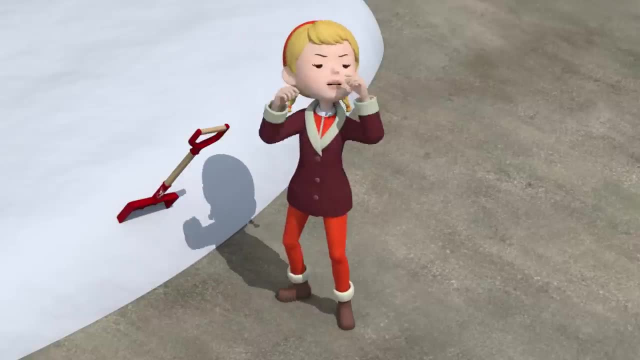 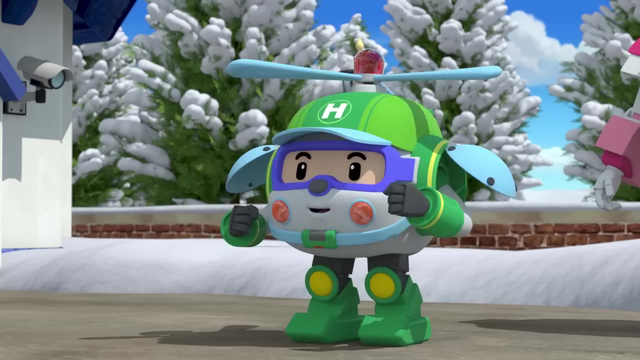 I look forward to winning again. Ugh, Would you guys stop this? Hey guys, Polly, Where have you been this whole time? There's so much work to do, Let's do it later. I want to sled. The kids are sledding on Apple Street and it looks so fun. 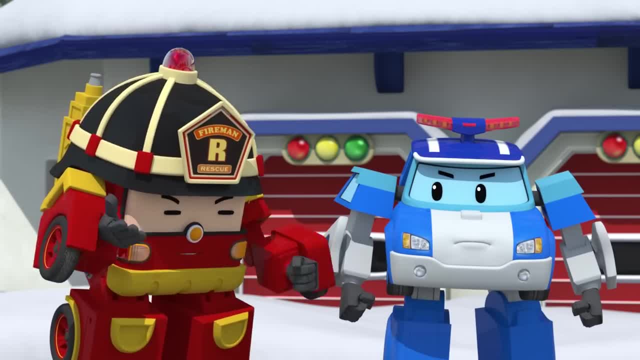 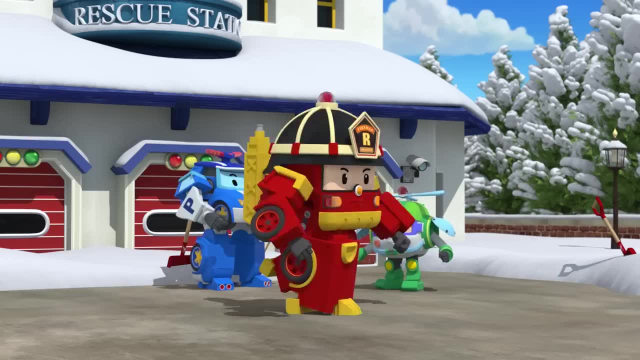 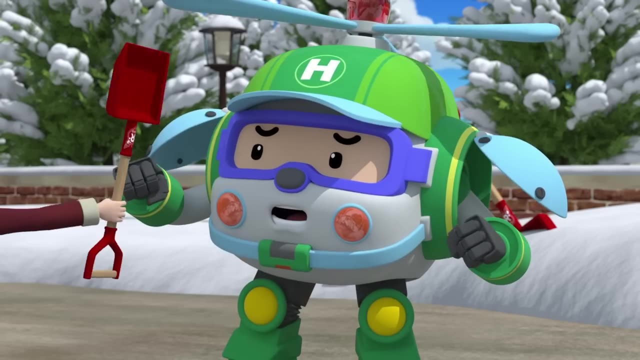 On Apple Street's hill. That hill could be dangerous. Are they alone? They need to be careful going down a hill that steep. I'll go check on them. I'll come as well. I want to come, Pelly. you're going to stay right here until your shuffling is done? 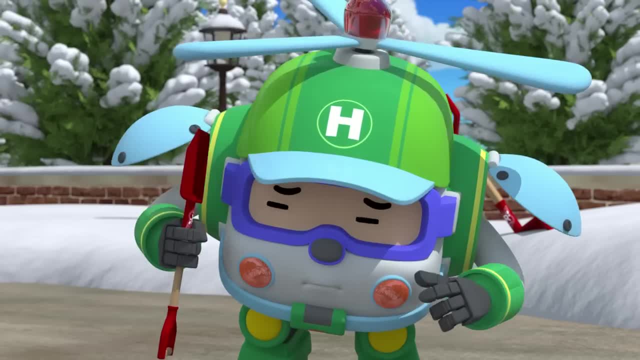 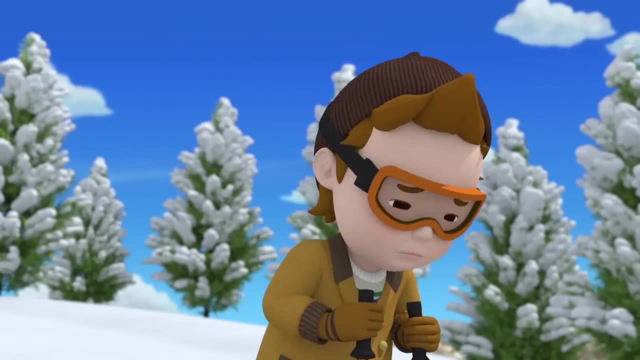 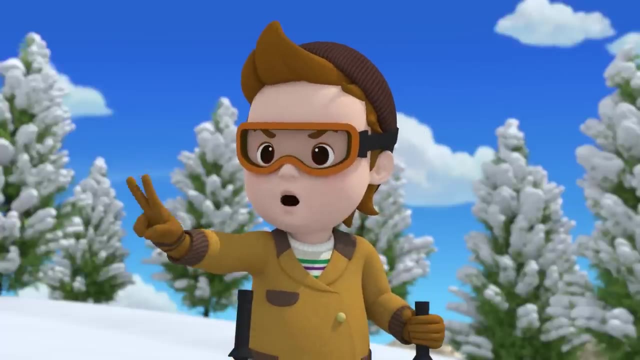 And all I wanted to do was sled. Don't you think this hill is a little tall? Oh my, Is someone chickening out now? I'm not scared. One, two, three and then we start. okay, Oh yeah. 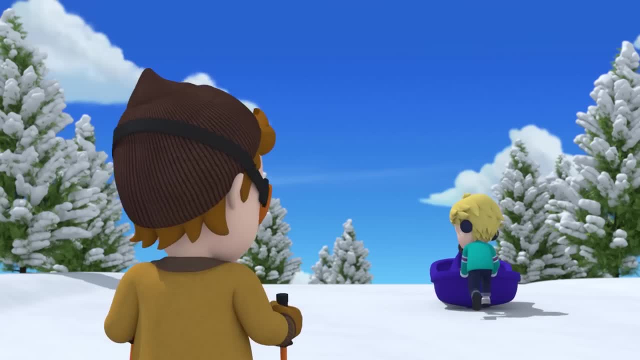 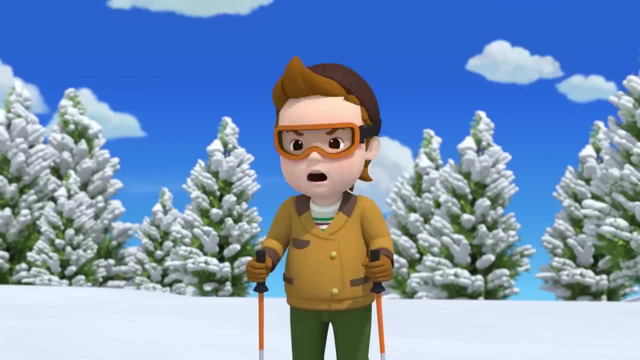 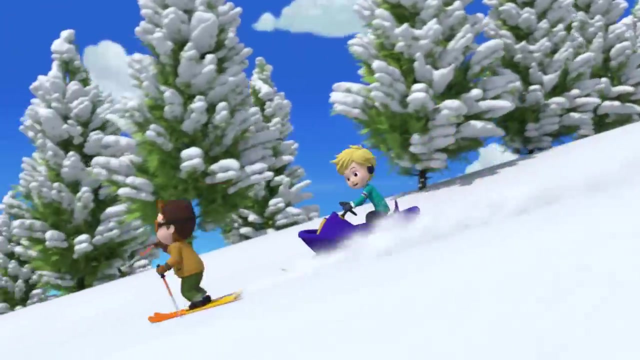 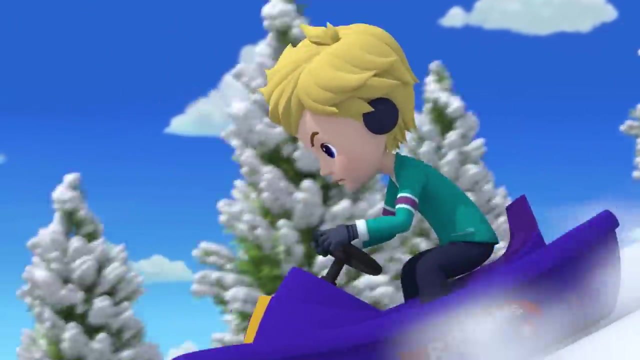 One, two, Smell you later. Hey, get back here. That's cheating. Couldn't hear you? You're too slow. Woo-hoo, Come on, I can't lose. Look who's still the fastest Me. Sorry, what was that? 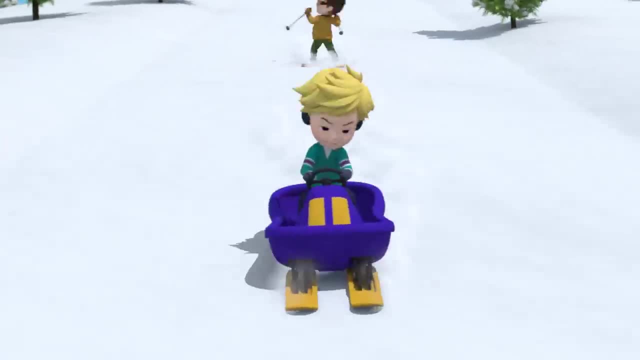 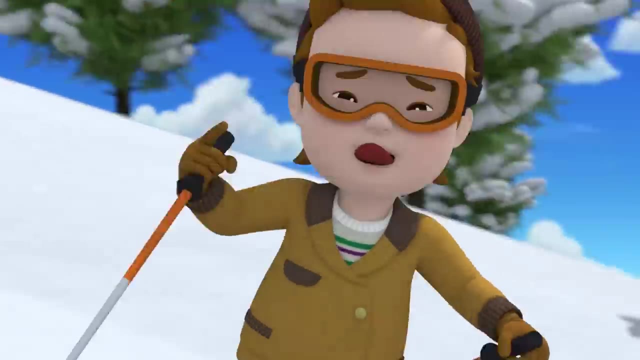 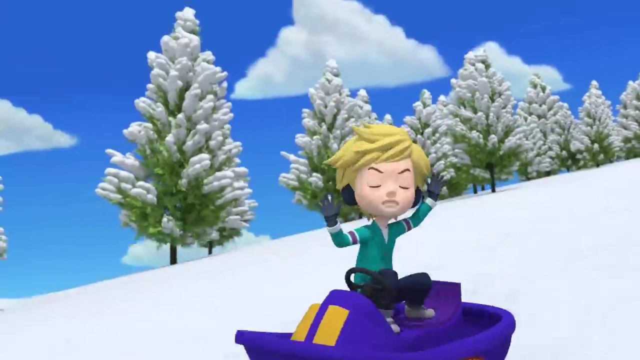 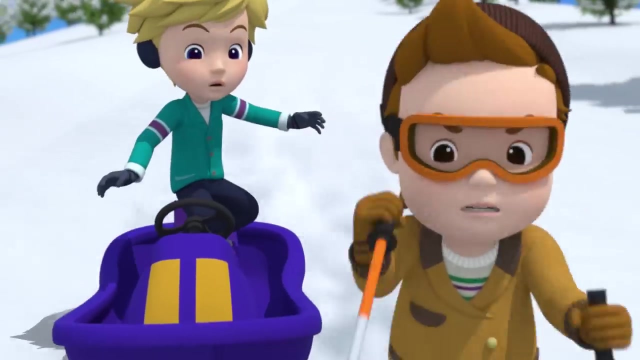 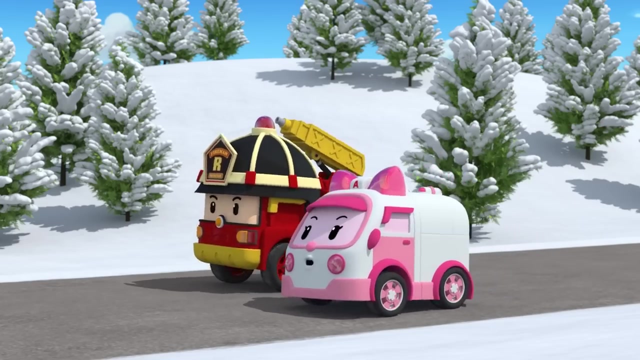 Ah, Sorry, Johnny, See you at the end. Huh Huh, Just admit I win. No way. Where did Helly say the kids were? Oh goodness, How fast are they going? Ten bucks says I win. 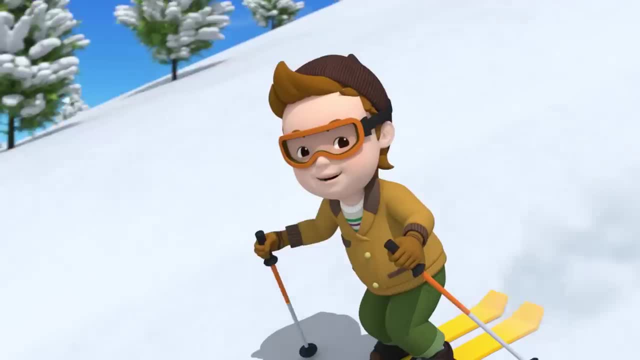 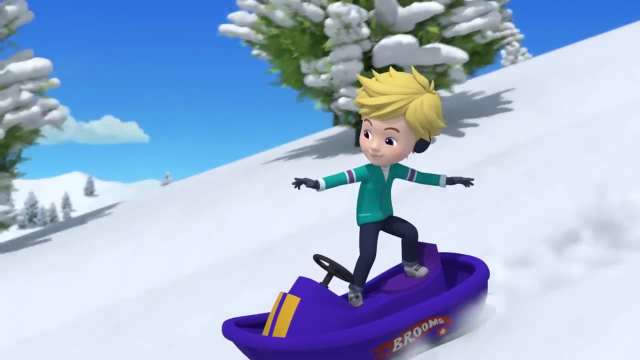 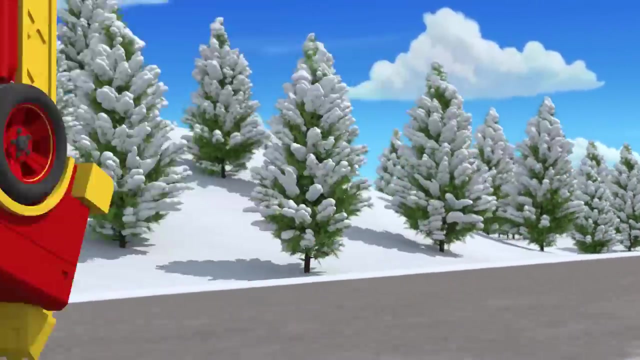 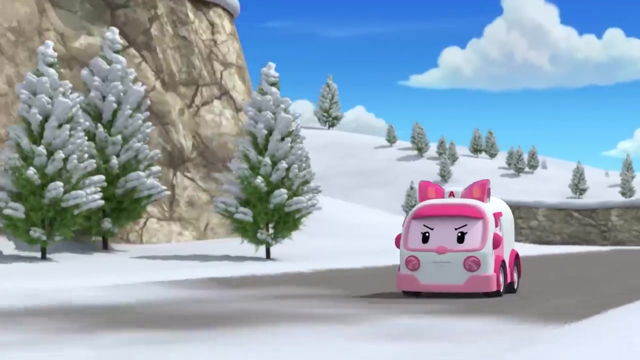 Huh, Oh, Johnny, watch out, I'm not falling for that. Victory is mine. Look out, Huh, Huh, Huh, Ah, Ah, Huh, Oh, Oh, Ah, Ah, Ah Ah. 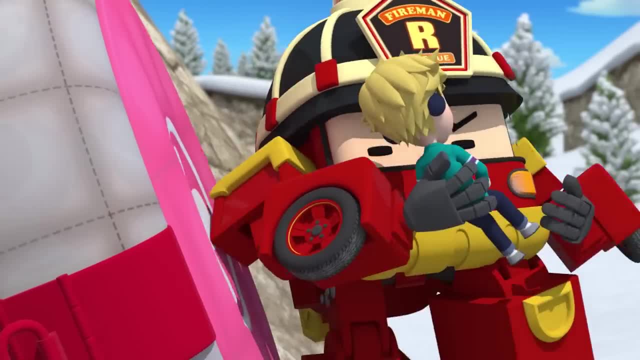 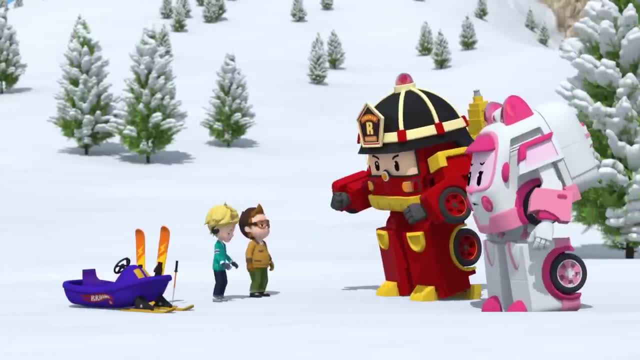 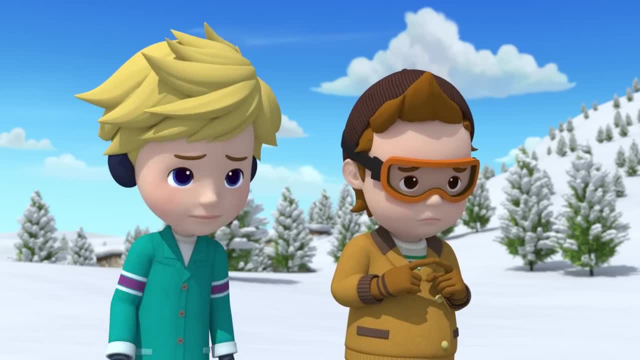 Thank you. Listen, don't you know how dangerous that was. You two could have gotten really badly hurt. We won't do it again. Roy, You guys, I know skiing and sledding can be a lot of fun in the winter.